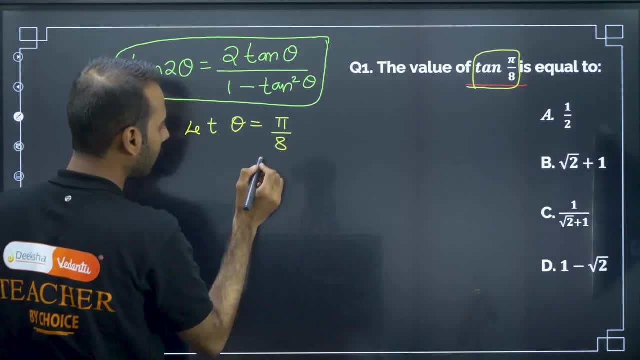 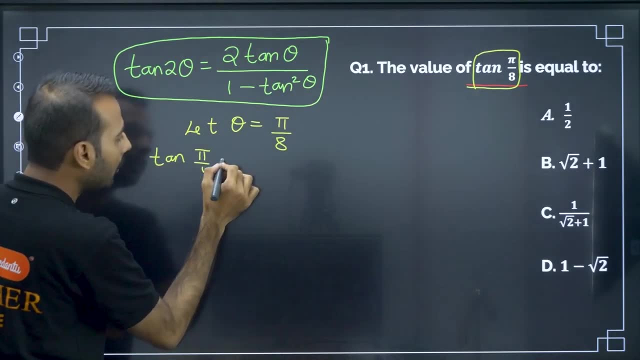 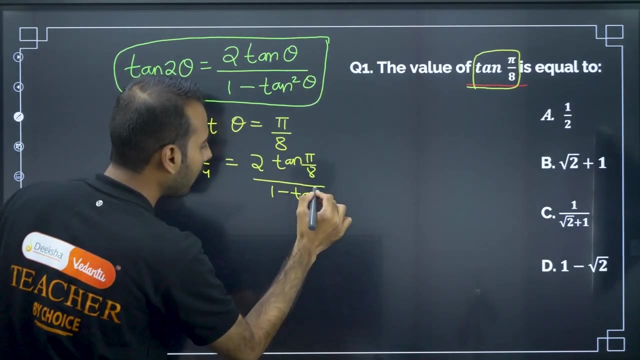 let theta is equal to let theta is equal to pi by 8.. So if I place this, theta is equal to pi by 8, this becomes tan pi by 4 is equal to 2 tan pi by 8, 2 tan pi by 8 by 1 minus tan square. 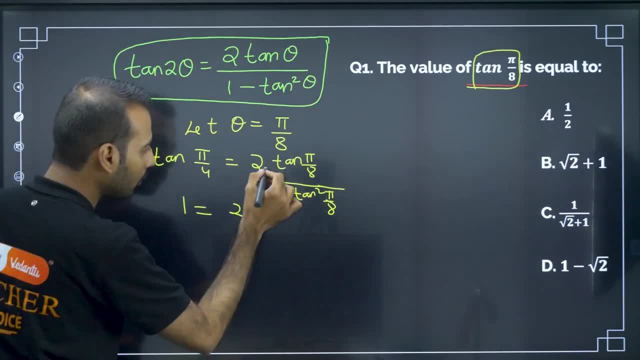 pi by 8.. Tan pi by 4 is 1, is equal to 2 tan pi by 8 by 1, minus tan square pi by 8.. 2 tan pi by 8,. let me name this as x For a moment. let me name this as. let me call this as. 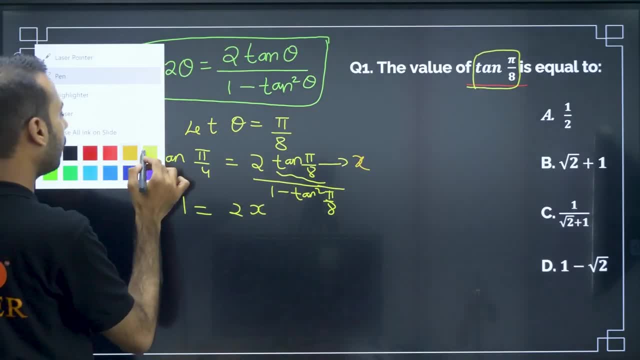 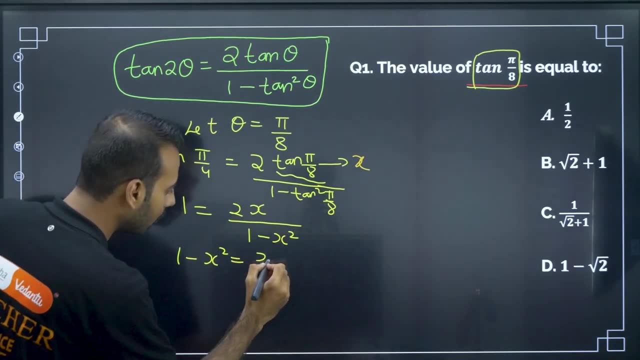 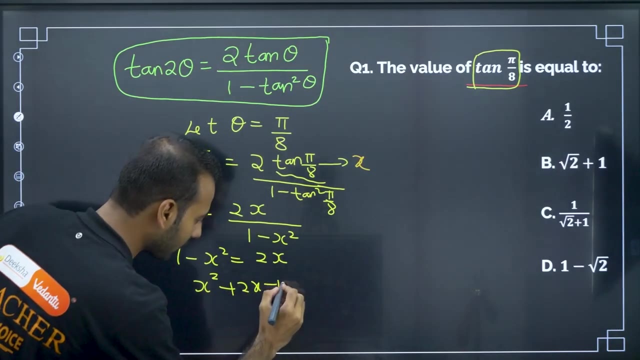 x. Let me call this as x. So this is 2x by 1 minus x square. So if I transpose this 1 minus x square is equal to 2x. If I transpose this x square, x square plus 2x minus 1 is equal to 0,. 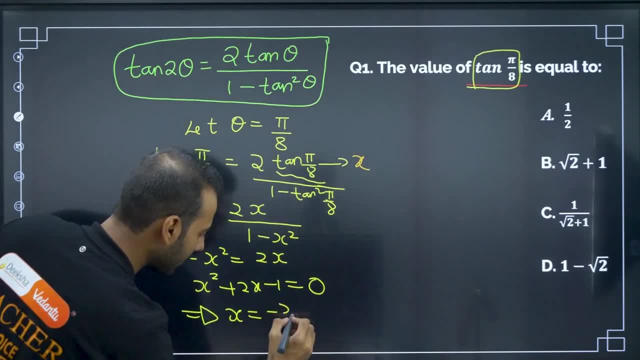 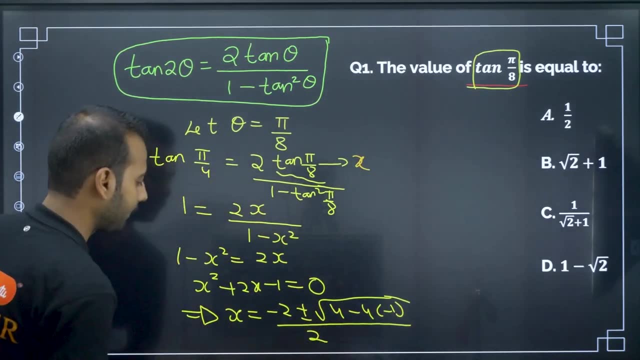 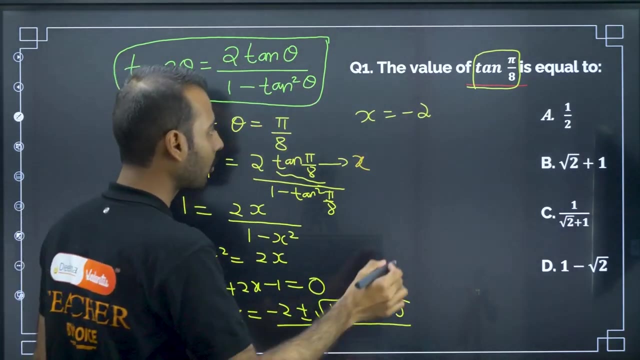 which implies x is equal to minus b, plus or minus minus. root of b, square minus 4ac by 2a. So from here we can say: x is equal to, x is equal to minus 2, minus 2, plus or minus plus, or. 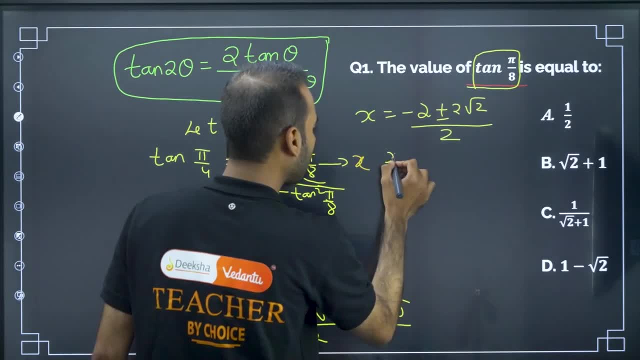 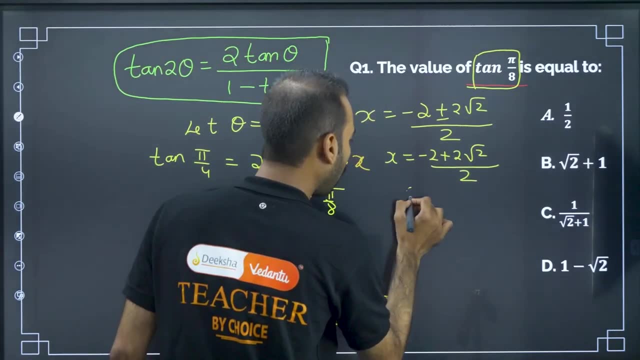 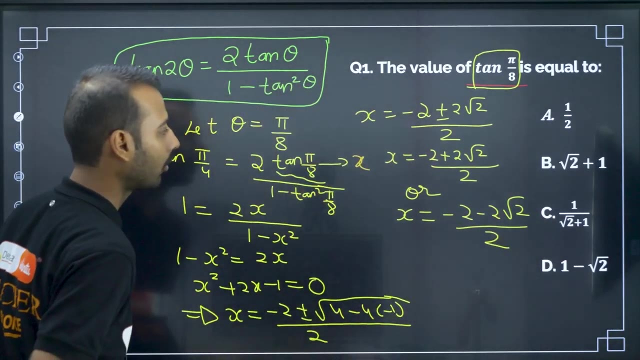 minus 2, root 2 by 2, which implies x is equal to minus 2 plus minus 2 plus 2. root 2 by 2, or x is equal to x is equal to minus 2 minus 2, root 2 by 2. there are two possibilities. this one I am discarding, because tan pi by 8 means this: 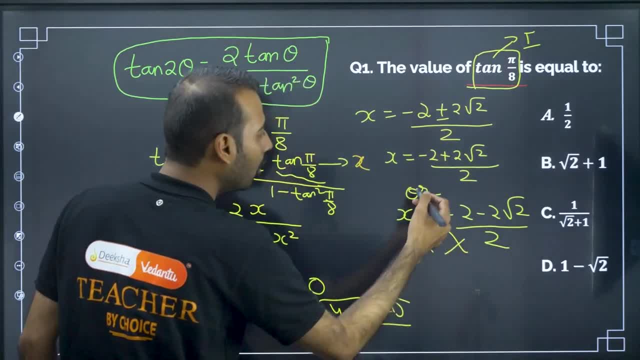 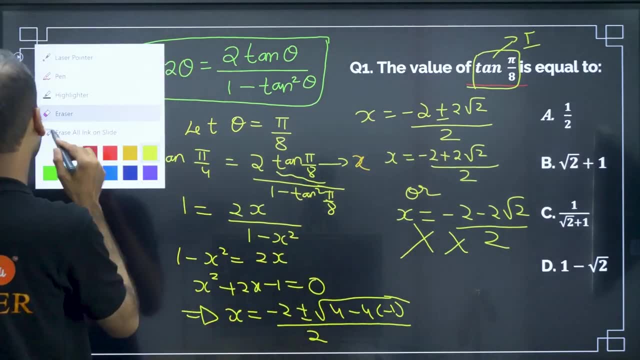 will lie in first quadrant. in first quadrant. here we are getting negative value, so this is not possible. next, moving on to next, we have to simplify this. x is equal to x is equal to this value. we have to simplify, to simplify this. let me erase few things. if you want to make an out of 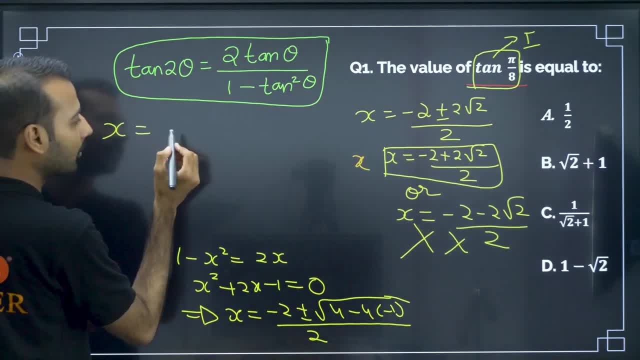 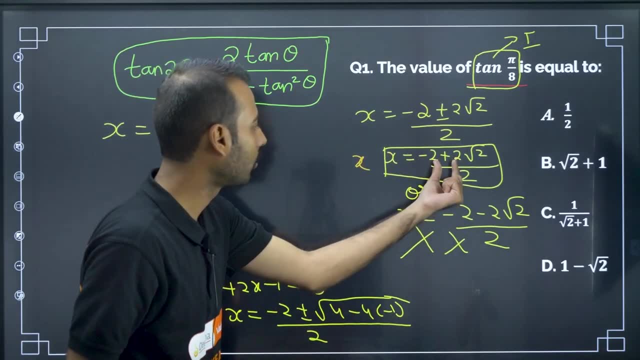 this. you make an out of this. x is equal to. x is equal to minus 1 minus 1 plus root 2. x is equal. if I simplify this, x is equal to minus 1 plus root 2. now x equal to. we were supposed to find. 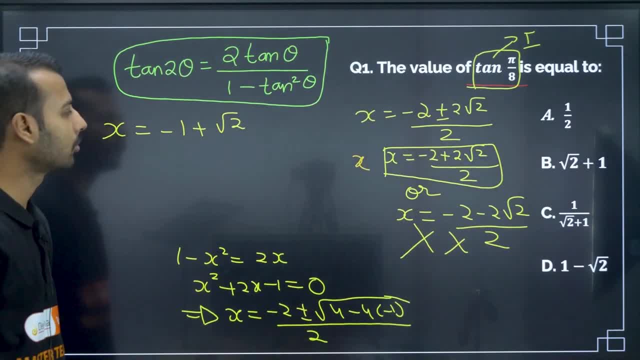 x. value x is equal to minus 1 minus 1 plus root 2. this is directly not available, so we have to do some alterations. root 2 minus 1: same thing I am writing. root 2 minus 1 is not there in option, so 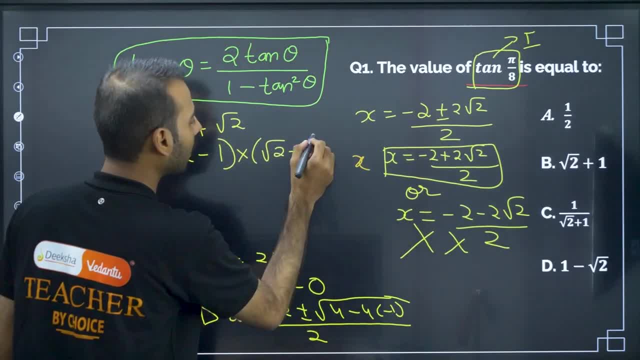 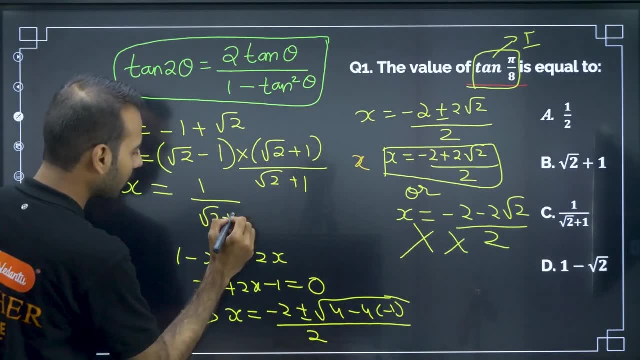 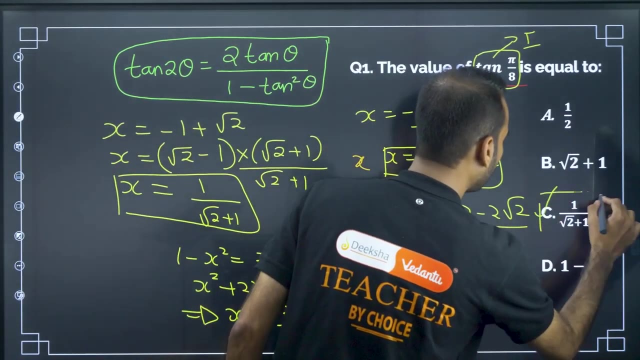 let me multiply and divide with its conjugate root 2 plus 1 by root 2 plus 1.. So, if I multiply, x is equal to 2 minus 1, is 1 by root 2 root 2 plus 1.. So x is equal to 1 by root 2 plus 1.. C is the answer. Moving on to next question, 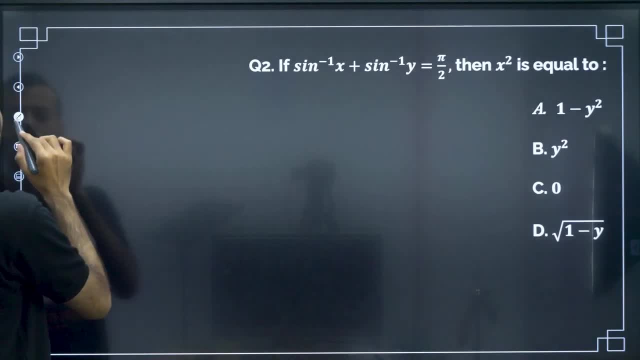 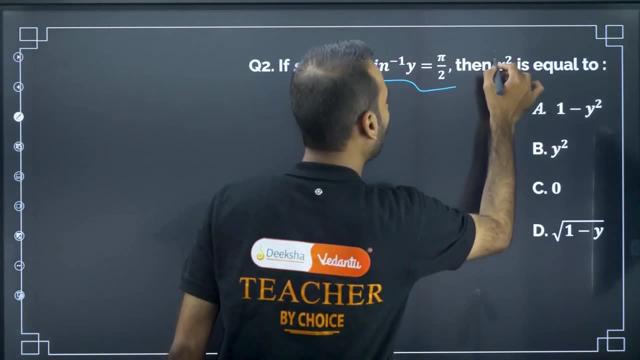 Sine inverse x, sine inverse x plus some information they have given. What is the information? Sine inverse x plus sine inverse y is equal to this. Then x square is equal to what x square is equal to. They are asking to find x value- Some information they have given. 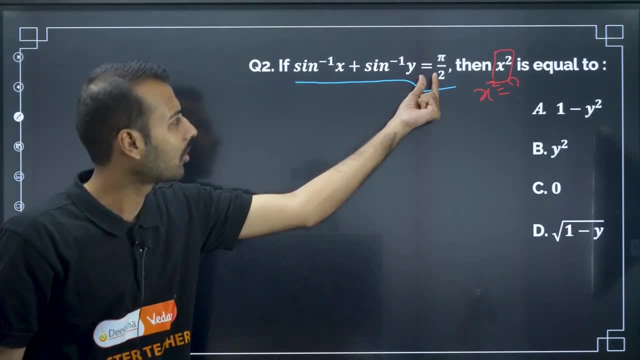 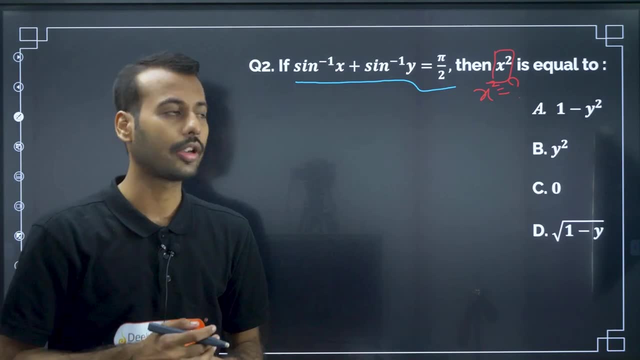 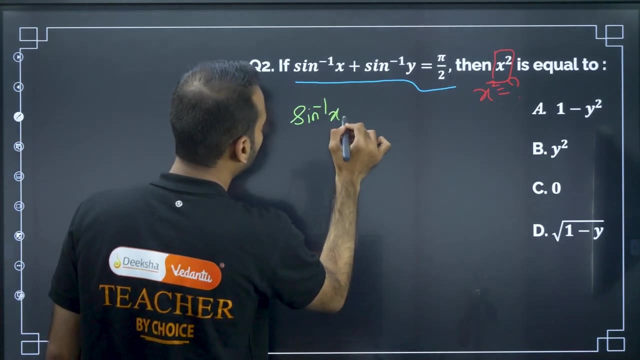 some information they have given: Sine inverse x plus sine inverse y is equal to pi by 2.. Now, in inverse trigonometry, some identities we are having. You should be able to recall some identities. What are those identities? One identity is sine inverse x plus cos inverse x. 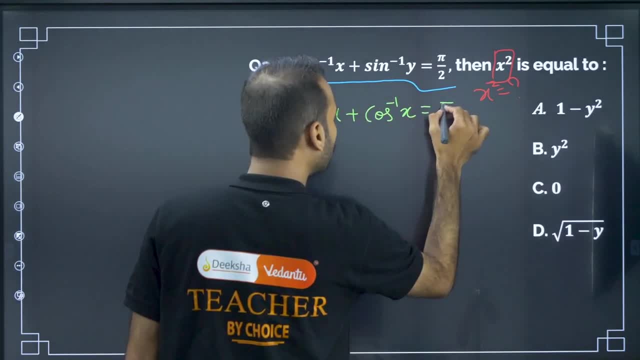 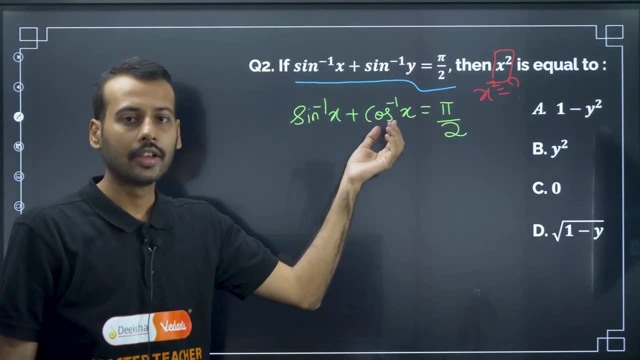 sine inverse x plus cos inverse x is equal to pi by 2. sin inverse x plus cos inverse x is equal to pi by 2.. Try to recall this identity, since I am writing with green pen means it is identity. it is a part of synopsis that you should be able to. 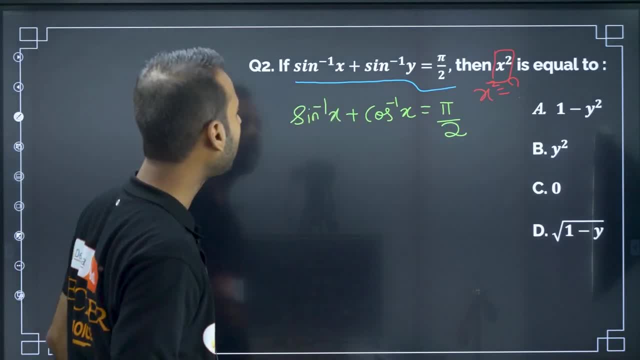 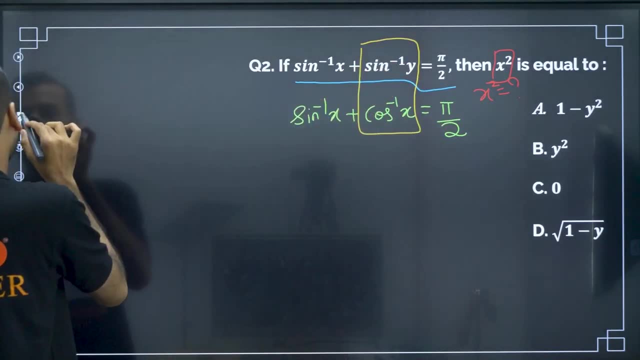 recall Now sin inverse x. the moment. you see, here everything is same. in place of sin inverse y we are having cos inverse x. that means that means sin inverse y. that means sin inverse y is equal to cos inverse x. from here I am coming to conclusion. Now, if I want to write sin inverse y in terms of: 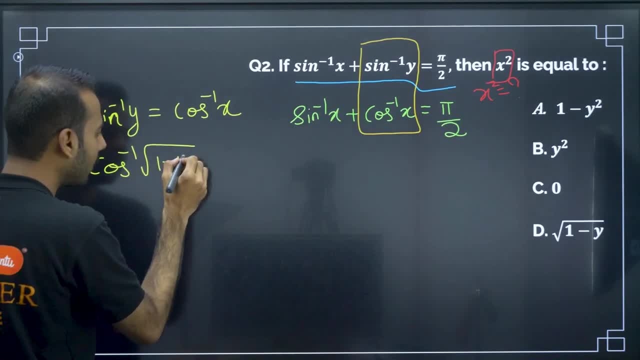 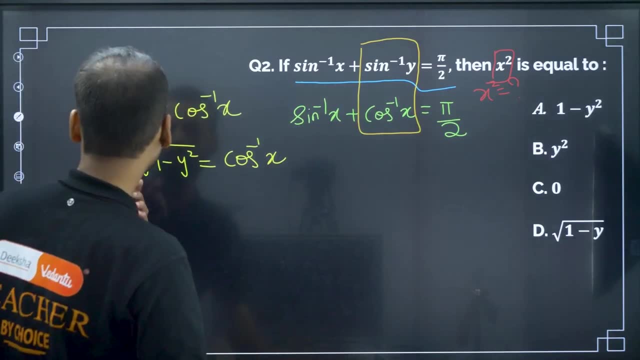 cos inverse. I will write this as: cos inverse root of 1 minus y square is equal to cos inverse x is equal to cos inverse x. So sin inverse y is equal to cos inverse y is equal to sin inverse y is equal to sin inverse y is equal to sin inverse y is. 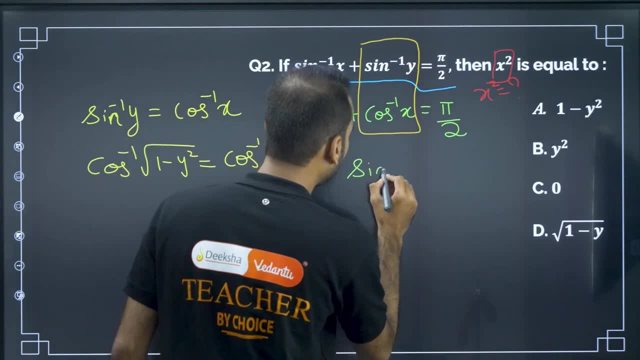 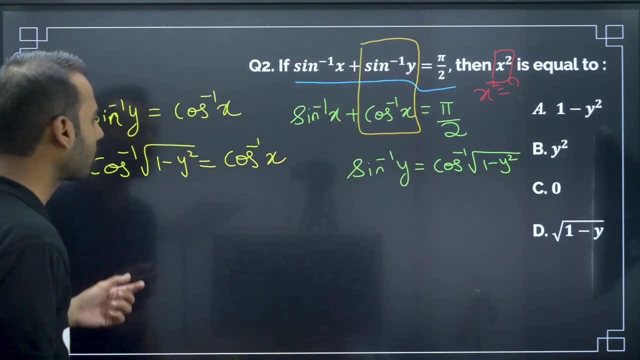 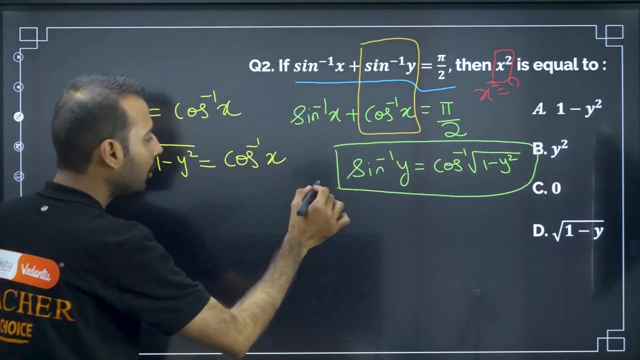 inverse. Now again one more synopsis point. you take: sin inverse y is equal to cos inverse root of 1 minus y square. Again one more synopsis point. you take, sin inverse y is equal to. so I am replacing cos inverse. This is one synopsis point you should be able to recall. 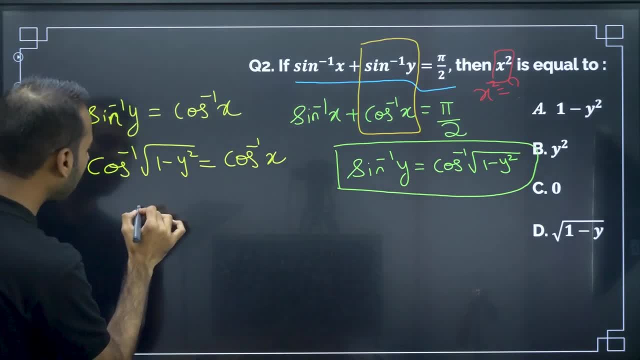 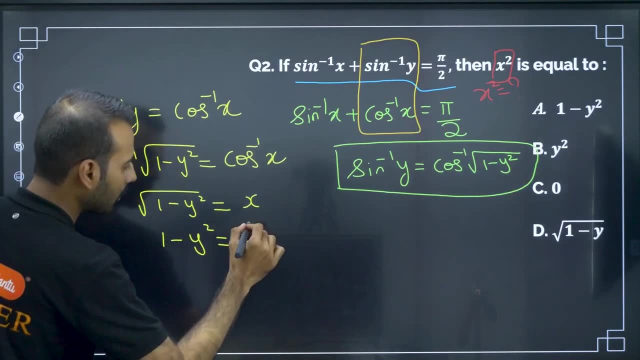 this at this point. Next now sin inverse. from here I can come to a conclusion: 1 minus y square is equal to x. If I square on both sides, 1 minus y square is equal to x square. 1 minus y square is equal to x square. So x square is equal to 1 minus y square. So 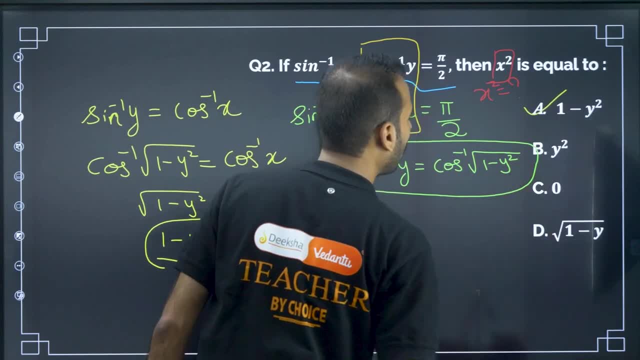 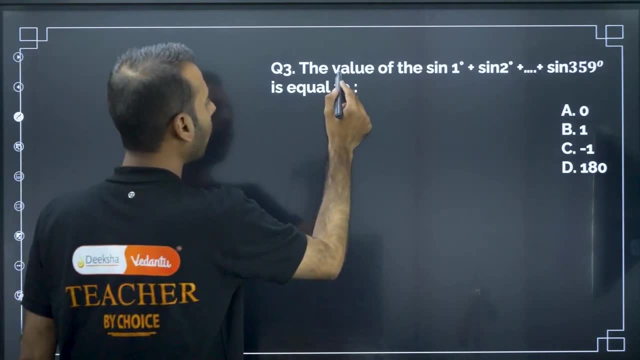 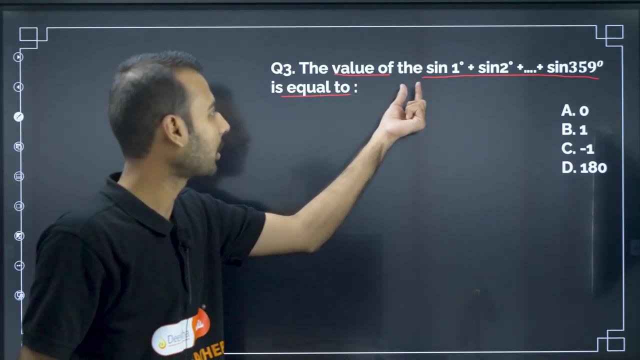 x square is equal to. they are asking to find value of x square. So a 1 minus y square is the answer for this. Moving on to next, the value of what is the question? The value of sin 1. all this is equal to what they are asking to find its value, The value of sin. 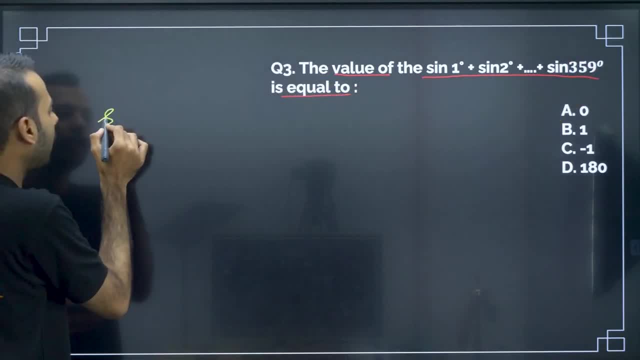 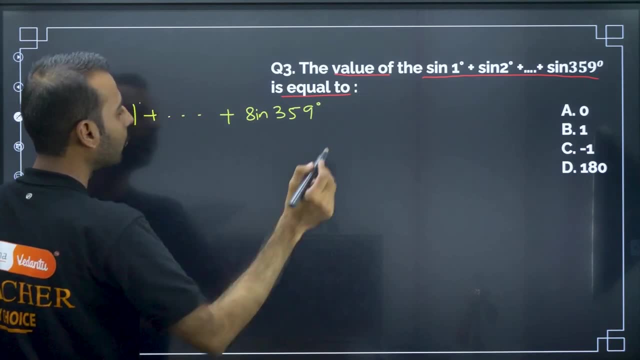 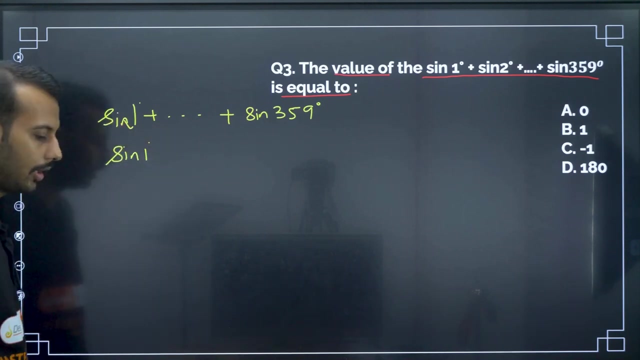 1 degree, sin 2 degree. up to this. Now let me copy and paste that sin 1 degree, plus so on, up to sin of 359 degrees, up to sin 359.. So sin 1 in place of sin 1. I am writing sin 1 degrees only in place of sin 1. let. 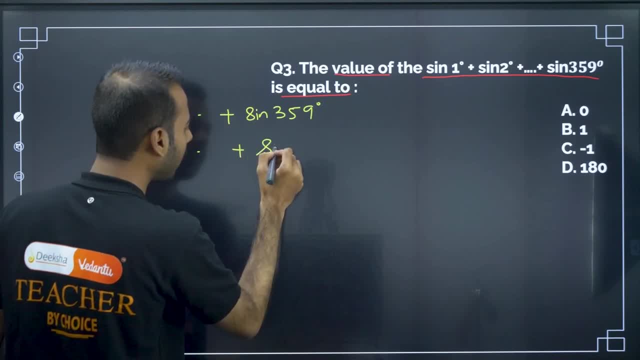 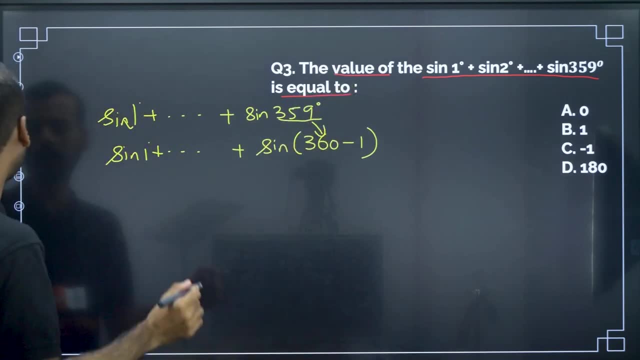 me write sin 1, so on remaining things. in place of sin 359, let me write 360 minus 1. 360 minus 1, 359 is same thing as 360 minus 1.. Now one synopsis point. you should be knowing what is. 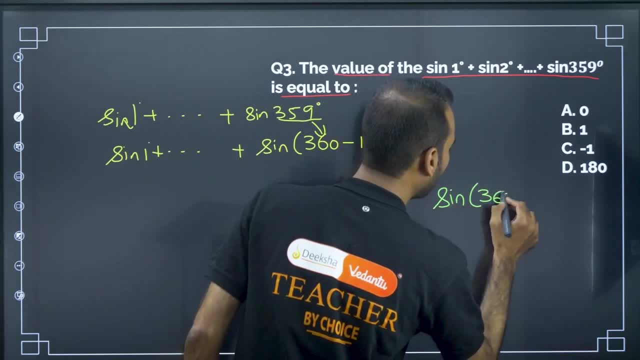 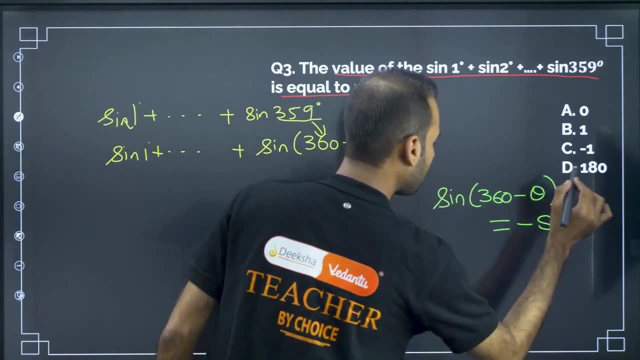 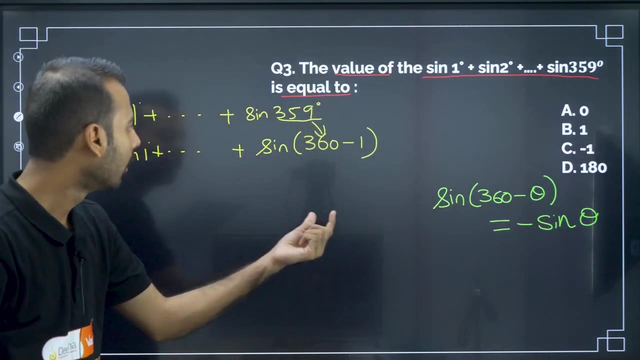 that synopsis point, sin of 360 minus theta is equal to minus sin theta, minus sin theta minus sin theta. So sin now for this. if if you are able to recall this synopsis point, it is a good thing. this synopsis point we have to use here: sin 1 plus blah, blah, blah, blah, minus, if you see. 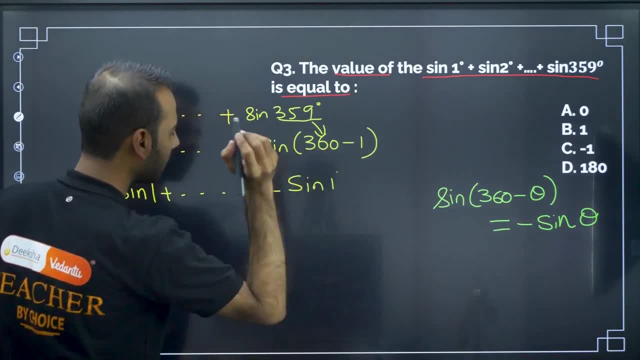 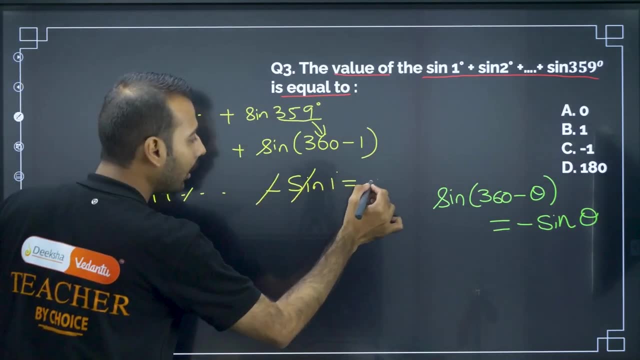 here. So sin 360 minus minus sin minus sin, So sin 1 plus all this, this plus 1 negative 1. in the same way, remaining terms also get cancelled and at last we are left with 0.. So the value of this? 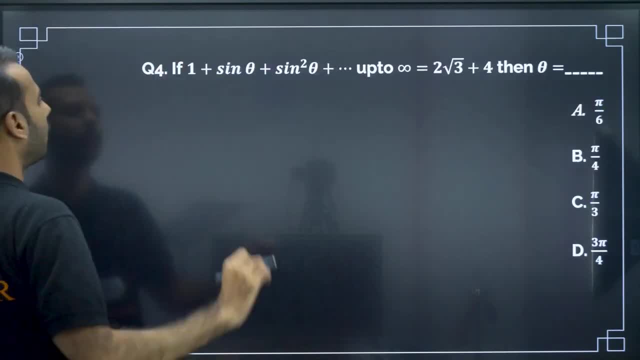 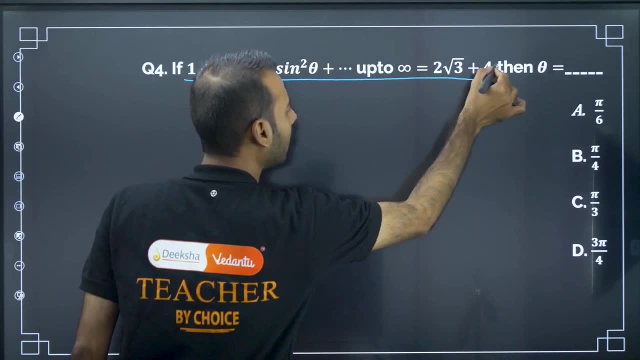 is equal to 0. the value of this is equal to 0.. Moving on to next question, some value. they have given one equation: 1 plus sin theta, up to infinity. then what are they asking? they are asking to find the value of theta. theta is equal to. 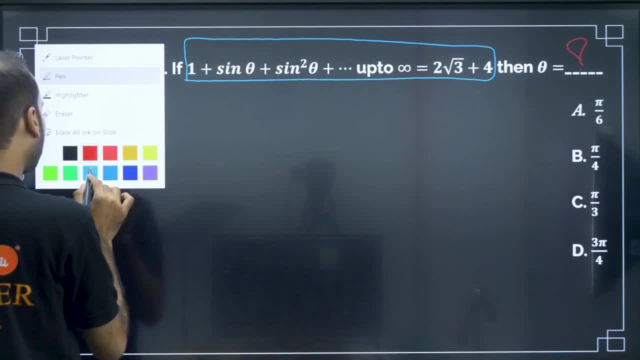 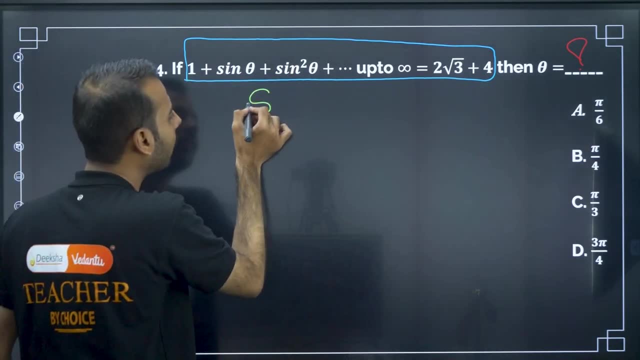 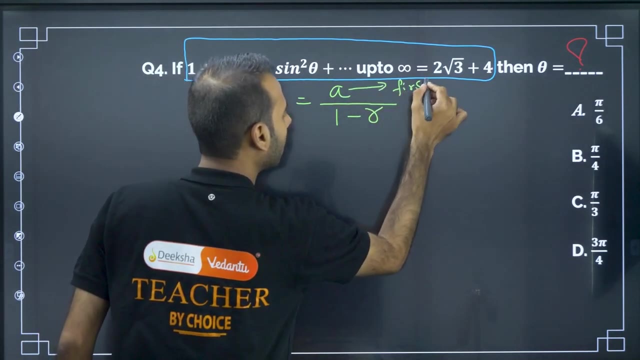 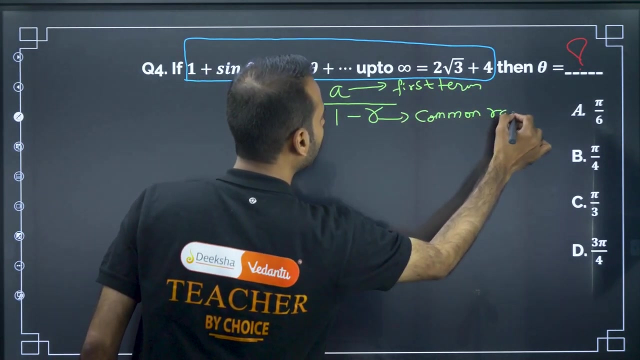 what? what now the movement? you see this one synopsis. if you see this, this is geometric progression, from geometric progression. sum of infinite terms of S. infinity is equal to a by 1 minus R. there, A is first term, first term, R is R is common ratio, common ratio. 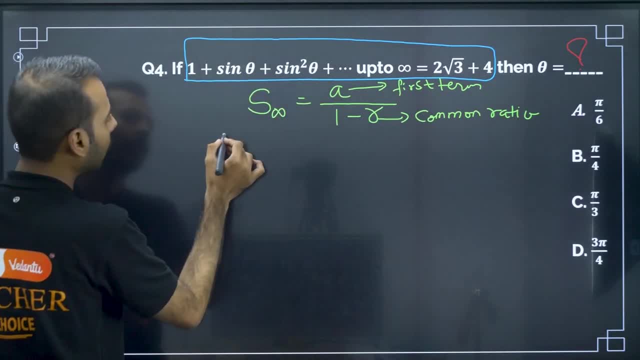 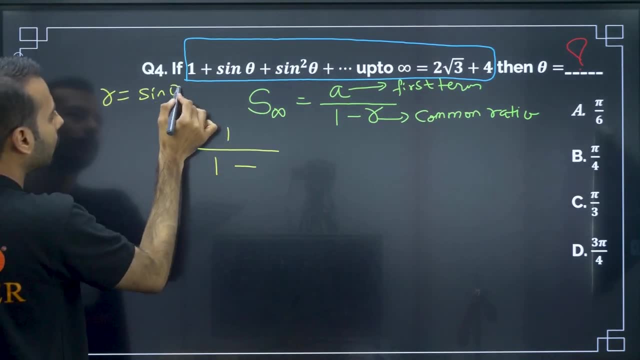 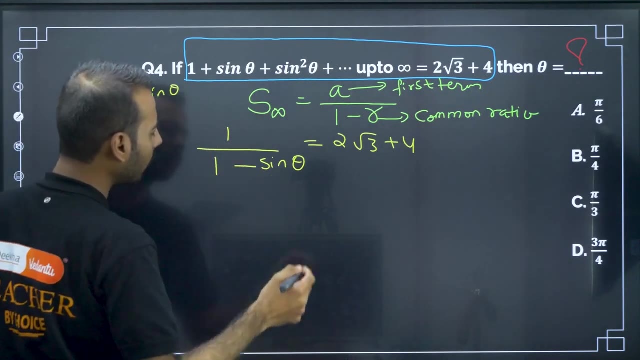 R is common ratio. Now S is first term, First term. first term term is 1 by 1 minus r is here, if you observe, r is equal to sin theta by 1.. So 1 minus sin theta is equal to 2 root, 3 plus 4.. So 1 by 1 minus sin theta is equal to 2 root. 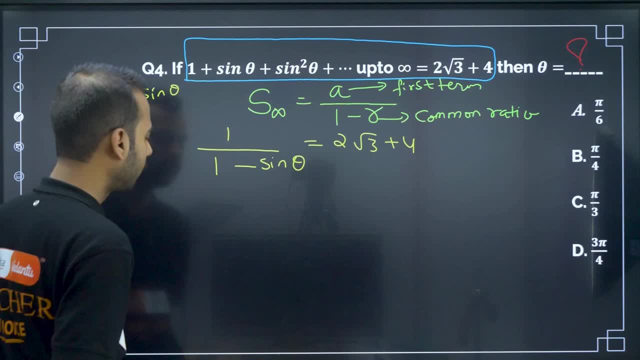 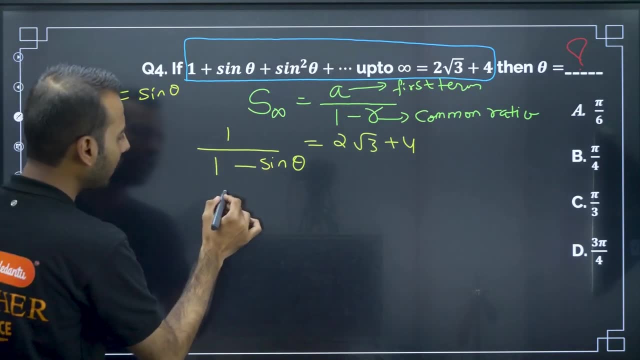 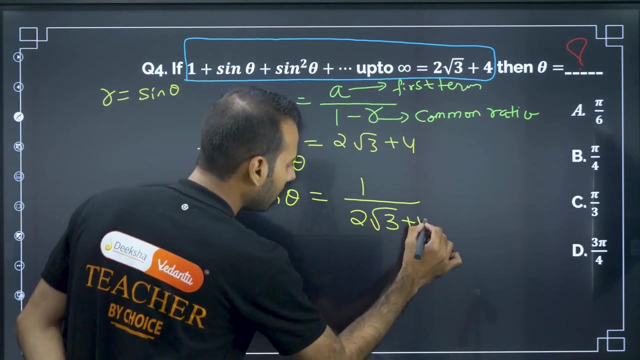 3 plus 4 is equal to 2 root 3 plus 4.. So for this, if I take reciprocal, what are they asking? they are asking to find theta from here. we have to find theta. So I will apply reciprocal: 1 minus sin. theta is equal to 1 by 2 root 3, 2 root 3 plus 4. 1 by 2 root 3. 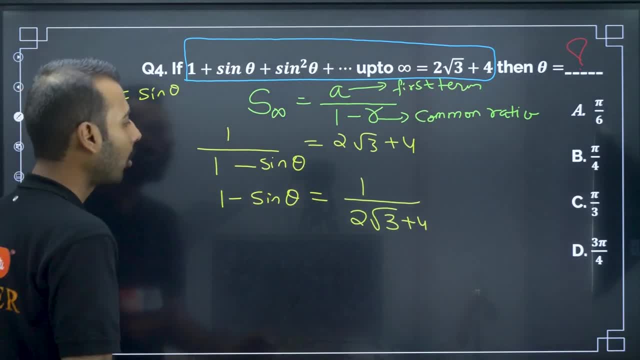 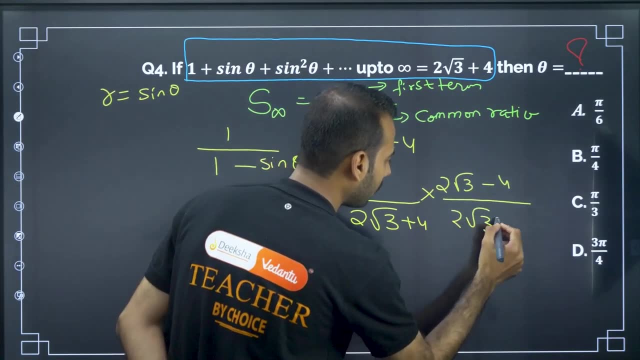 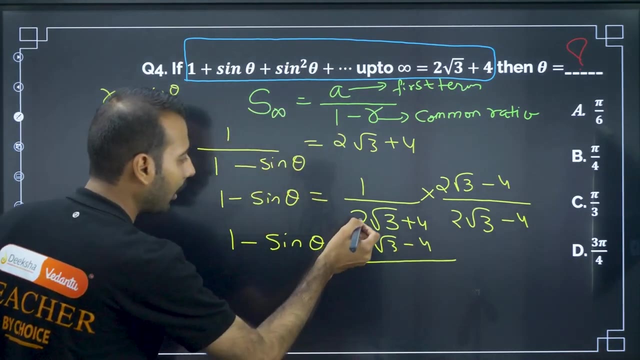 plus 4.. I am applying reciprocal function on both sides Also here. if I multiply 2 root 3, 2 root 3 minus 4 by 2 root 3 minus 4, 1 minus sin, theta is equal to 2 root 3 minus 4 divided by. if you multiply this: a plus b, a minus b, a square. 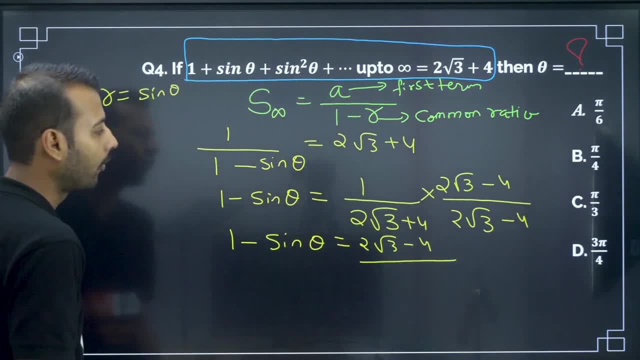 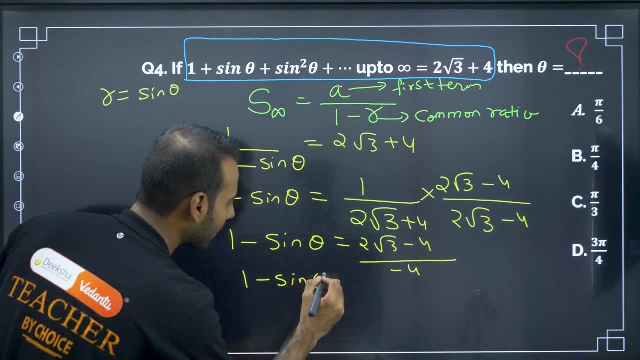 minus b square. a square minus b square means 4. 3 is a 12 minus 16. 12 minus 16 is minus 4. so 1 minus sin theta, 1 minus sin theta is equal to minus root, 3 by 2 minus minus plus 1. so if I cancel this plus, 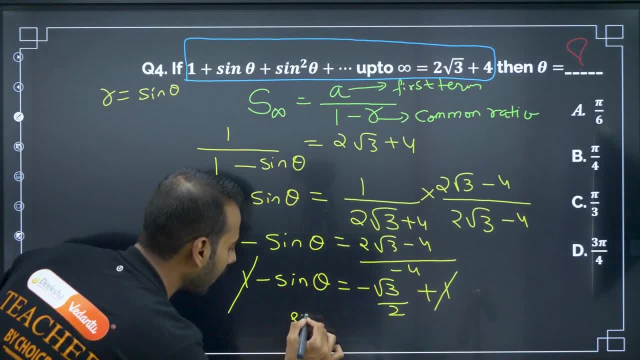 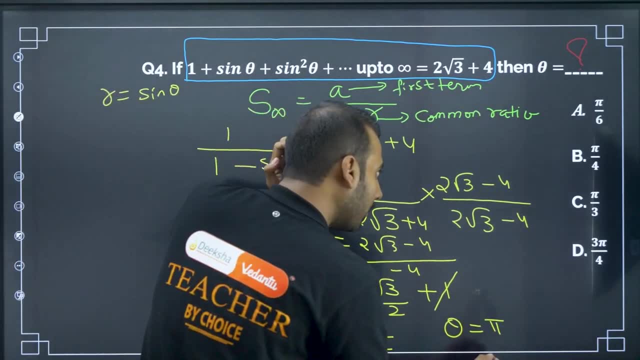 1 and plus 1 from here. here I am left with sin. theta is equal to root 3 by 2, which implies theta is equal to pi by. theta is equal to pi by 3. theta is equal to pi by 3. theta is equal to pi by 3 is. 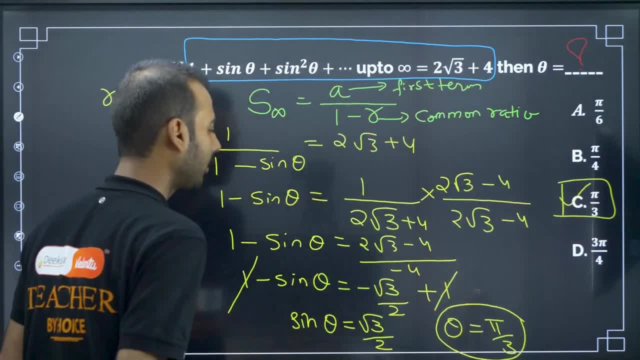 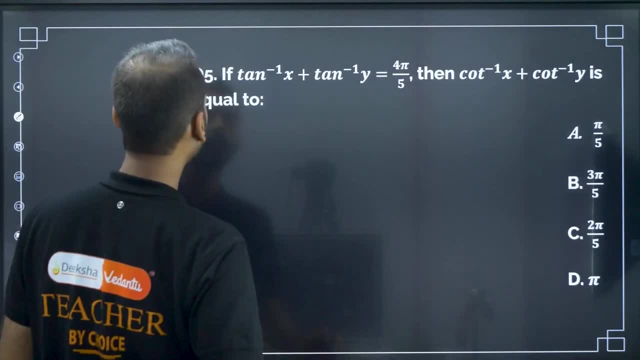 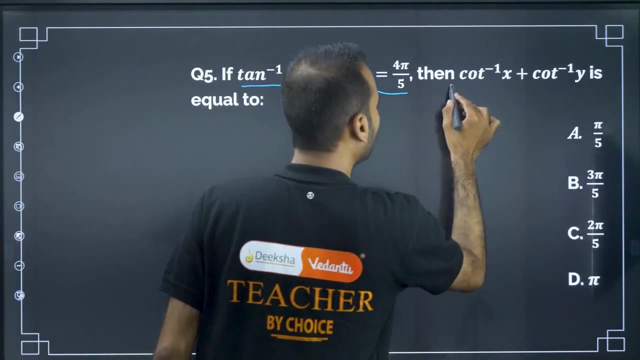 there, any such option like theta is equal to pi by 3. yes, c, theta is equal to pi by 3, is the answer for this. Moving on to next question. so in this question, some data they have given: if tan inverse x plus tan inverse y is equal to this, and they are asking, they are asking to find this, what is? 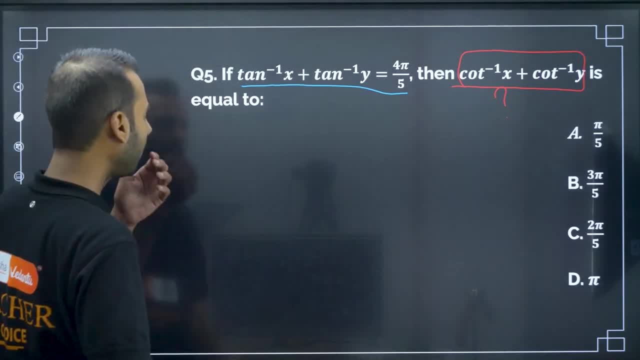 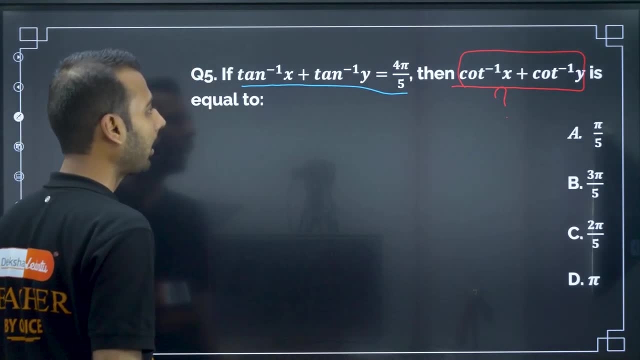 value of this. So this: if tan inverse x plus tan inverse y is 4 pi by 5 tan inverse x plus tan inverse now one i. they are asking they have given tan inverse x and they are asking cot inverse x. so there is a. 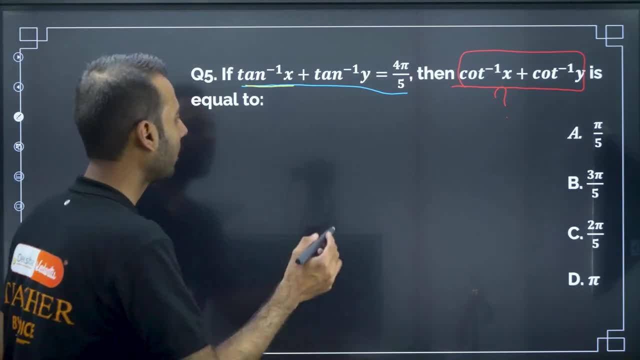 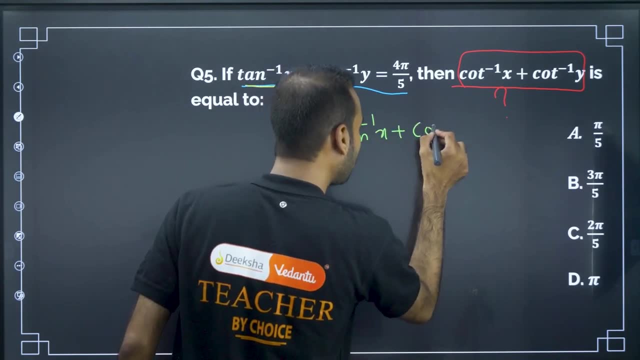 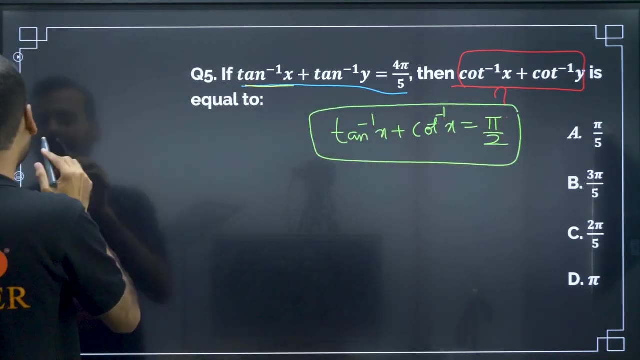 relation. there is one identity between tan inverse and cot inverse x. what is that identity? try to recall- i am writing this as synopsis point: tan inverse x. tan inverse x plus cot inverse x. cot inverse x is pi by 2. this is one identity in inverse trigonometry. now in place of tan inverse. 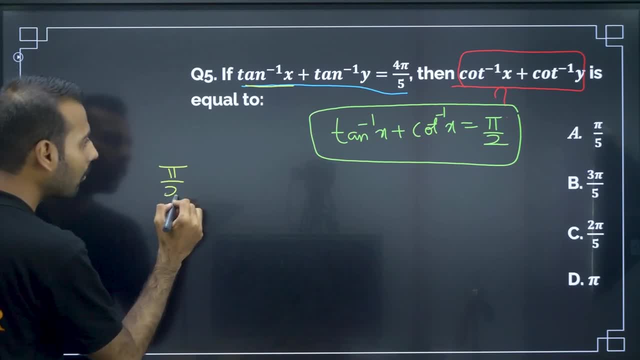 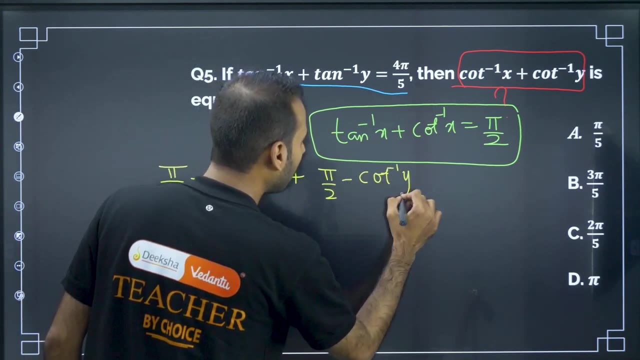 x in place of tan inverse x. i will write pi by 2 minus cot inverse x. pi by 2 in place of tan inverse x. i am doing this substitution. next, in place of tan inverse y, in place of tan inverse y, i will write pi by 2 minus cot inverse y, cot inverse y. its value is given as 4, pi by 5 its. 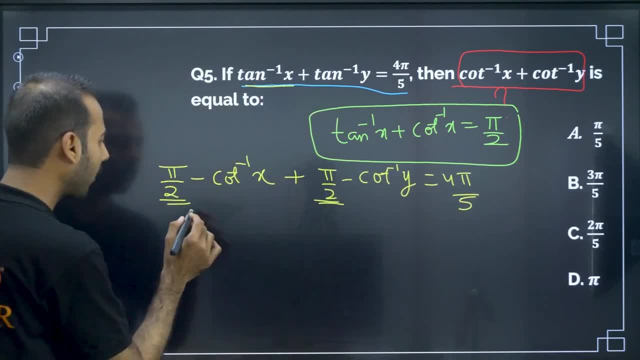 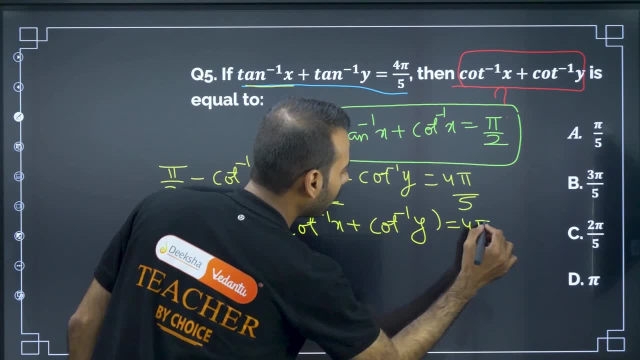 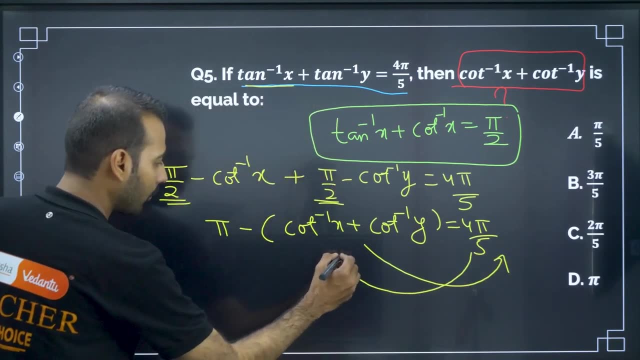 cot inverse y is equal to 4 pi by 5. 4 pi by 5, pi minus 4 pi by 5. if I transpose this to that side and if I transpose 4 pi by 5 here, I will get pi minus 4. pi by 5 is equal to. 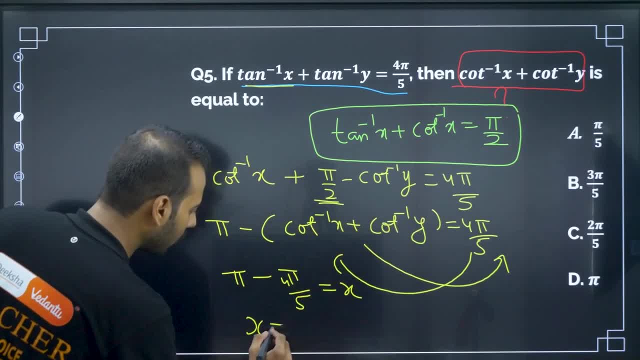 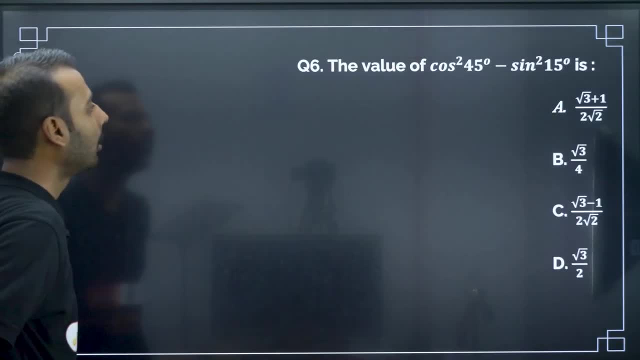 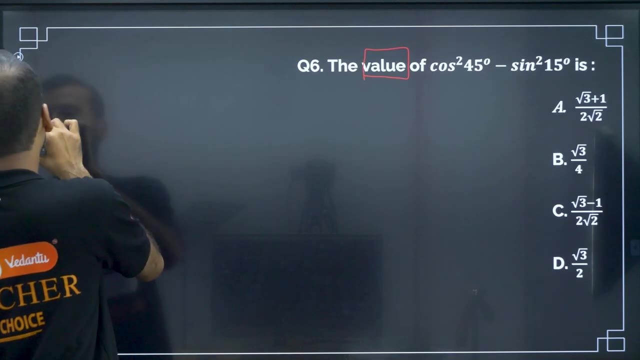 whatever this, I will name this as x. so x is equal to pi by 5. x is equal to pi by 5. so answer is pi by 5.. Moving on to next question, the value of the value of. they are asking to find the value of value of one trigonometric equation. they 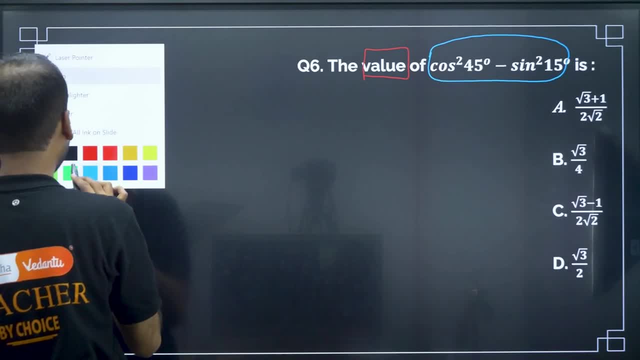 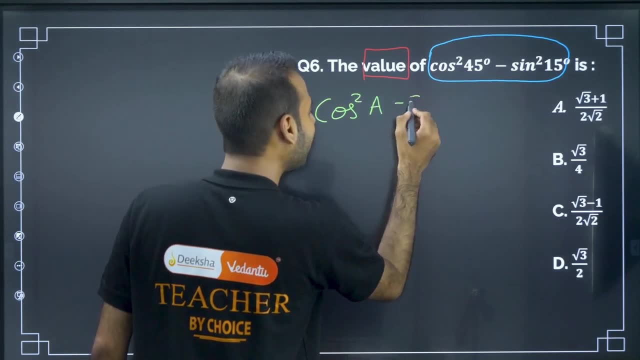 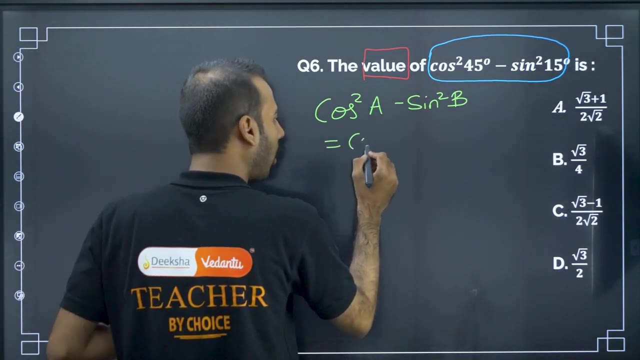 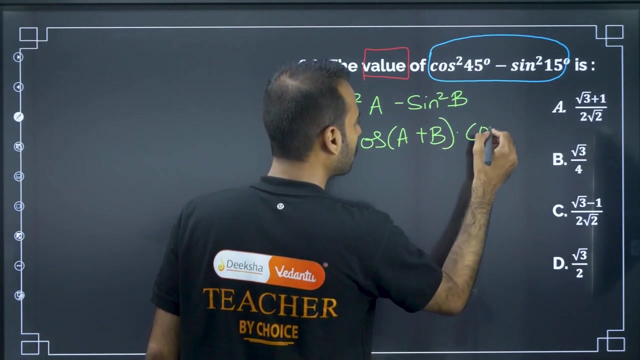 are given. there are. ask now, the moment you see cos square a minus sin square b, there is one standard identity for this: Cos square a minus sin, square b minus sin square b is equal to equal to cos of, is equal to cos of a plus b, a plus b into cos of a minus b, This identity. 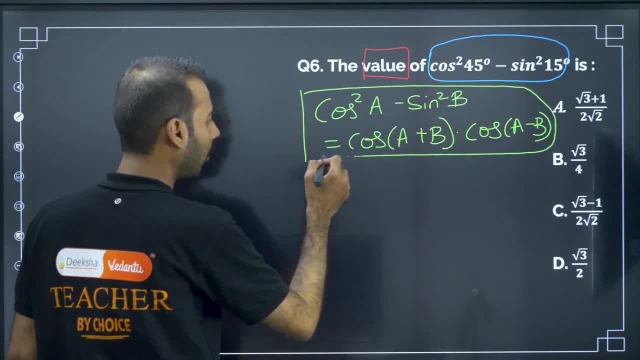 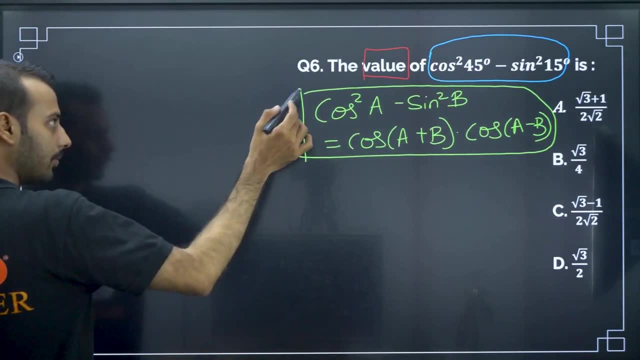 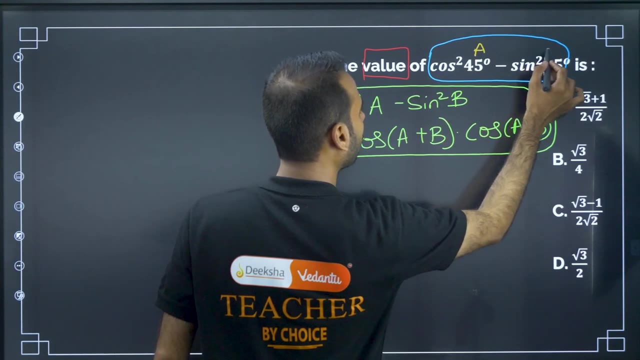 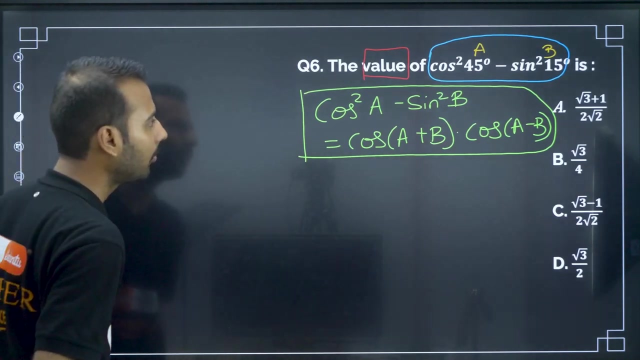 is their standard. you call this as formula or this. Now I am using this to solve this problem. So, in place of a, in place of, in place of a, we are having 45, in place of b, we are having 15.. So, cos of a plus b, cos of a plus b means cos of 45 plus 15, cos of. 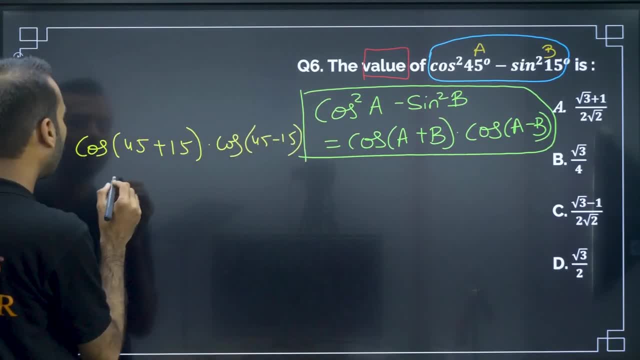 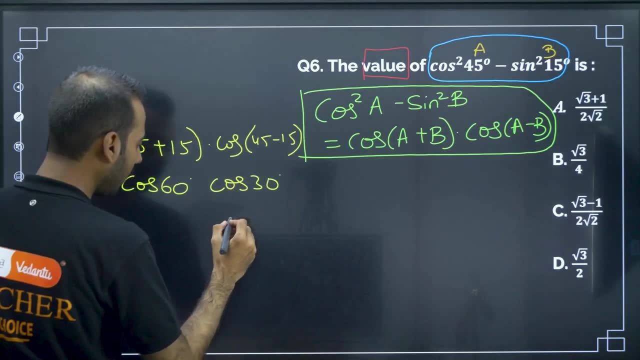 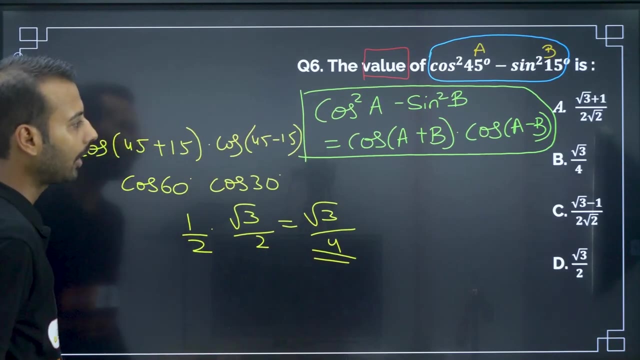 a minus b, 45 minus 15, cos 60, dot cos 30.. Cos 60 is cos 30, is root 3 by 2. cos 60 is 1 by 2.. So this is root 3 by 4.. So is there any such option like root 3 by 4.. So this is: 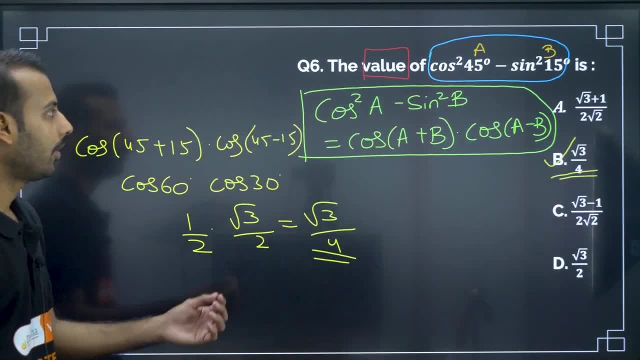 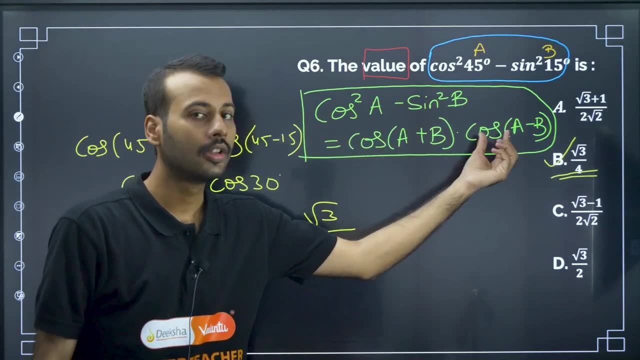 root 3 by 4. yes, b is the answer for this. See here: very easy question, less time consuming. only thing that you are supposed to know in this question is cos square a minus sin square b. if you know this in exam, no need to write this also. just you just have to calculate. 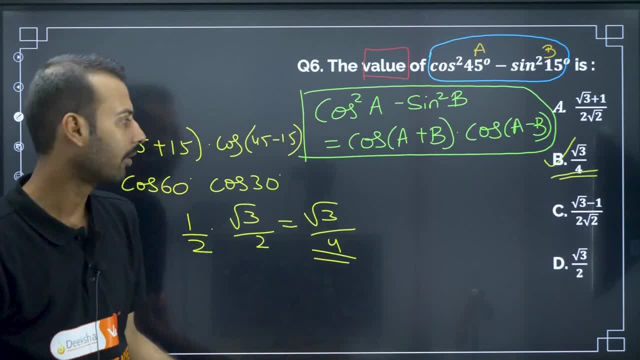 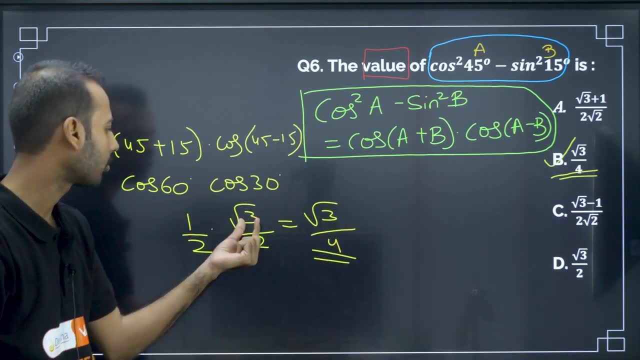 this cos 60, cos 30. everybody knows the values in 10 standard. only they will teach all this cos 60, cos 30, all these values. So root 3 by 4. hardly this will take 10 or 15 seconds. just you just have to substitute this. So do not leave trigonometry. trigonometry is very. 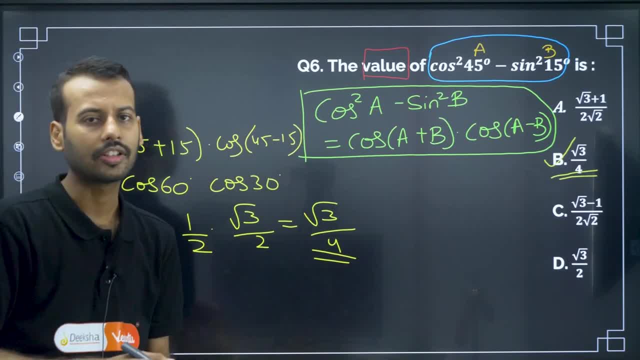 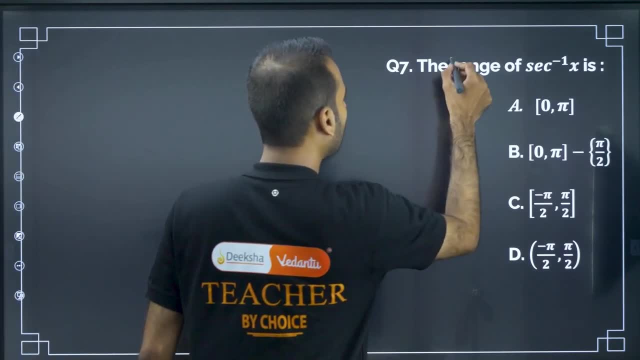 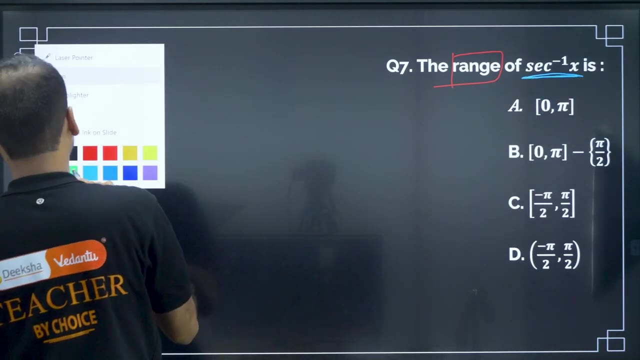 important chapter And inverse trigonometry generally. they will consider this as trigonometry only. moving on to next question, The range of secant inverse x is- see this question- the range of secant inverse x is. they are asking to find range of secant inverse x. Now, range of secant. 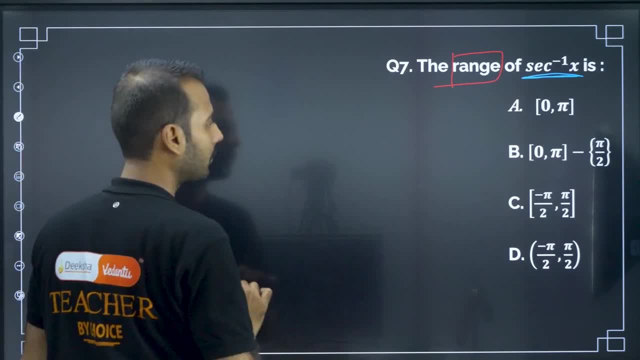 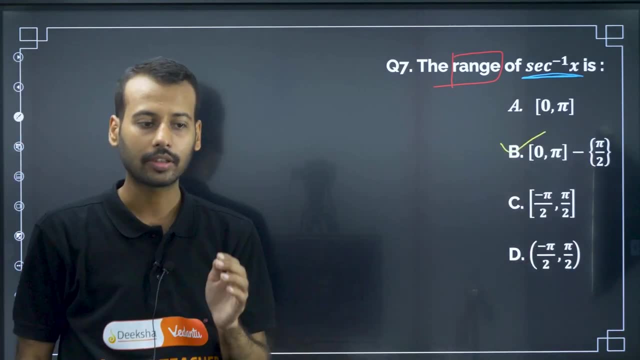 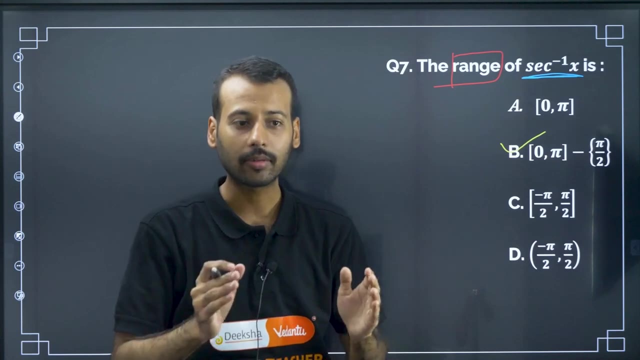 inverse x is range of secant inverse x is 0 to pi minus pi by 2.. So in inverse trigonometry, chapter, Chapter 2.. Second PUC, inverse trigonometry, range of secant inverse is 0 to pi minus pi by 2, one table. 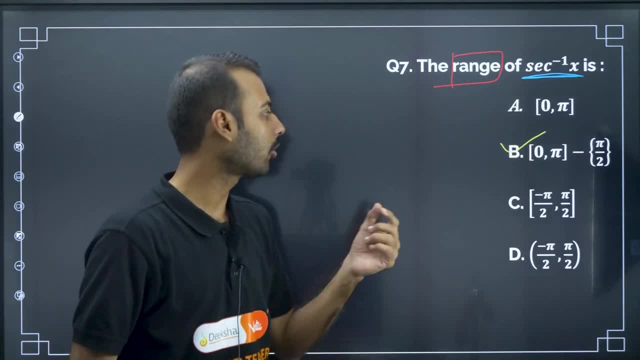 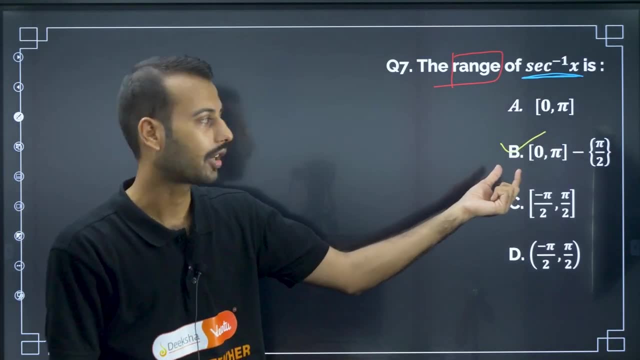 is there sin inverse cos, inverse, tan inverse cos, xx. the table you have to remember. So the moment you see range of secant inverse 0 to pi, only just to tick you need time. that is 1 second or hardly 2 seconds. So this is the answer: 0 to pi minus pi by 2.. So trigonometry. 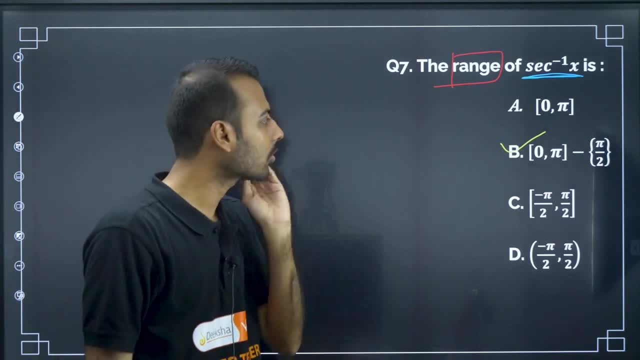 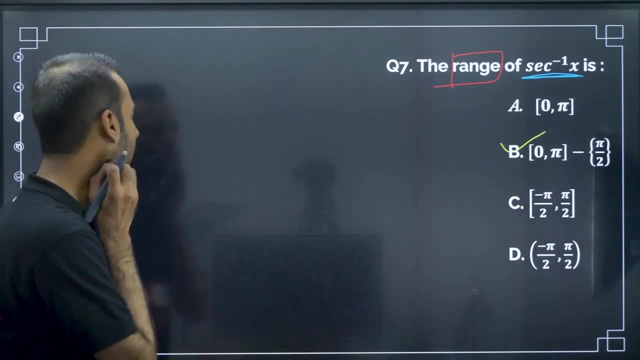 and inverse trigonometry. nobody should leave. So, if I know this synopsis: 0 to pi minus pi by 2, just only 1 second. within 1 second, 1 marks. So the remaining time you can give for time consuming questions. 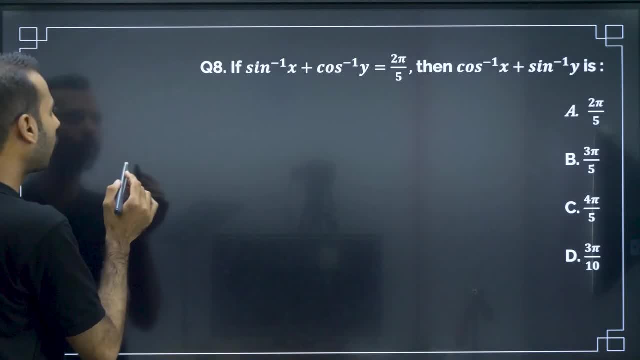 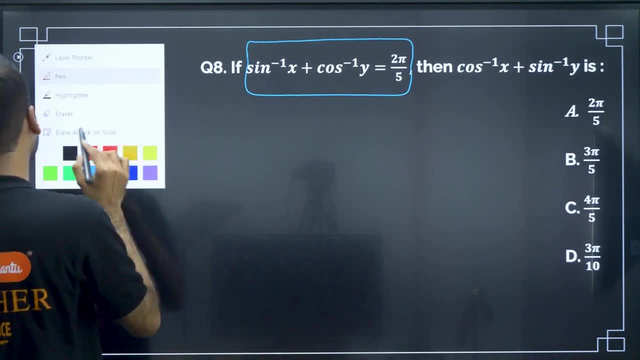 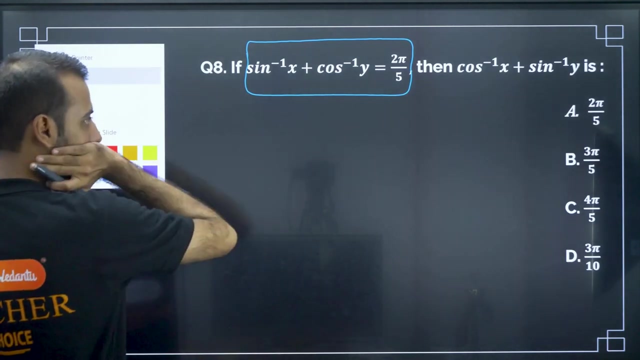 Moving on to next question, If one equation they have given one, if sin inverse x is equal to sin inverse x plus cos inverse y is equal to, then cos inverse x they are asking to find. what are they asking to find? cos inverse x plus sin inverse y is what are they asking? 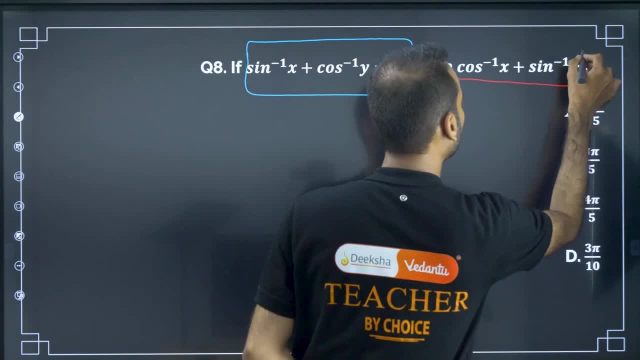 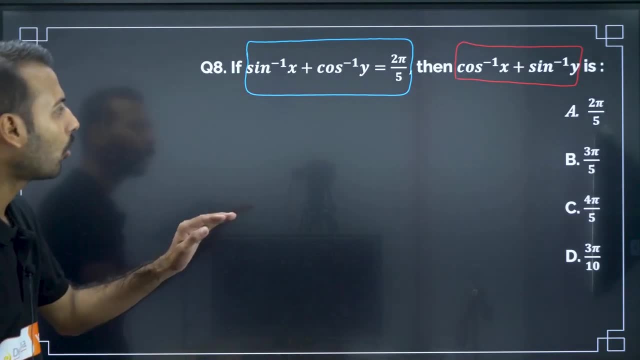 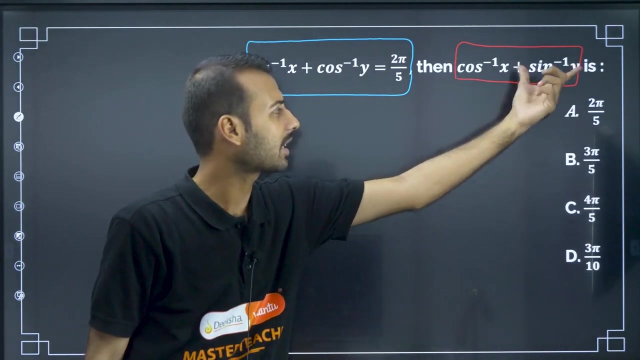 then they are asking to find cos inverse. Now they are asking this value, So they are asking this value. so what have they given and what are they asking? they have given some equation in terms of sin inverse x, cos inverse y, but they are asking cos inverse x, sin inverse y. so the moment you see, 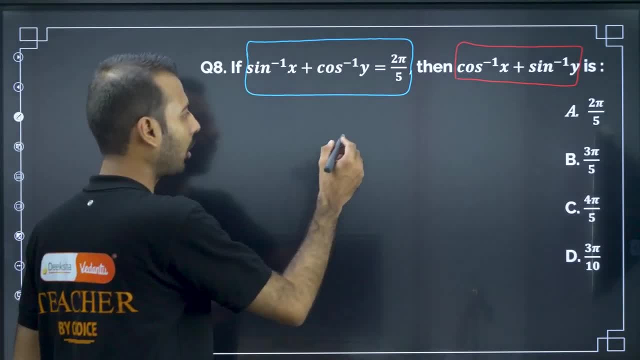 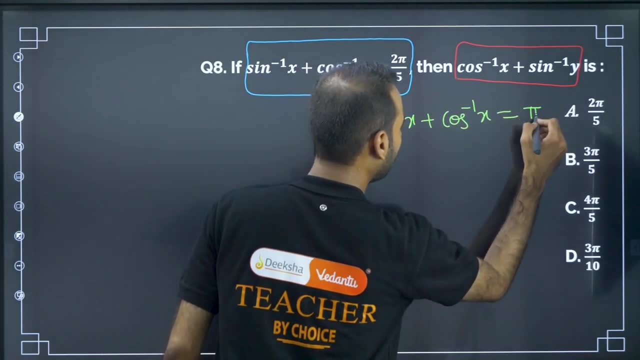 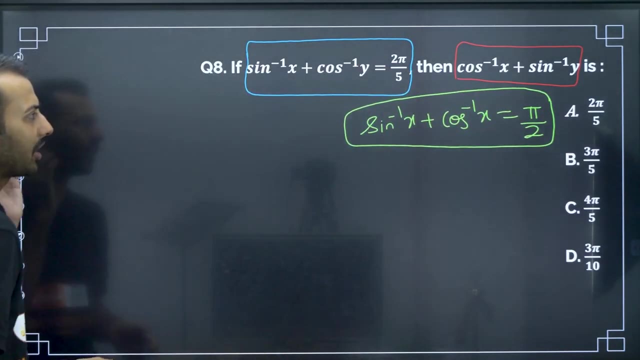 sin inverse x. there is one relation between sin inverse x and cos inverse x. what is that relation? sin inverse x plus cos inverse x is equal to pi by 2 is equal to pi by 2. if you know this relation, this problem is solved. so here how to approach this: sin inverse x in place of sin inverse x i. 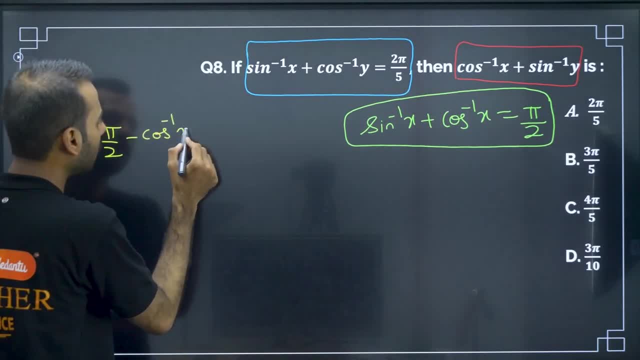 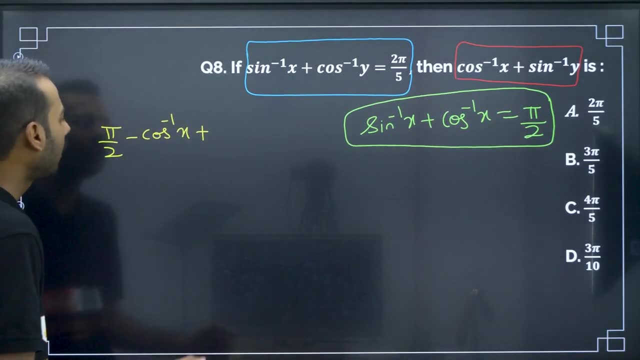 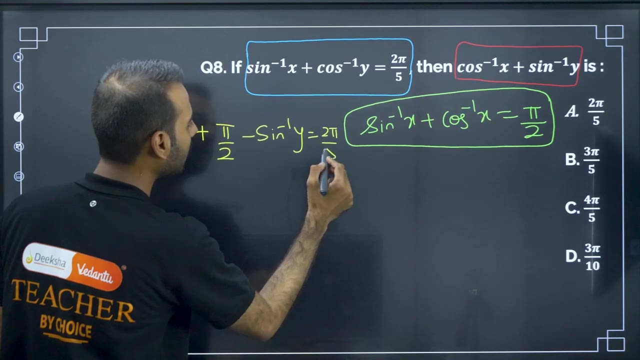 will write pi by 2 minus cos inverse x, cos inverse x plus. in place of cos inverse y. in place of cos inverse y, i will write: pi by 2 minus sin inverse y is equal to 2. pi by 5 is equal to 2. pi by pi by 2. pi by 2, this becomes pi by 2 minus cos inverse x. 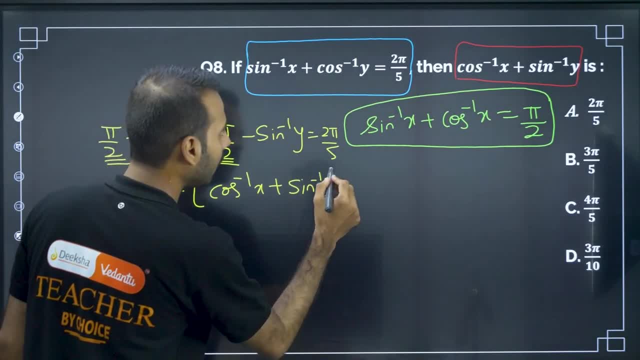 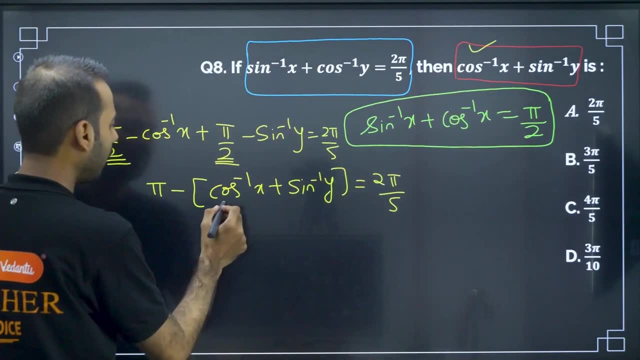 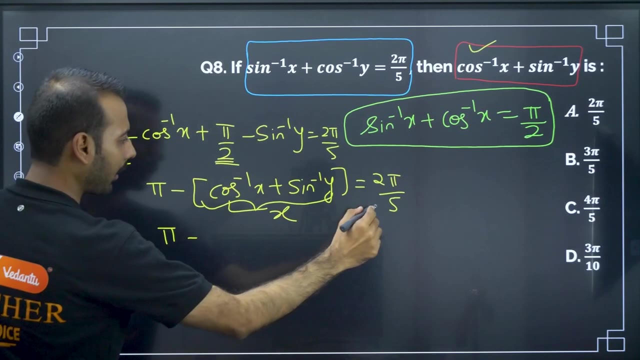 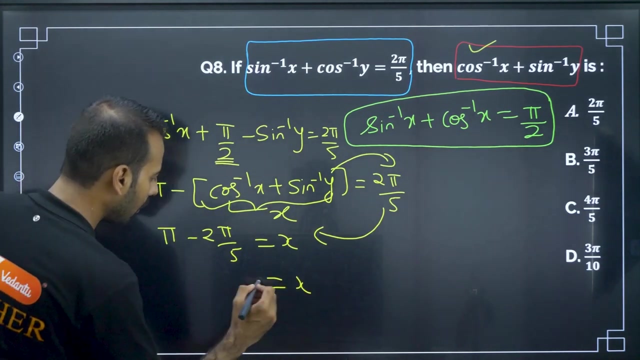 plus sin inverse y is equal to 2 pi by phi. now see the question: cos inverse x plus sin inverse y, this one, and here also same thing. so if i name this as x, if i name this as x, pi minus, if i transpose this to this side, if i transpose this pi minus 2 pi by phi is equal to x. so x is equal. 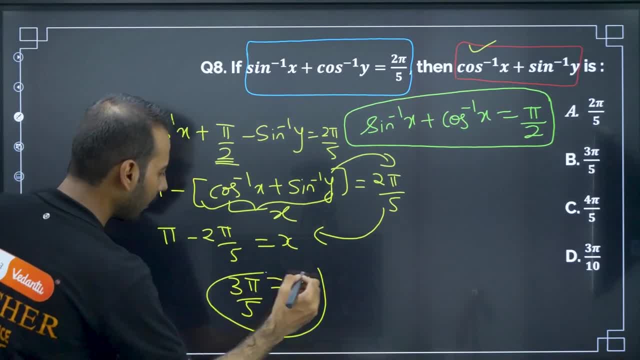 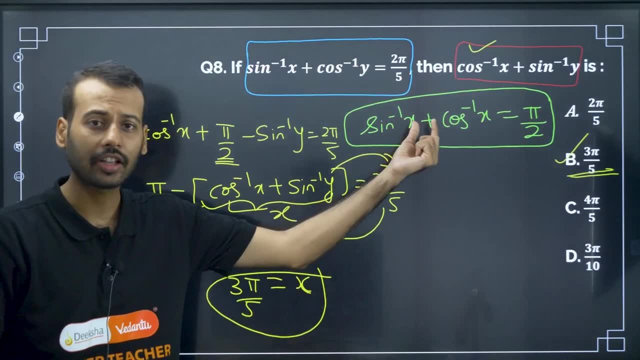 to 3 pi by phi. x is equal to 3 pi by phi. so is there any such option? x is equal to 3 by phi. yes, b is the answer. so again, easy question: only only one identity, if you know you are getting one marks. so trigonometry and inverse trigonometry. please don't leave this, don't skip this chapter if you. 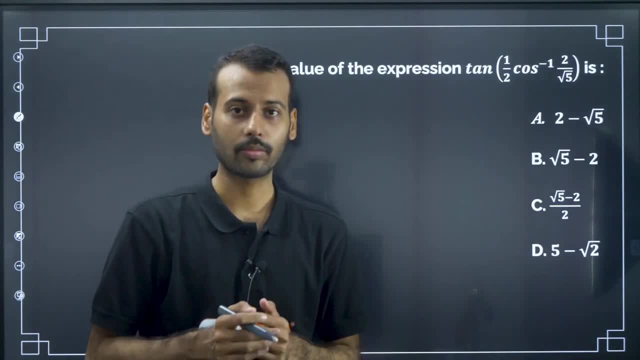 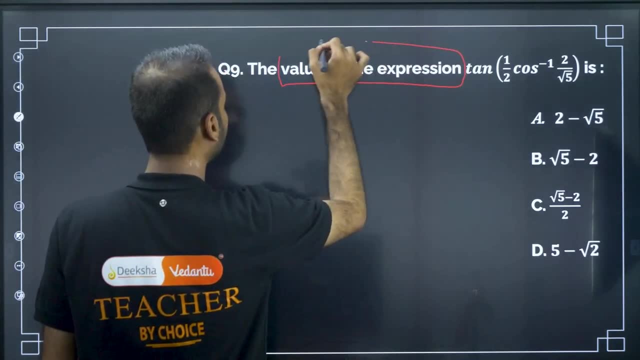 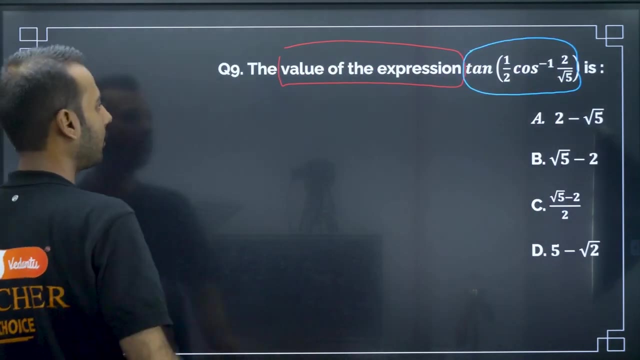 want to skip any, any other chapter. if you want to skip any other chapter because of time constraint, you can skip, but don't leave this. next, the value of expression. again they are asking the value of expression, one expression they have given. what is that expression? tan, tan of something they have given tan of for this. let me copy and paste that expression. 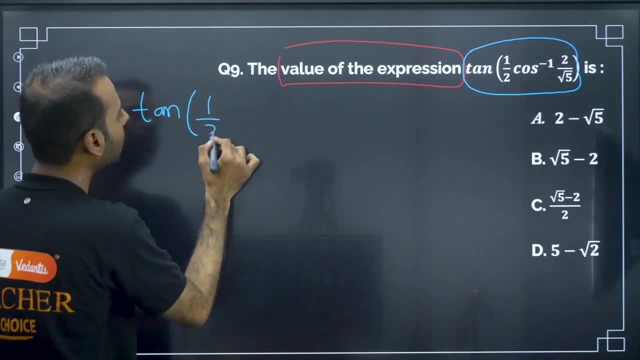 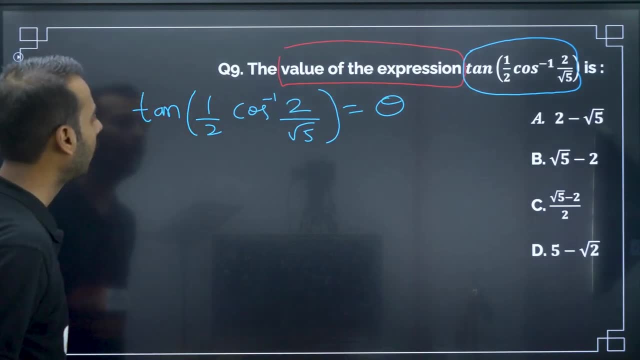 tan of 1 by 2 cos inverse 1 by 2 cos inverse 2 by root phi. 2 by root phi is equal to theta. let let me call whatever they have given as theta. now, if i apply tan inverse on both sides, this becomes 1 by 2 cos inverse 2 by root phi. 2 by root phi is equal to. 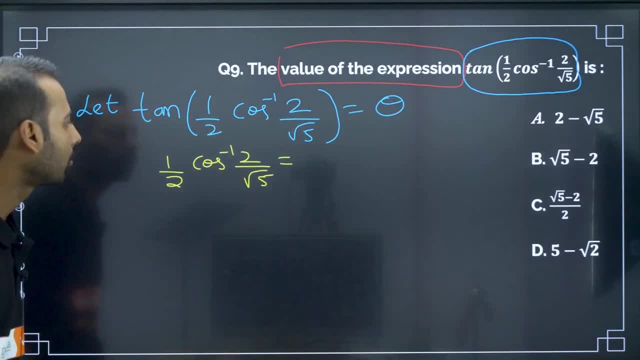 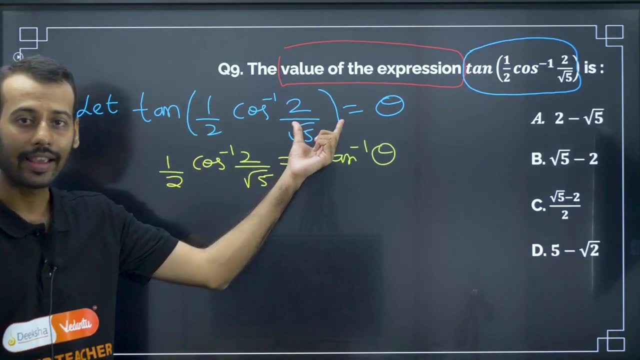 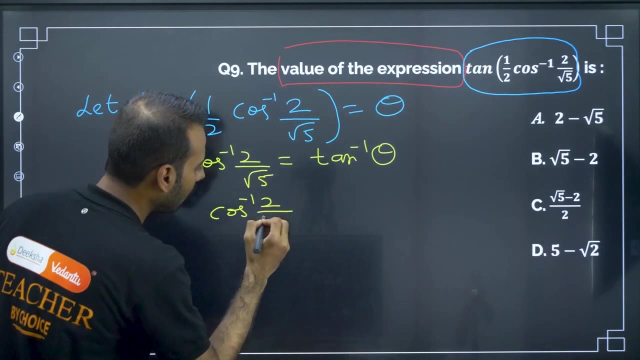 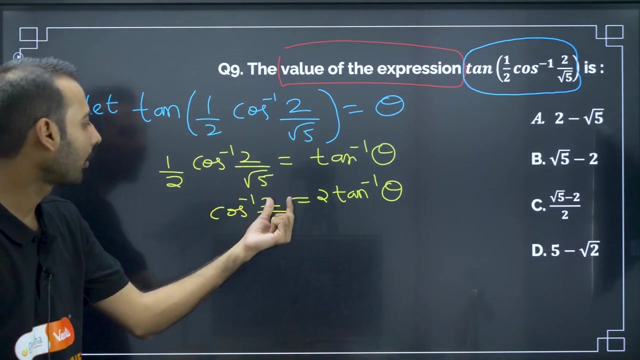 1 by 2 cos inverse 2 by root phi is equal to tan inverse theta, tan inverse theta: see here for this equation i am applying tan inverse on both sides, so tan inverse- this now cos inverse, cos inverse 2 by root phi is equal to 2 tan inverse theta, 2 tan inverse theta, cos inverse 2 by root. 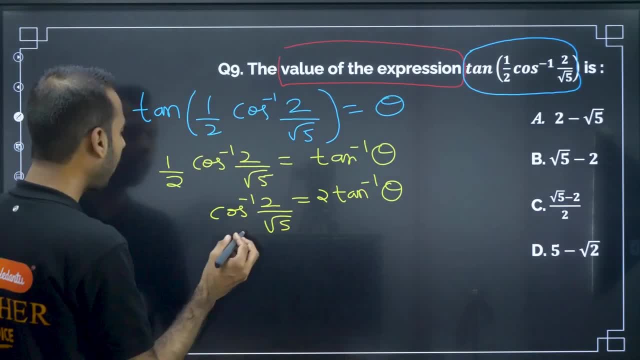 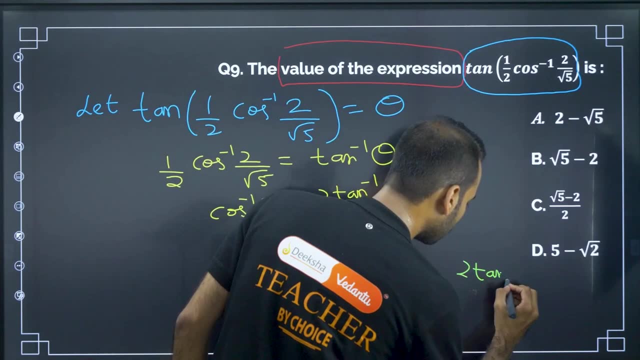 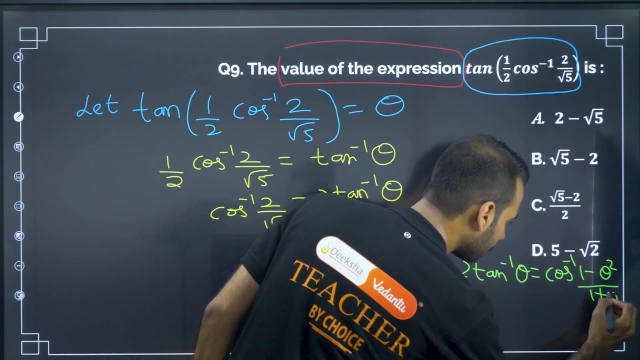 phi is equal to 2 tan inverse theta. Next now, one synopsis point. you should be able to recall at this point: 2 tan inverse theta. 2 tan inverse theta is equal to cos inverse 1 minus theta square by 1 plus theta square. So 2 tan inverse theta is equal to 2 tan. 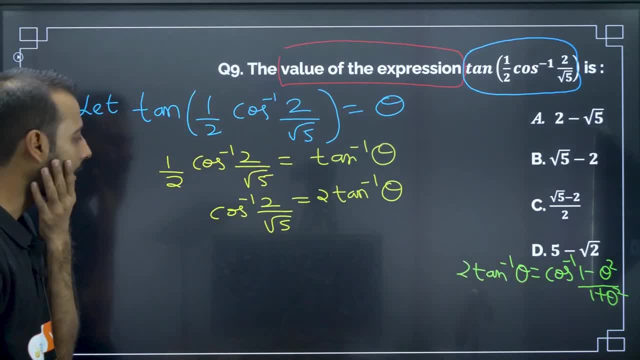 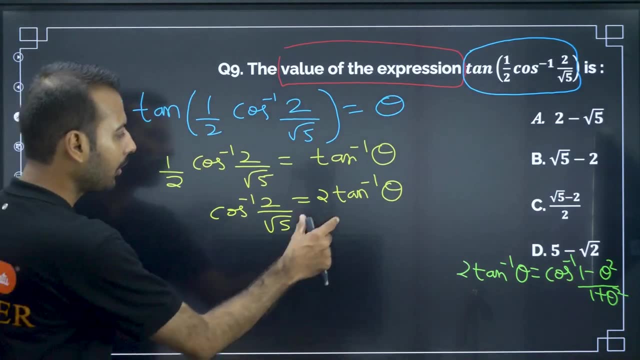 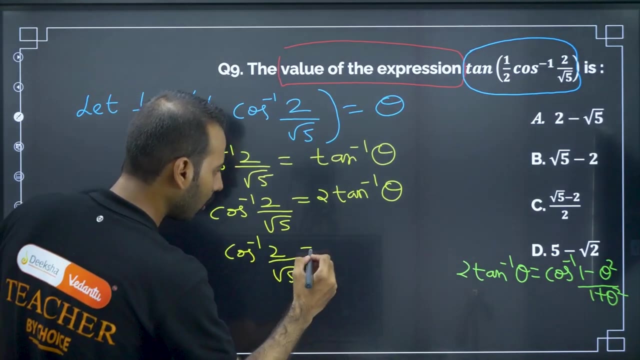 inverse theta is equal to cos inverse 1 minus theta 1 plus theta square. So cos inverse 2 by root 5 is equal to 2 tan inverse theta. Now you relate this 2 tan inverse theta. For that I will write this. let me copy and paste this: cos inverse 2 by root 5 is equal. 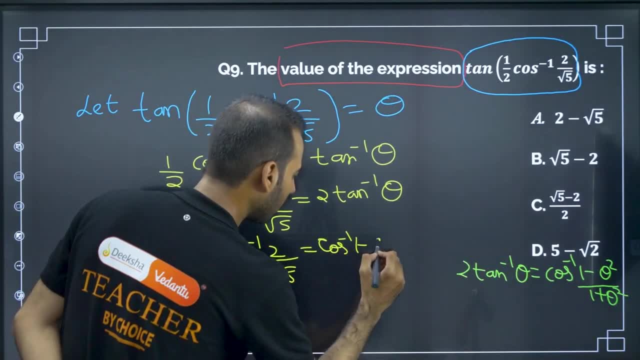 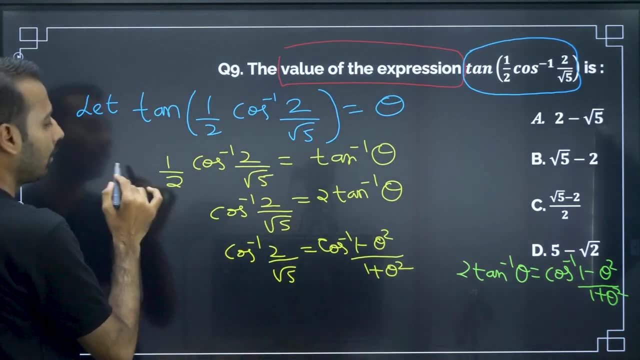 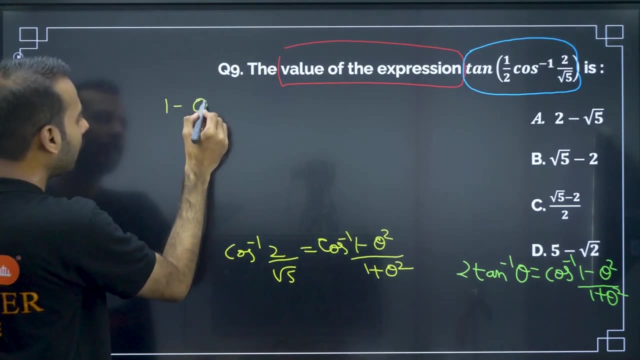 to cos inverse: 1 minus 1 minus theta square by 1 plus theta square. So cos inverse, cos inverse. finally, from there, I am just copying, Copy and pasting. let me erase this for simplification: 1 minus theta square by 1 plus theta square. 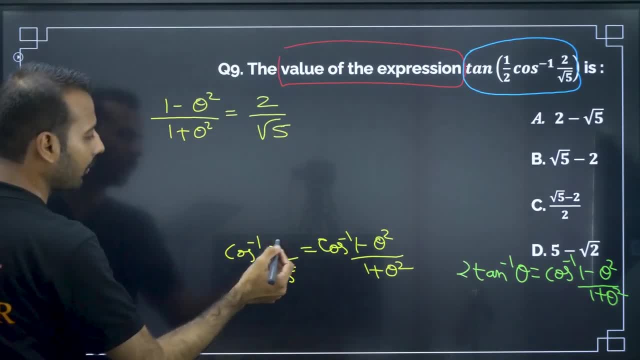 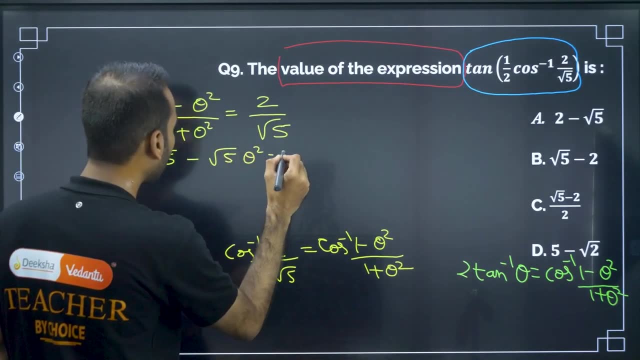 is equal to 2 by root 5 cos inverse. if I apply cos function on both sides, Now root 5 minus root 5 theta square is equal to 2 plus 2 theta square. 2 plus 2 theta square. 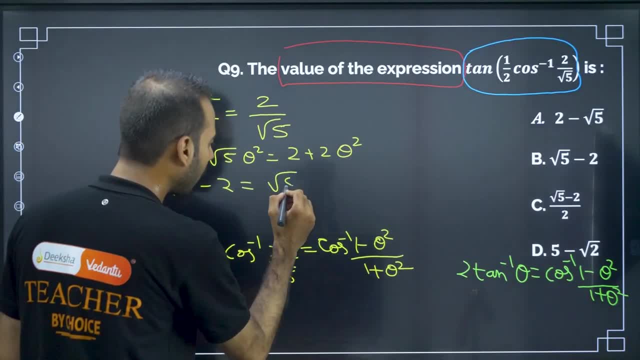 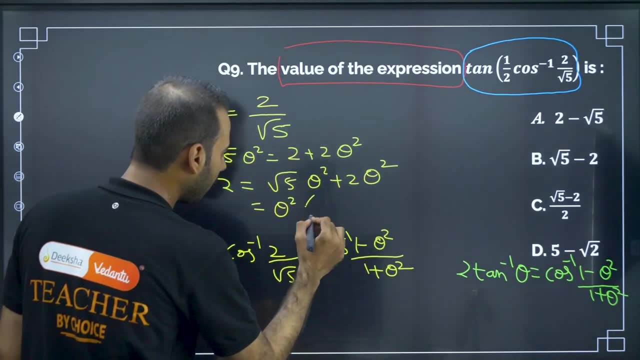 So root 5, root 5 minus 2 is equal to root 5, theta square plus 2 theta square. So if I take theta square common this side here, I am left with root 5 plus 2 root 5 plus. 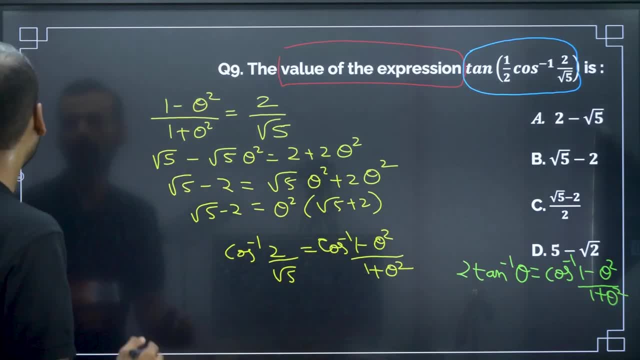 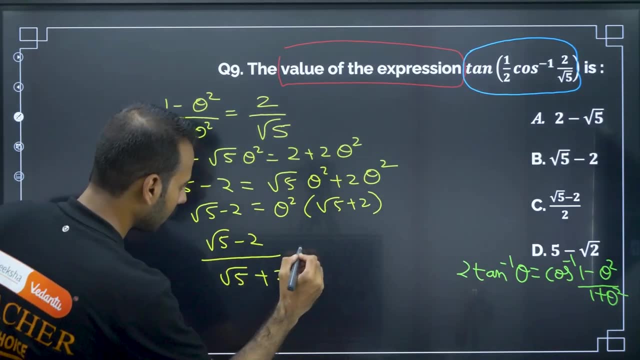 2 here. root 5 minus 2, root 5 minus 2.. Now let me erase this root 5 minus 2. by root 5 plus 2 is equal to theta square is equal to root 5 minus 2. by root 5 plus 2 is equal. 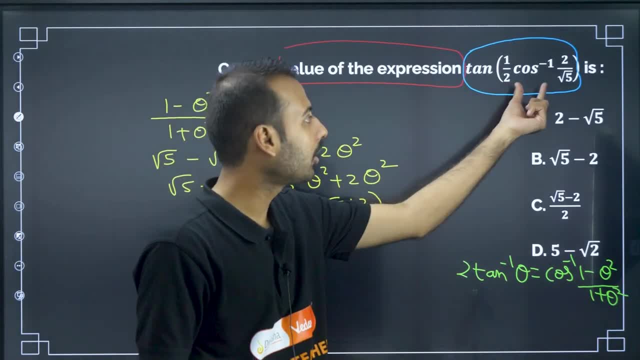 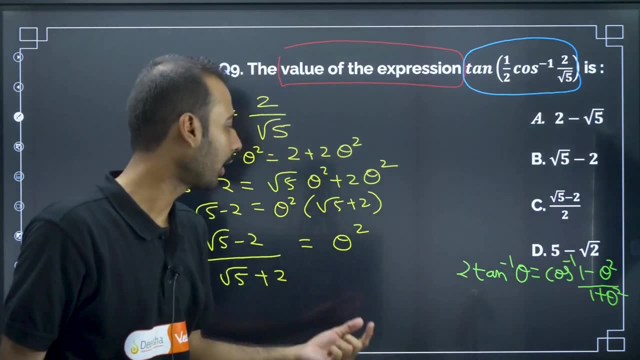 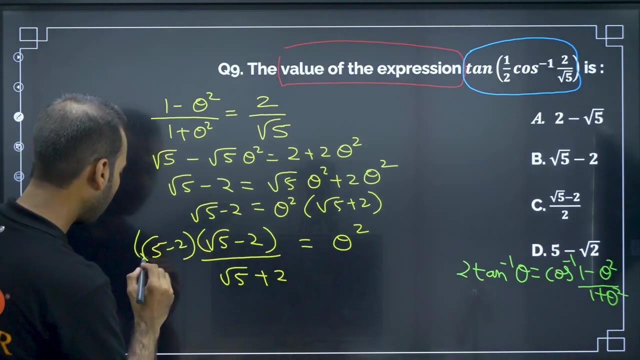 to theta square. Now for this expression. we have named this as theta. try to recall in the previous when we started problem this. So we are supposed to find value of theta. So to find value of theta, let me multiply this with root 5, root 5 minus 2, and here: 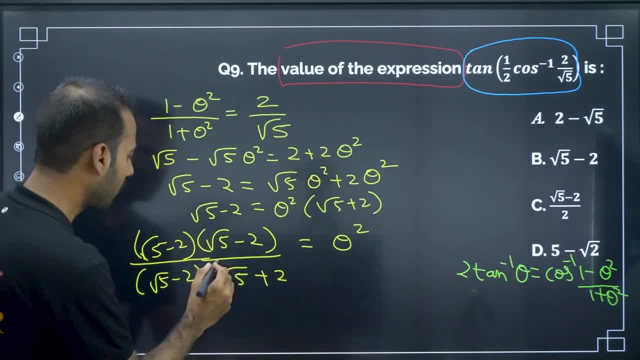 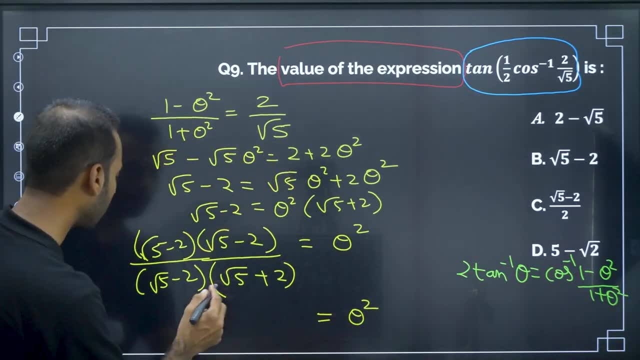 also root 5 minus 2. root 5, minus 2, phi minus 2, just, I am multiplying root 5 minus 2, root phi minus 2.. So here we will get theta. square is equal to: this is 1, this is root 5 minus. 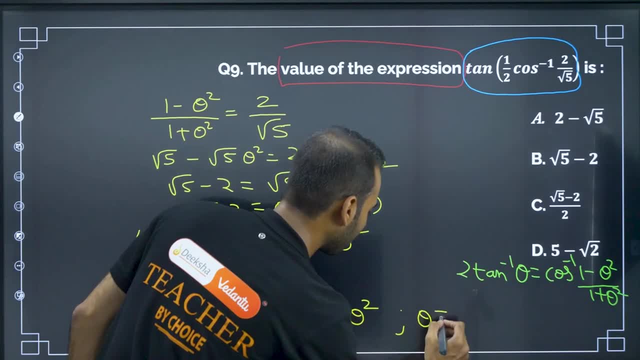 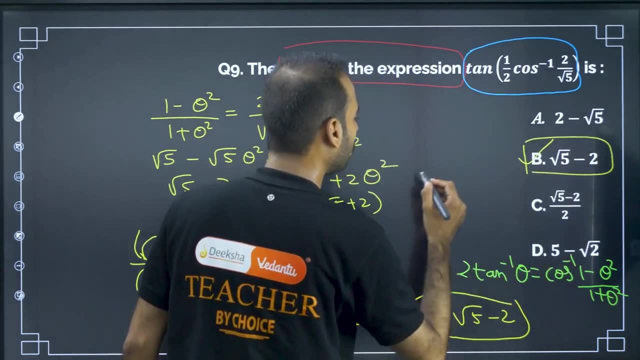 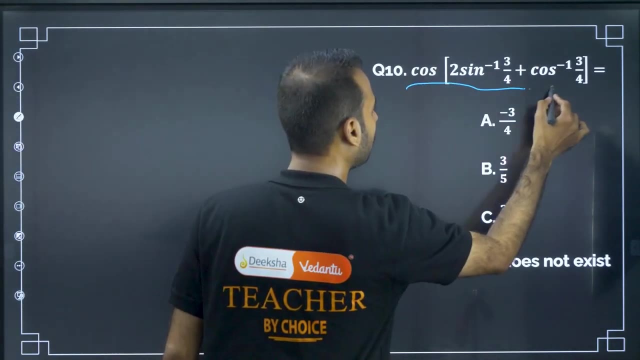 2 square. So theta is equal to. theta is equal to root 5 minus 2.. minus 2, theta is equal to root 5 minus 2.. So b is the answer for this. Moving on to next question: cos of? they have given some expression. cos of 2, sin, inverse this and they: 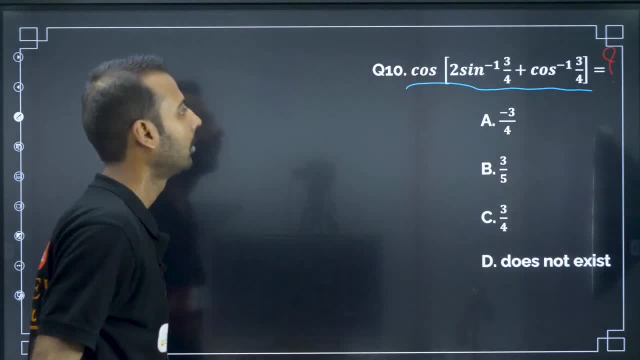 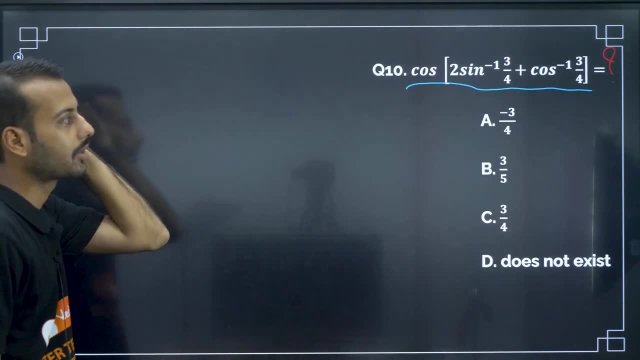 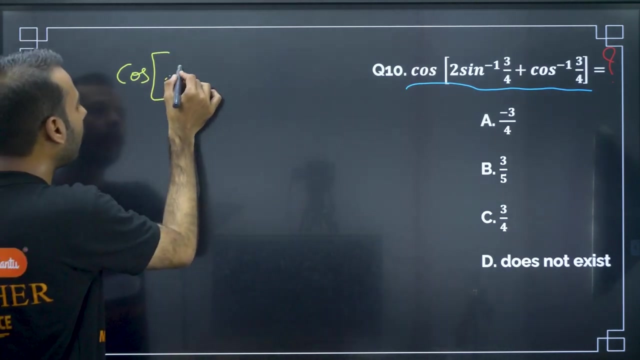 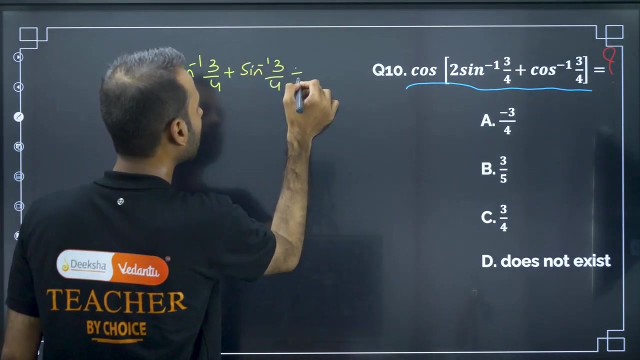 are asking to find what is the cos of something. we have to find a value of this. So how to approach this? cos of 2 sin inverse 3 by 4 plus cos. Now let me write that cos of 2 sin inverse. for that let me write sin inverse 3 by 4 plus sin inverse 3 by 4 plus cos inverse. 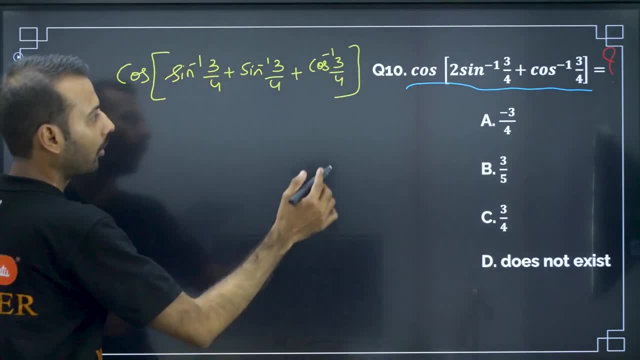 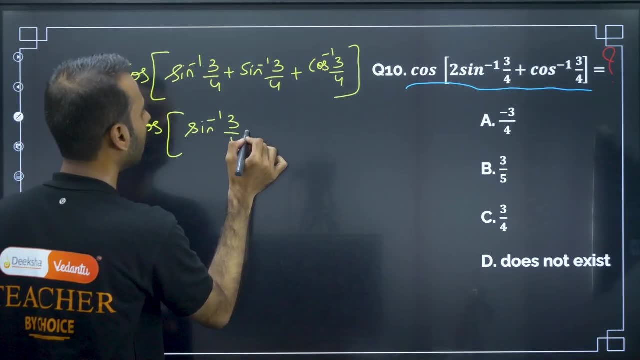 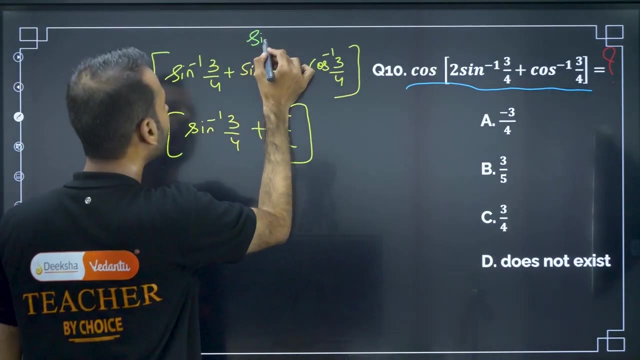 cos inverse 3 by 4.. So for this 2 sin inverse 3 by 4, I am writing like this: cos of sin inverse 3 by 4 plus pi by 2, pi by 2 from synopsis. try to recall sin inverse x plus sin inverse. 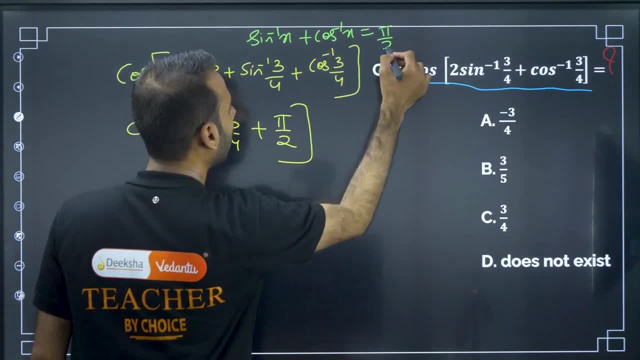 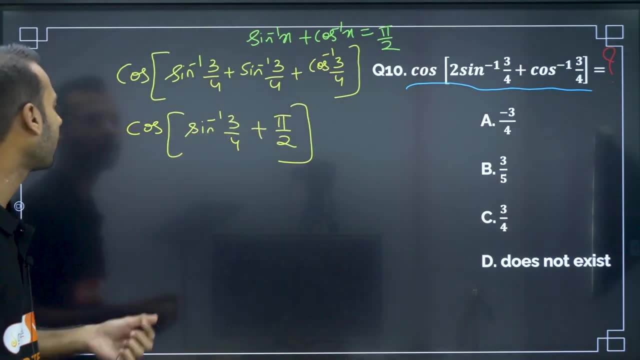 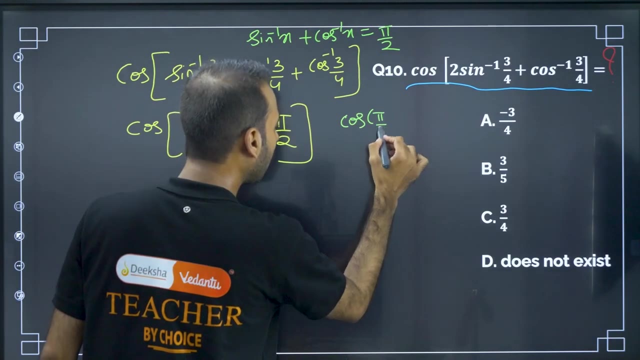 4 plus cos inverse x is equal to pi by 2.. So sin inverse 3 by 4 plus cos inverse 3 by 4. I am writing like this. Now one more synopsis point. you should be able to recall what is that cos of pi by 2 plus theta is: 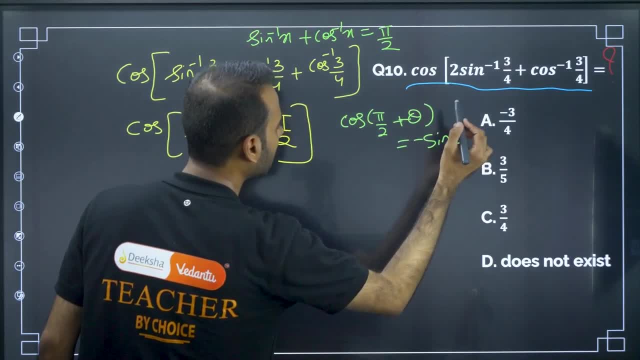 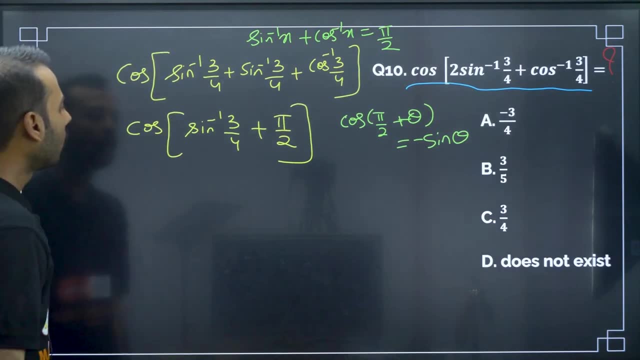 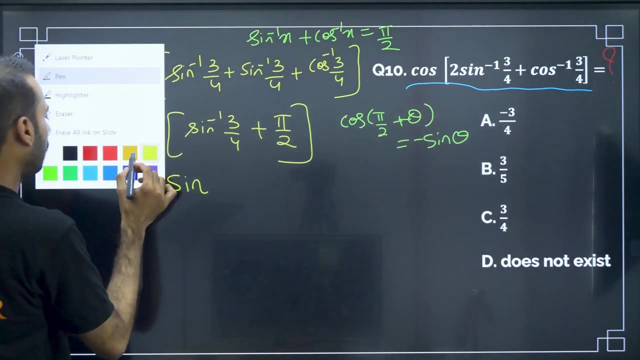 equal to negative sin theta is equal to cos of pi by 2 plus theta is equal to negative sin theta. so cos of pi by 2 plus theta is equal to negative sine theta, so negative sine. if you observe here, if you observe here, if i name this as theta, if i name this as cos of pi by 2 plus theta, means 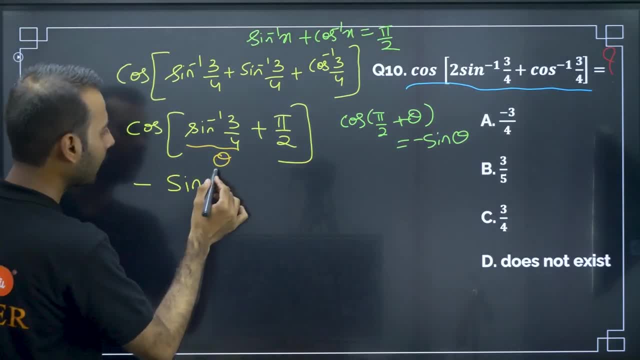 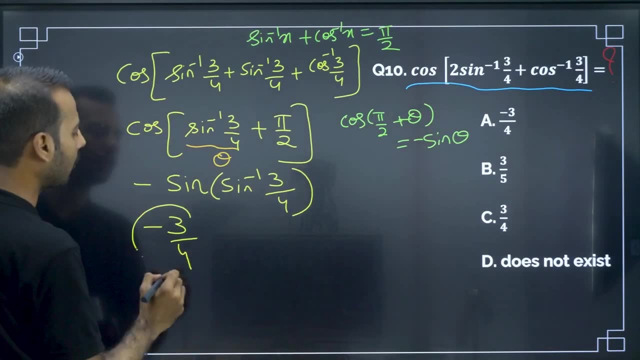 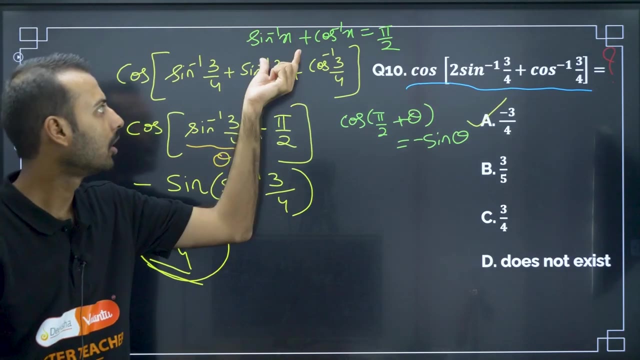 negative sine theta. so negative sine theta is sine inverse 3 by 4. so this becomes minus 3 by 4. is there any such option? minus 3 by 4: yes is the answer. moving on to next question, see, this is also very easy question. just one, two identities you should be knowing, and then simplification. 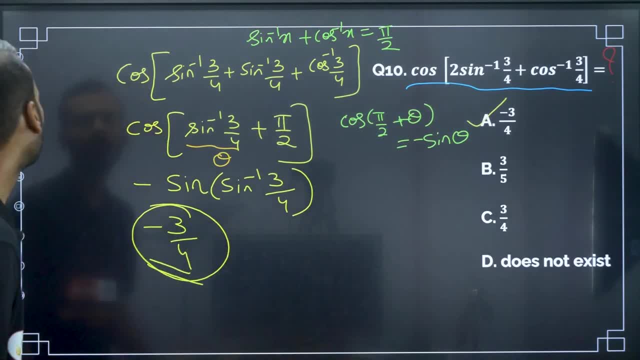 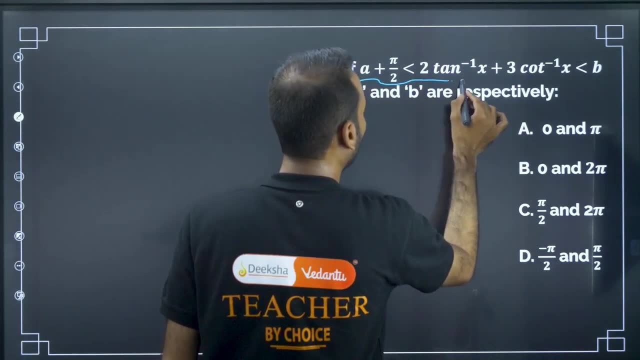 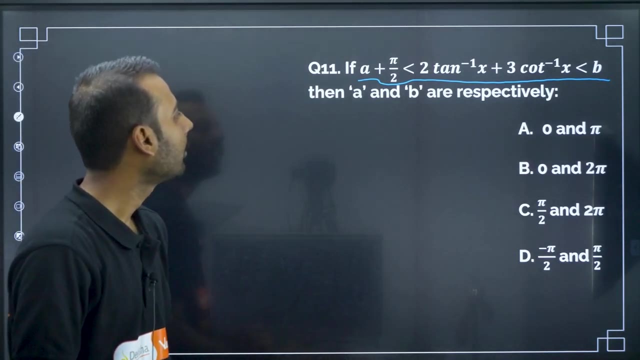 within within 30 or 40 seconds, you will get the answer. moving on to next question, if they have given one identity, a plus pi by 2, all this b, a plus pi by 2 less than 2, tan inverse x plus 3, cot inverse x is less than b. then a and b are respectively. what are they asking? they are asking: 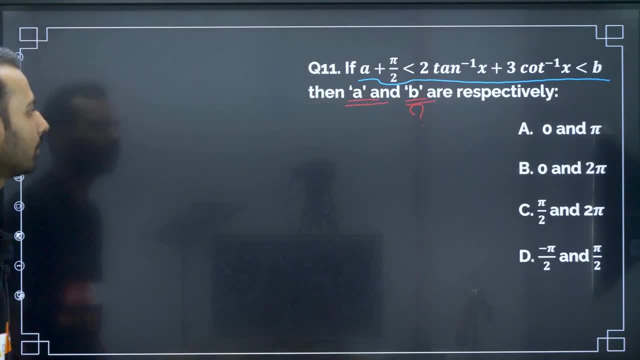 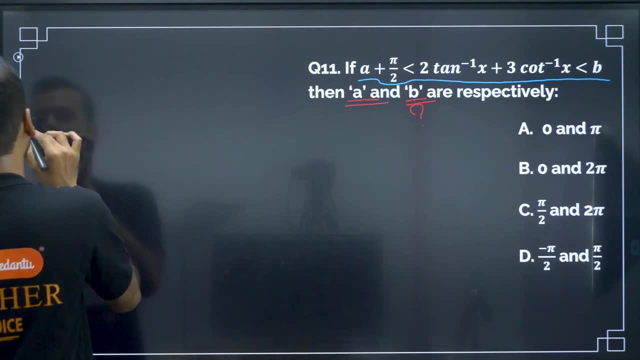 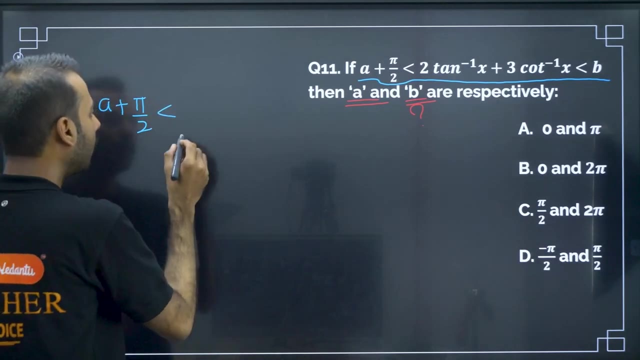 a and b are respectively: what a and b are respectively: a plus pi by 2 less than 2 tan inverse x. so just let me copy and paste that a plus pi by 2 less than less than 2 tan inverse x. just i am copying: plus 2 cot inverse x. 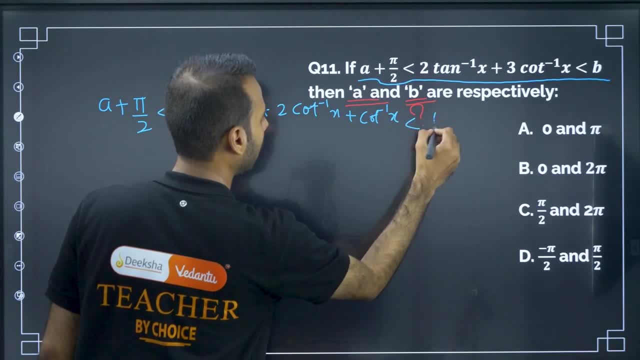 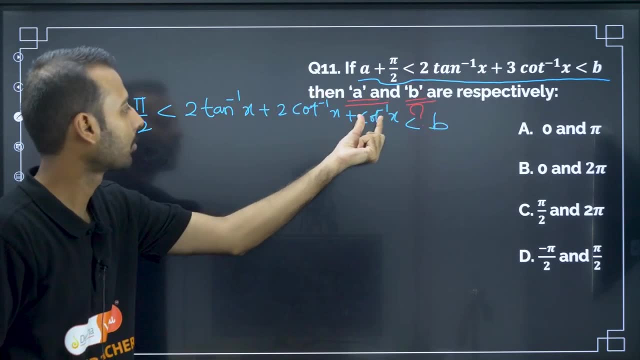 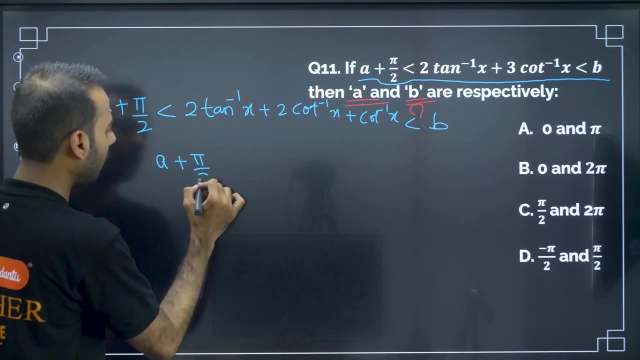 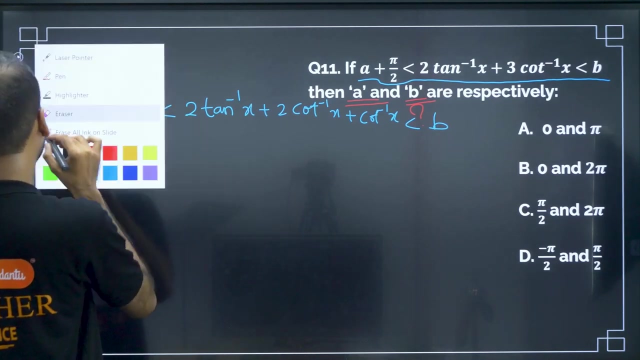 plus cot inverse x, less than b. for three: cot inverse x, i am writing 2 cot inverse x plus cot inverse x. now next a plus pi by 2. a plus pi by 2 less than 2. this for this: a plus pi by 2. i am keeping as it is this symbol. also now for this: 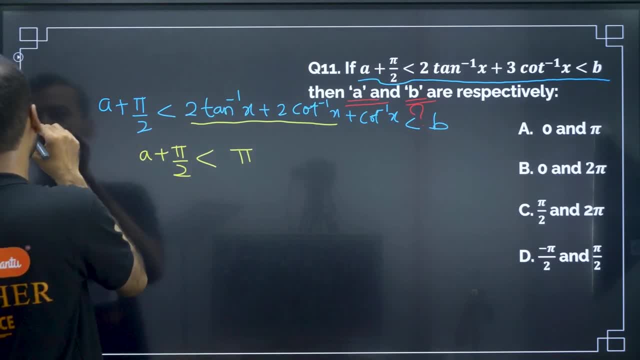 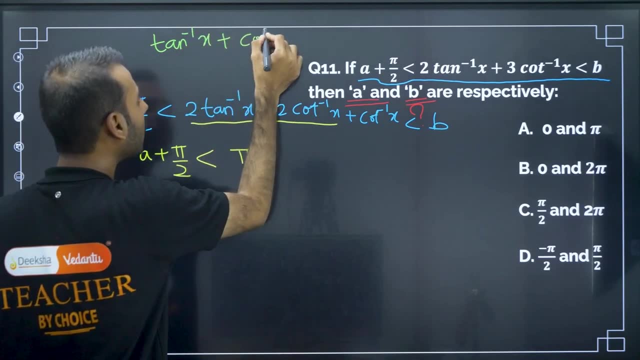 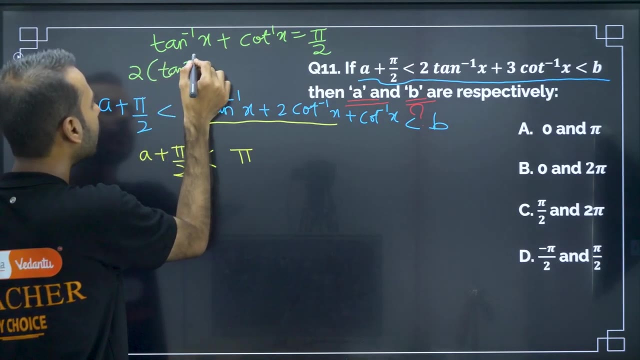 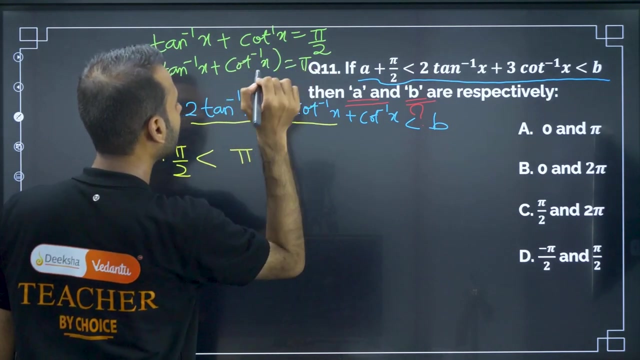 i will write this as pi, the reason why i am writing pi. one synopsis point should come to your mind: tan inverse x plus cot. inverse x is equal to pi by 2: 2. tan inverse plus 2. tan inverse x plus 4: inverse x is equal to pi is equal to pi. 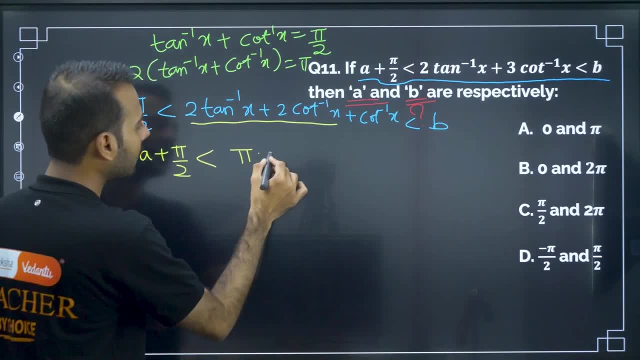 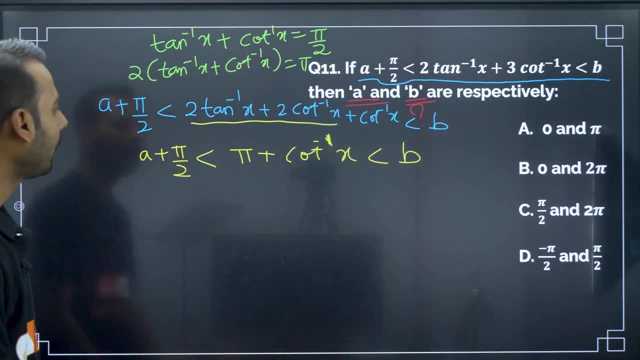 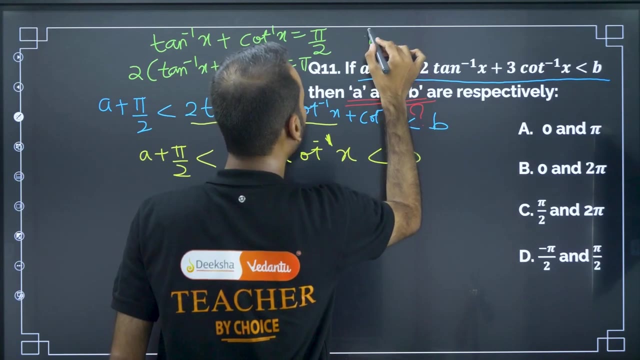 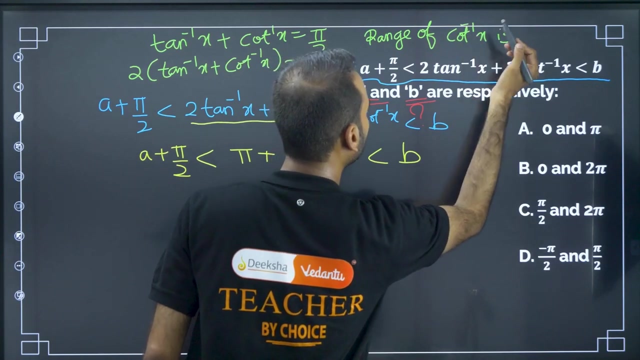 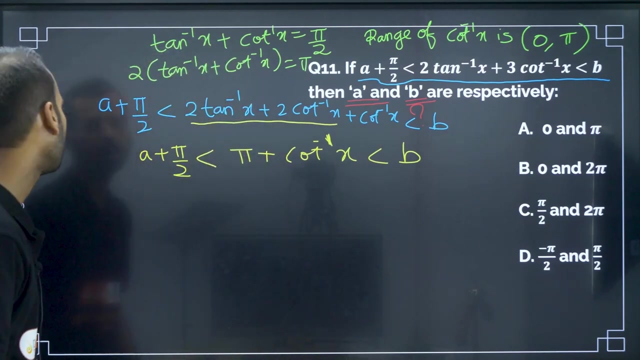 so a plus pi by 2 is less than pi plus cot inverse x. cot inverse x less than b. less than b. now try to recall the range of cot inverse x. range of range of cot inverse x. cot inverse x is 0 to pi, is 0 to pi. cot range of cot inverse x is 0 to pi. so a plus pi by 2. 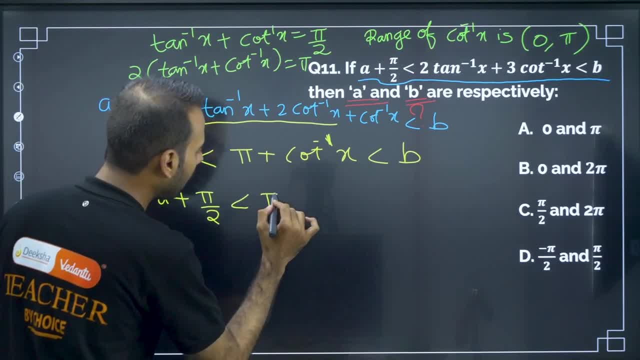 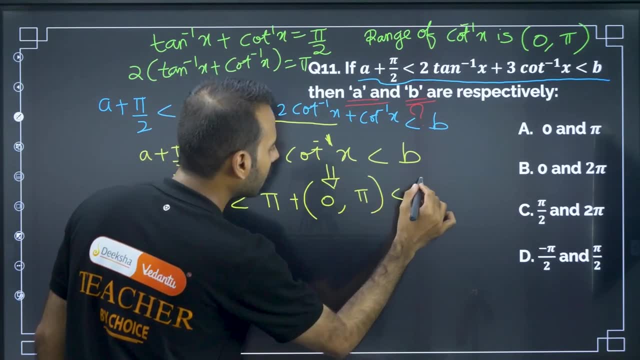 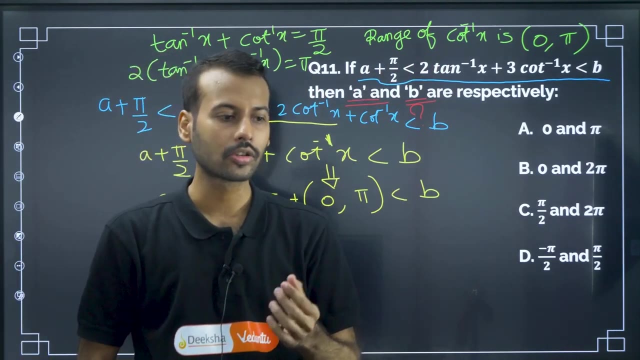 a plus pi by 2 less than pi. in place of this, this goes from max 0 to 0 to pi less than b. range of cot inverse x: see here for synopsis point in inverse trigonometry synopsis. what you have to remember is all the domain and range of sign, all those six inverse trigonometric. 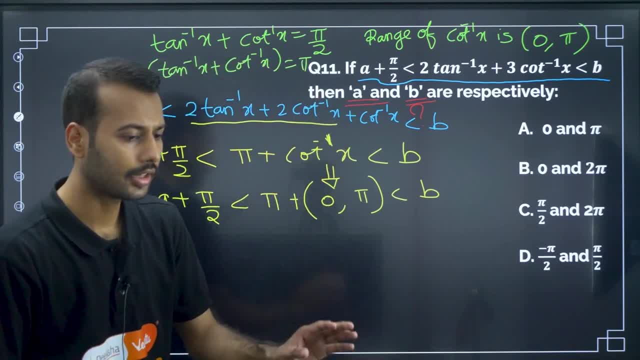 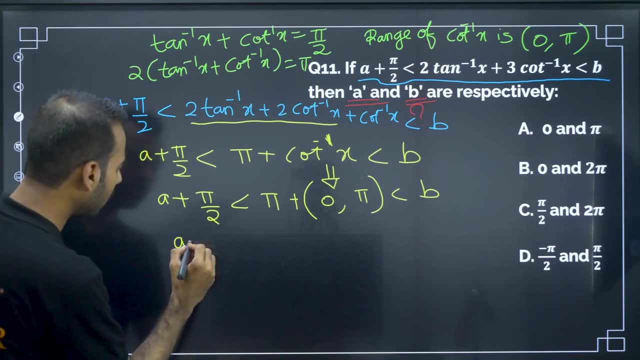 that is 100 percent mandatory, that that is the most important thing in that chapter itself. so now, if you see here, if you go for further synopsis point in inverse trigonometry synopsis point in inverse trigonometry, synopsis point: simplification: a plus pi by 2. a plus pi by 2 less than here, this is pi less than b, so or? 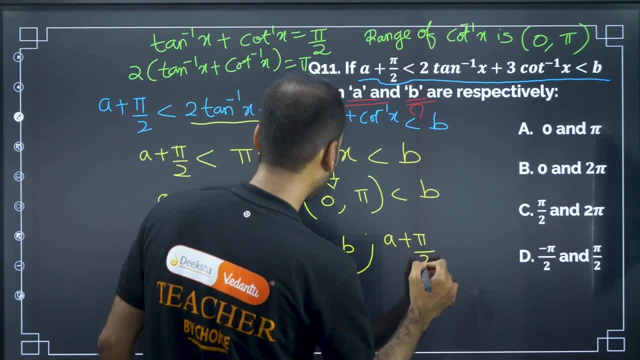 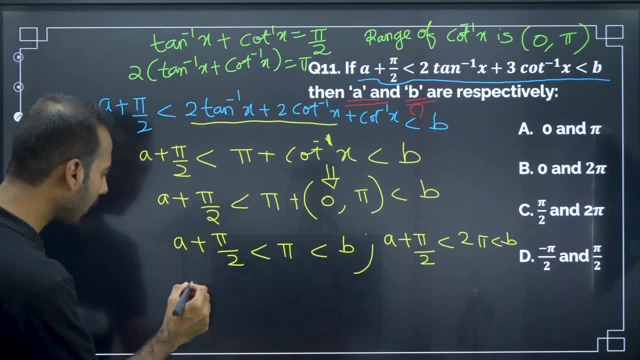 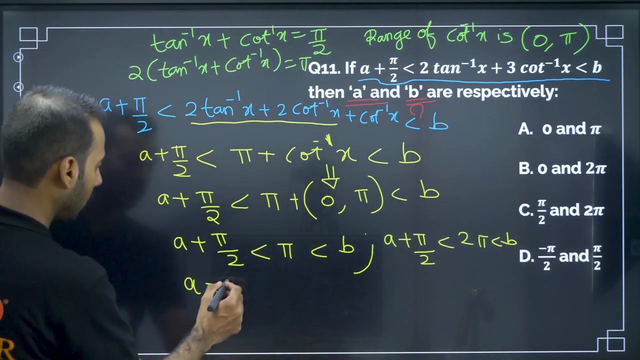 further, this can be written as: a plus pi by 2. less than 2, pi less than b. less than b. now in place of a, in place of a pi by 2. so this goes from pi to 2 pi. so a is equal to, a is equal to, a is equal to. from here we can come to a conclusion: a is equal to. 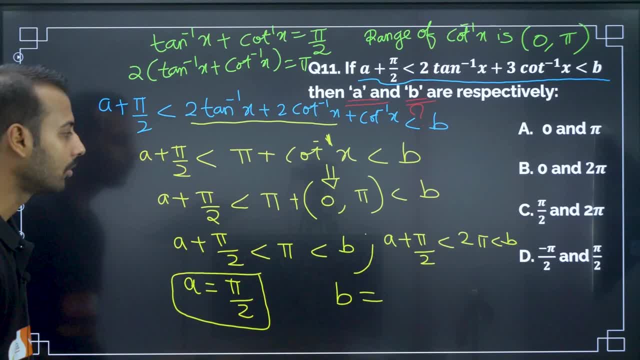 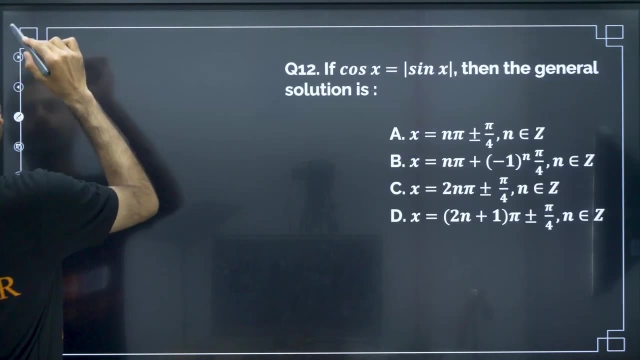 pi by 2 and b is equal to a is equal to 2 pi. a is equal to pi by 2 and b is equal to 2 pi, which is the answer. c is the answer. moving on to next question, if cos x is equal to some information, 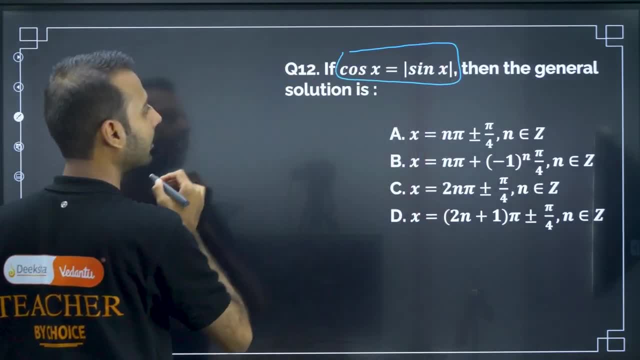 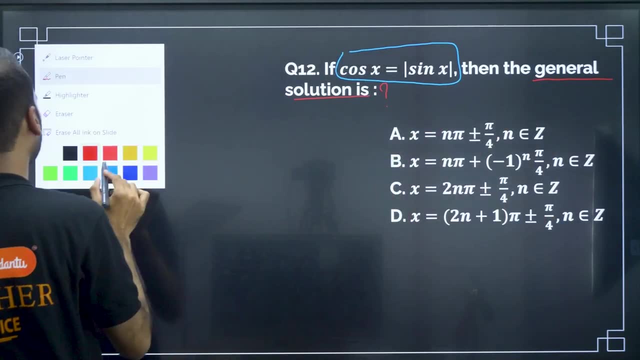 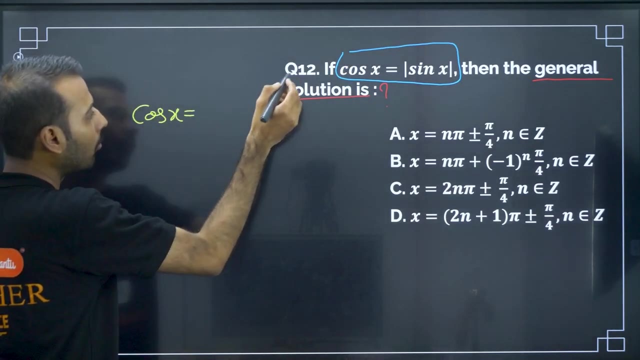 they have given. if cos x is equal to this, then the general solution is: what are they asking? they are asking to find general solution is: if cos x is equal to some, if cos x is equal to modulus of sin x, so cos x is equal to. cos x is equal to modulus of sin x means if i remove modulus i have. 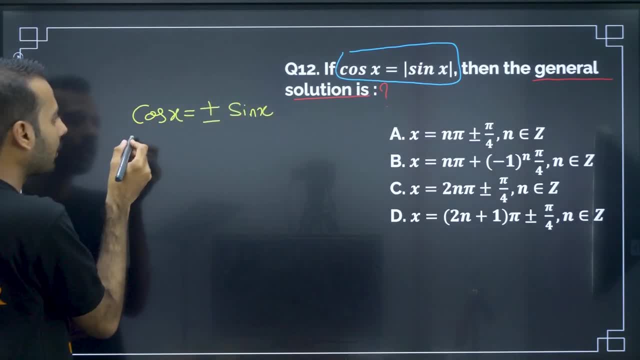 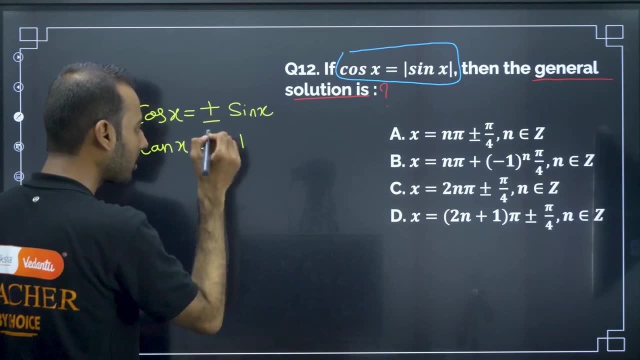 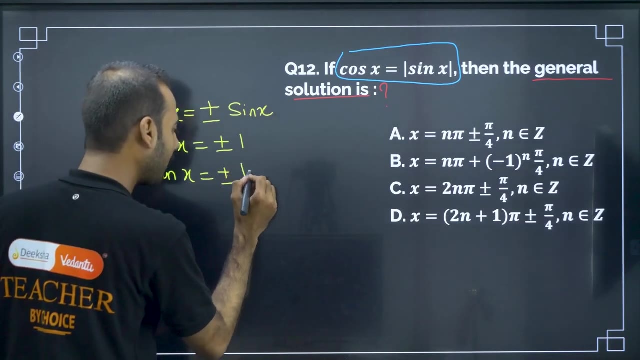 to write plus or minus. so cos x is equal to plus sin x or minus sin x. now for this. if i transpose this sin x, i can write: tan x is equal to plus or minus sin x. so if i transpose this sin x, i can r minus 1.. Now further, tan x can be written as tan x is equal to plus or minus tan pi by 4 tan. 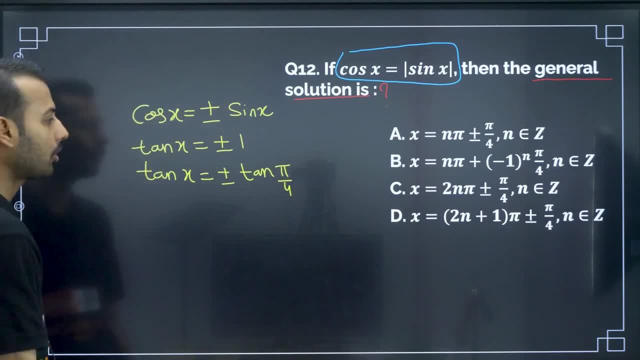 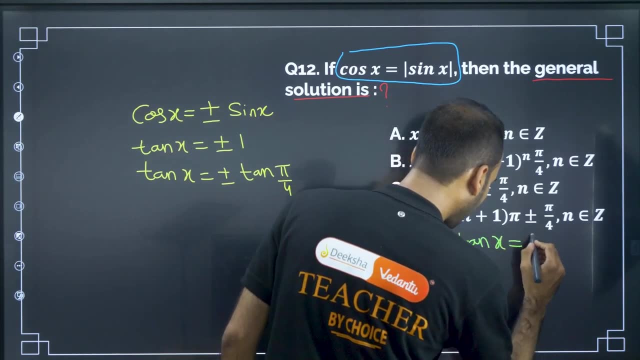 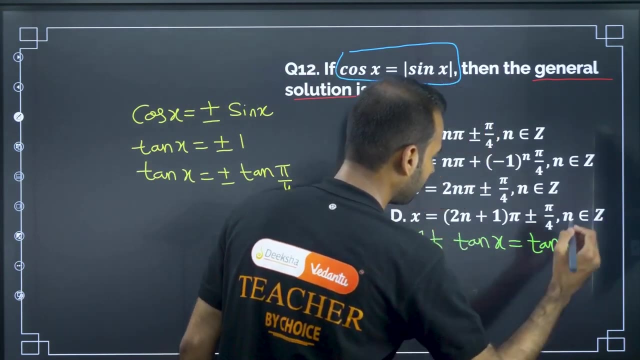 pi by 4.. Now one synopsis point you should be able to recall at this point: If, if tan x is equal to, if tan x is equal to tan, if tan x is equal to tan, pi by 4, sorry. if tan x is equal to tan, alpha. 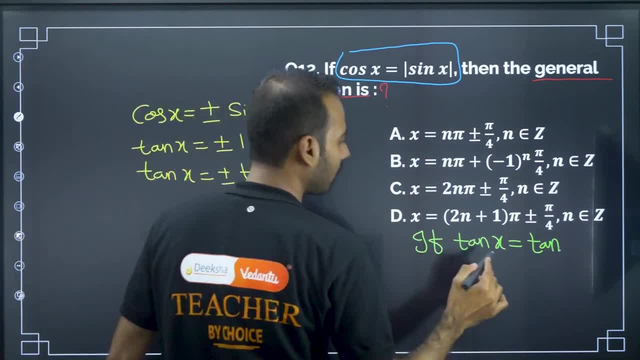 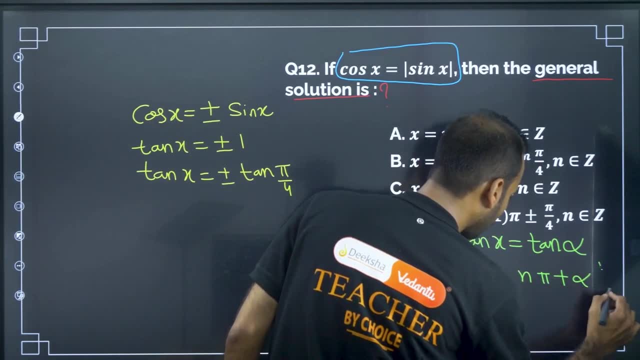 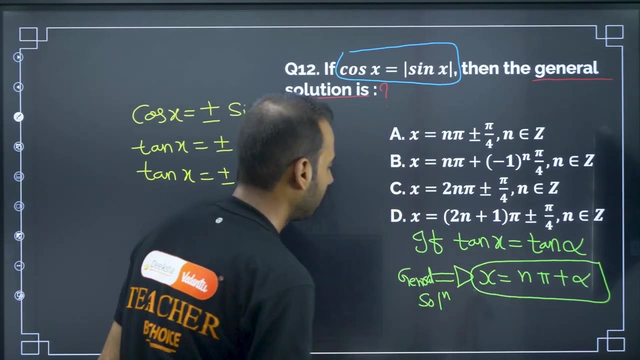 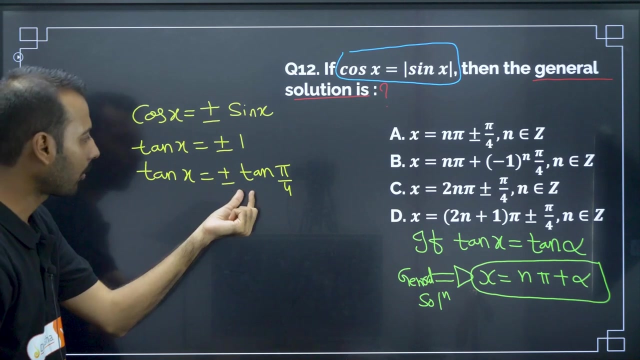 if tan x is equal to tan alpha, then x is equal to n pi plus alpha. General solution is given by general general solution. If tan x is equal to tan alpha, x is equal to n pi plus alpha. Now tan x is equal to plus or minus tan pi by 4.. So x is equal to, x is equal to. 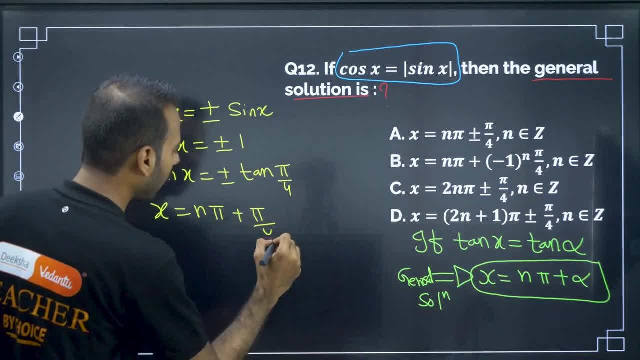 n pi by 4.. So x is equal to. x is equal to n pi by 4.. So x is equal to. x is equal to n pi by 4.. n pi plus pi by 4, or if I take minus, so n pi plus or minus 4, is there any such option? x is equal to. 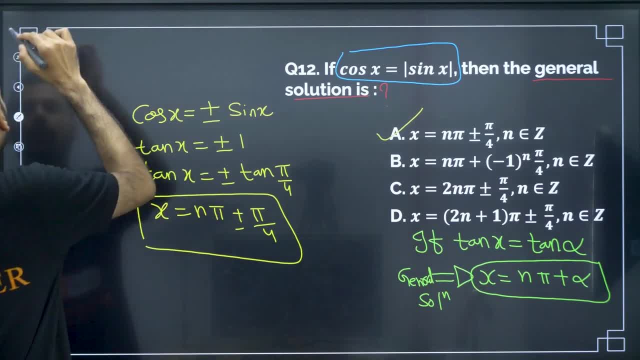 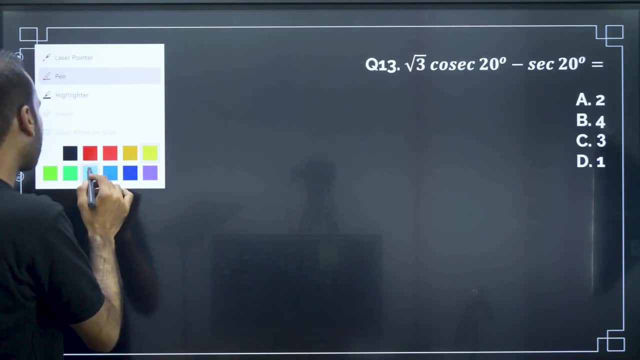 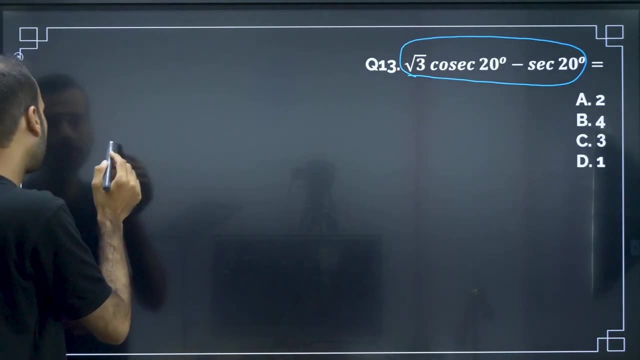 n pi plus or minus pi by 4. a is the answer. moving on to next question: root 3, root 3, cosecant 20 minus. they are asking one expression they have given and they are asking to find its value. now, here, how to approach this problem. the moment you see this, the moment you, 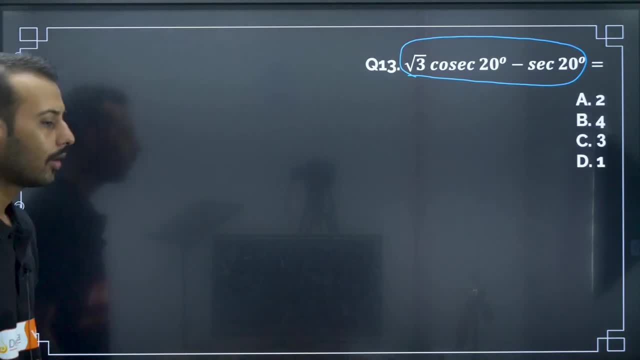 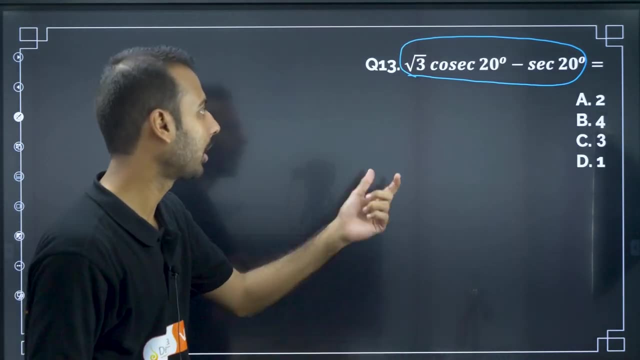 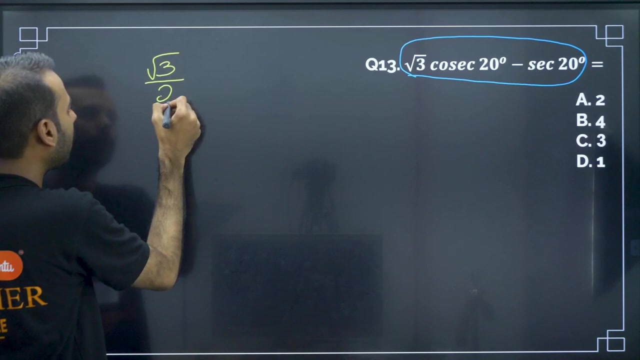 see this expression: cos 20 degree, cosecant 20 degrees, secant 20 degree. they are not standard angles. so one way is to find that cosecant 20, secant 20, all those, or else. or else we can go for algebraic manipulation. root 3: let me write by 2 here. let me write 2 here: cosecant 20, cosecant. 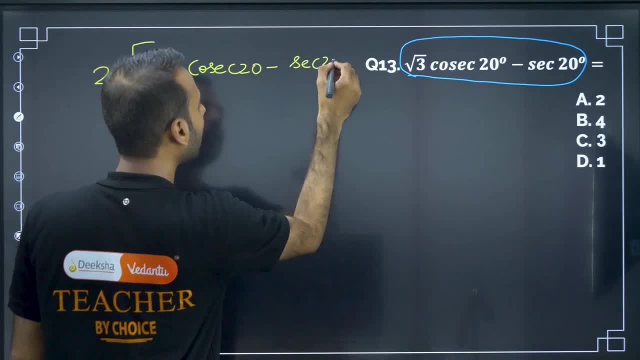 20 cosecant 2 cosecant 3. cosecant 4. cosecant 5. cosecant 5. cosecant 10. cosecant 10. cosecant secant 20 minus secant 20. let me write here by 2 what I did in this step. I have multiplied and. 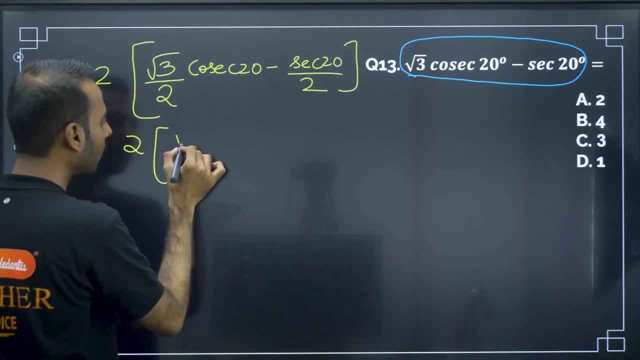 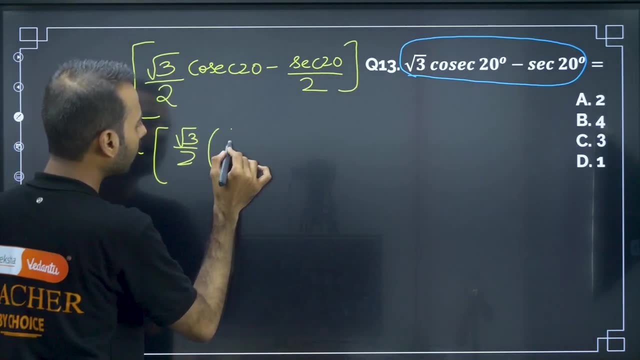 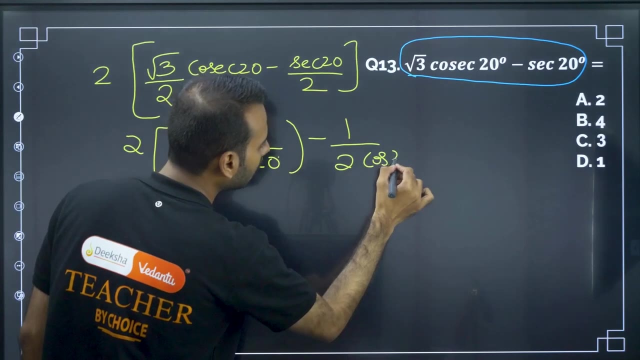 divided by 2.. So let me write 2 here, as it is root 3 by 2, root 3 by 2. let me write root 3 by 2 only for this cosecant: 1 by sin 20. 1 by sin 20 minus 1 by 2. 1 by 2 cos: 20 degrees. 1 by 2 cos. 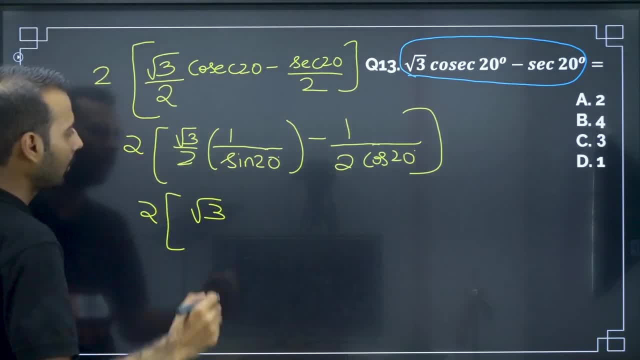 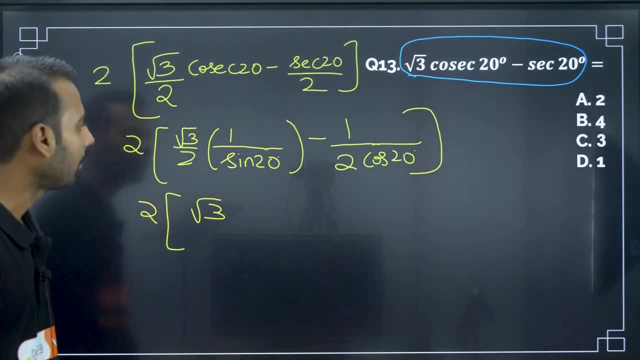 20 degrees. So 2 root 3 root 3 root 3 by 2 sin 20 minus 2 root 3 by 2 sin 20 degrees. cosecant can be written as 1 by sin, secant can be written as 1 by cos. So that one I have done Now. 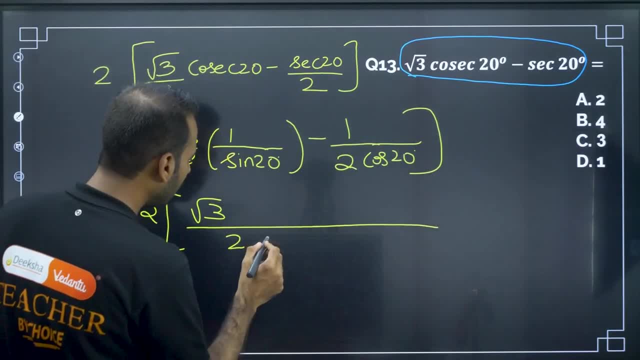 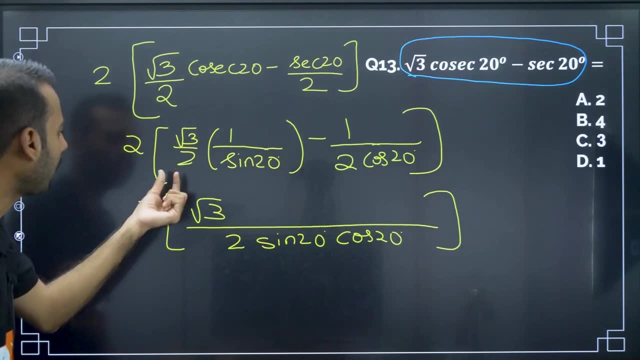 if I take LCM, if I take LCM here, I will get 2 sin 20 degrees, 2 sin, 20 degrees, cos, 20 degrees. What I have written. if I take LCM- 2 sin 20 degrees, 2 cos- I will get this as here I have. 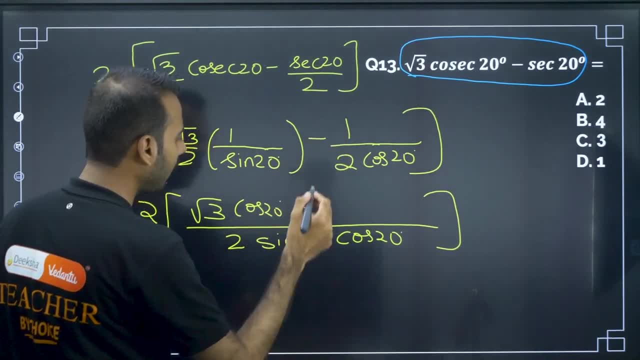 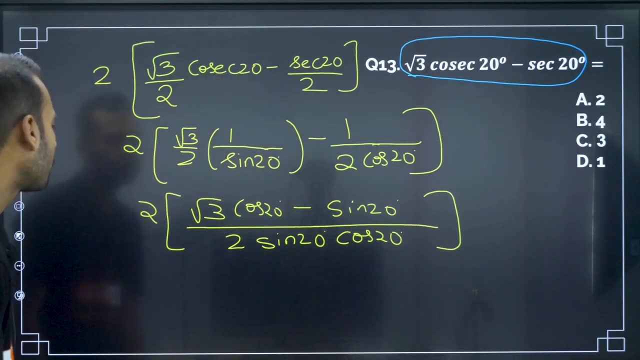 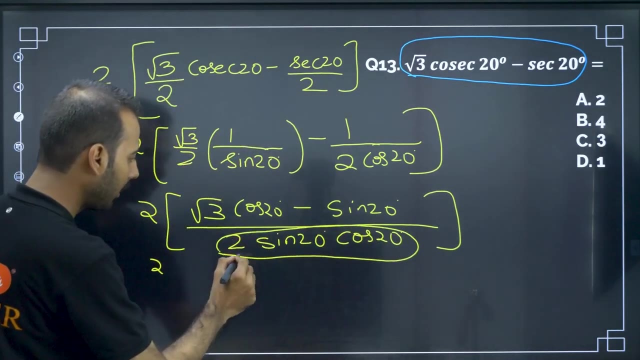 to multiply with cos 20 degrees, cos 20 degrees, and here here I have to multiply with sin 20 degrees, sin 20 degrees. So 2, now 2. let me write this 2 as it is. this becomes sin 40 degrees, sin 40 degrees. 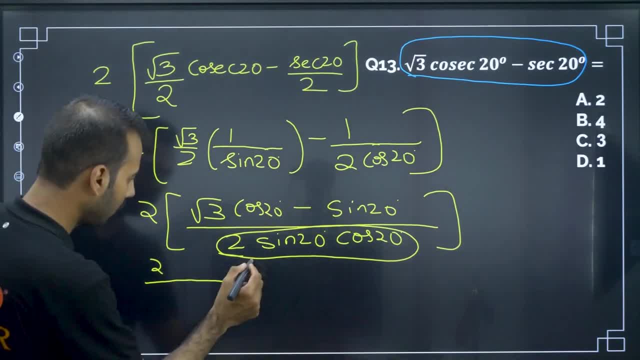 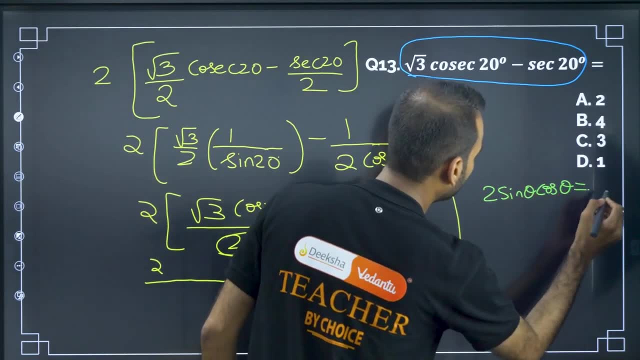 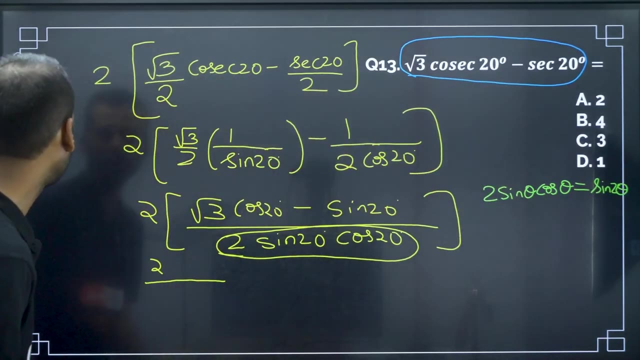 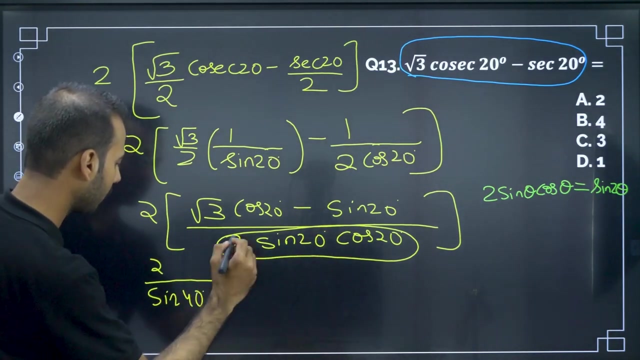 Now try to recall 1 synopsis, point 2: sin theta, 2 sin theta cos theta is equal to 2 sin theta cos theta is equal to sin 2 theta, sin 2 theta. So this becomes to sin theta cos theta is equal to sin 40 degrees sin 40.. Now here in the bracket, what are we left? TP 3 cos. 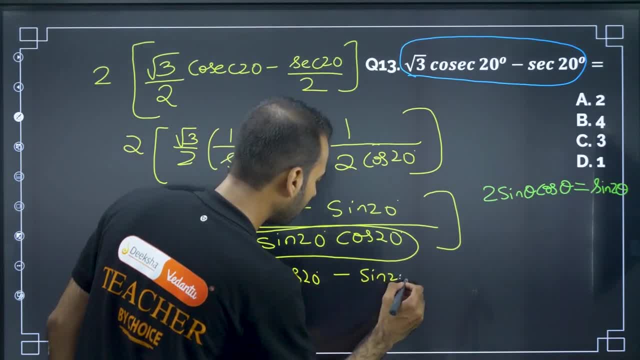 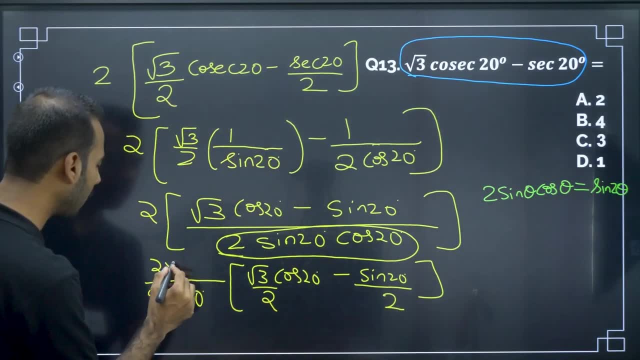 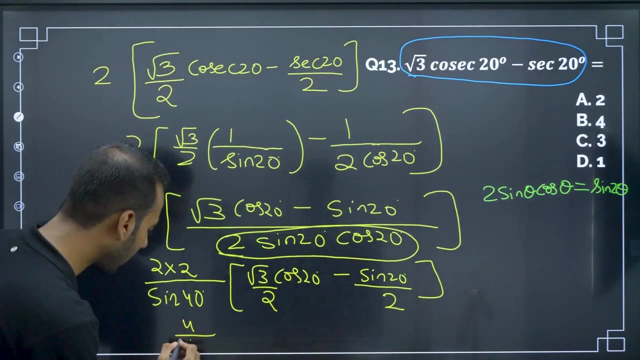 3, cos 20 minus sin 20, sin 20. this many things are there. Let me go again for divide by 2. divide by 2 and then multiply by 2.. So the equation also remains balanced and everything is fine Now. 2: this becomes 4 by sin, 40 by sin 40, 4 by sin 40. root 3 by 2 in place of root 3 by 2. 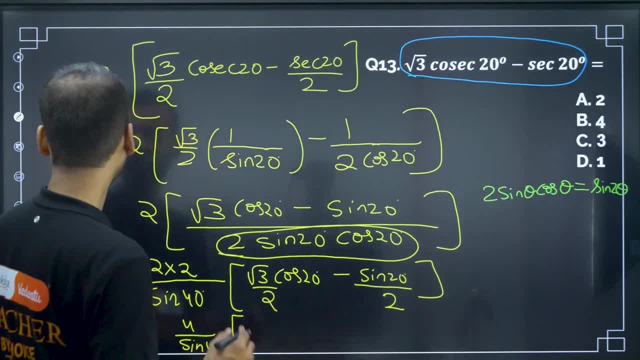 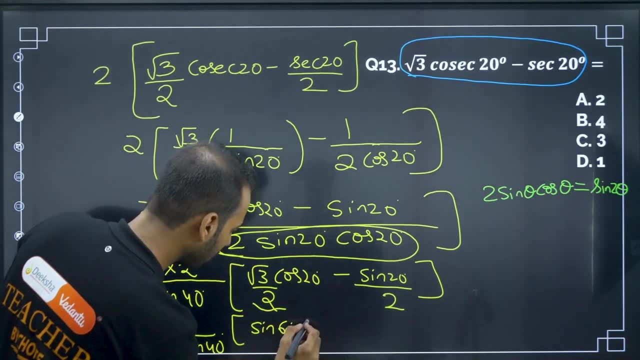 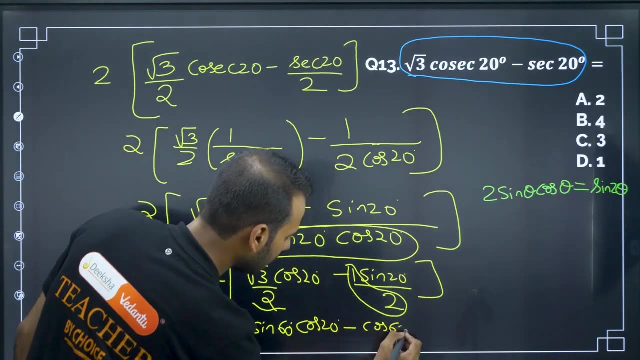 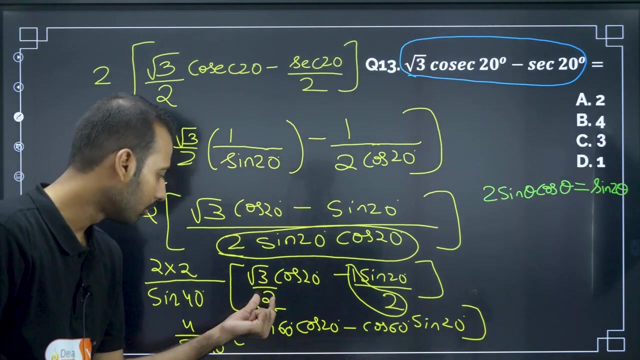 can I write this as in place of root 3 by 2, I will replace it with sin 60 degrees, cos 20 degrees. in place of 1 by 2, I will write this as: cos 60 degrees, sin 20 degrees. See here root 3 by 2. in place of root 3 by 2, I am writing sin 60 in place of 1 by 2. I am writing: 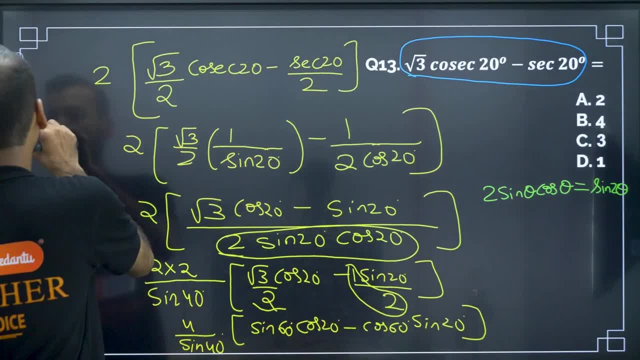 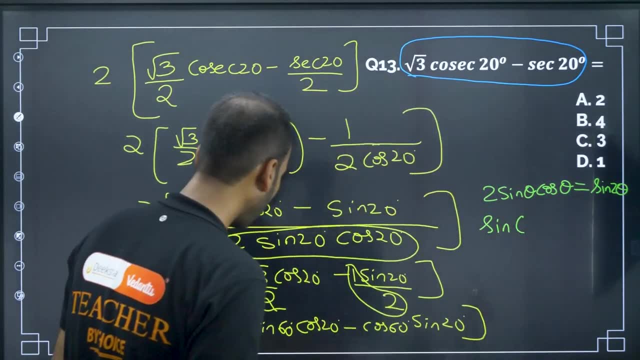 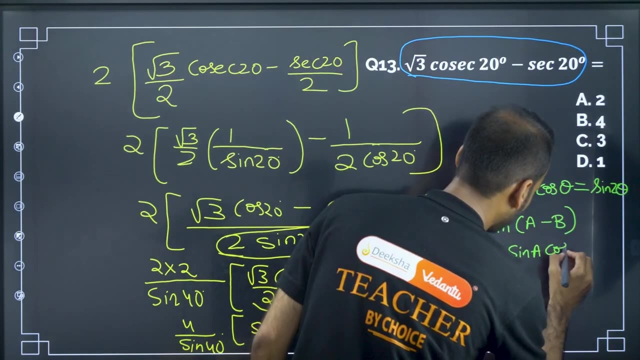 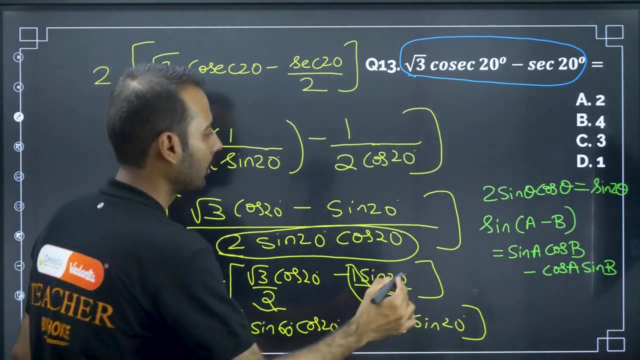 cos 60.. Now one point. you try to recall one synopsis point. what is that synopsis point? at this point you should be knowing sin of sin of a minus b- a minus b is equal to sin a cos b minus cos a sin b. So one synopsis. this is first synopsis point. this is second synopsis point. sin a minus b is equal to. 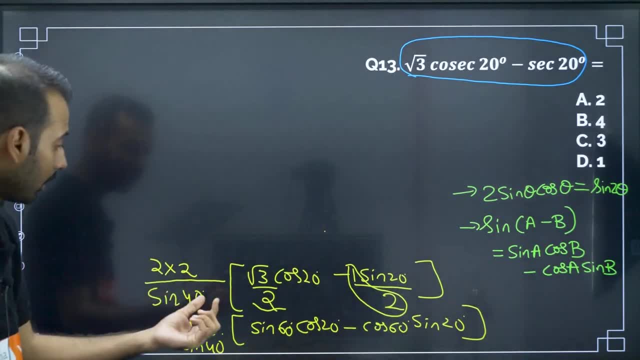 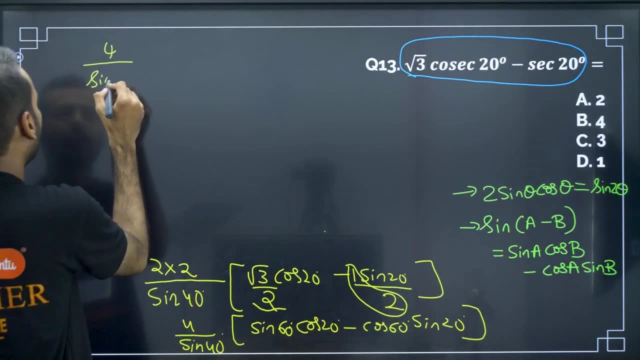 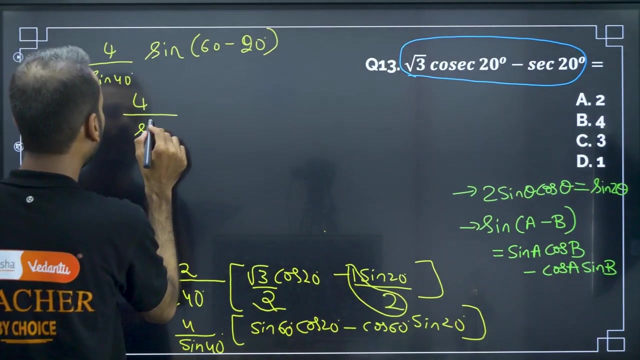 sin a cos b minus cos a sin b. Now let me remove some things: sin a minus b. Now if you see here sin a, cos b minus cos a sin b. for that, this 4 I am writing as it is sin 40. I am writing sin 40. I am writing as it is sin of sin of a minus b, 60 minus 20, 60 minus 20. next, 4 sin 40. 4 sin 40 and this is also sin 40. 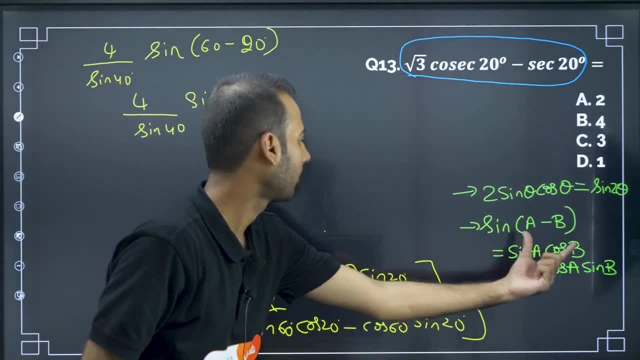 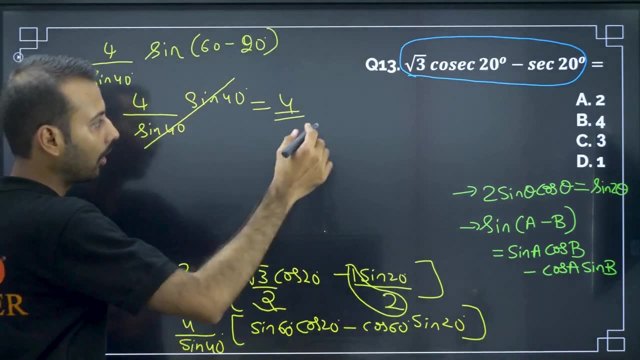 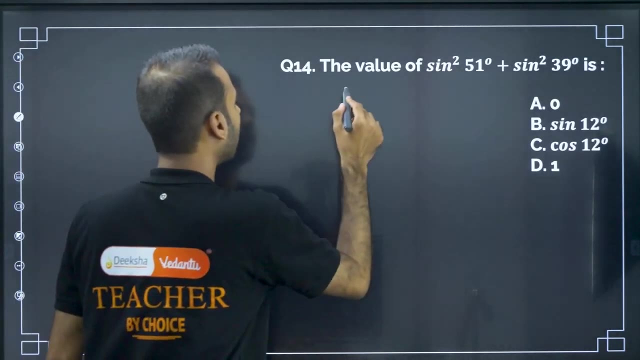 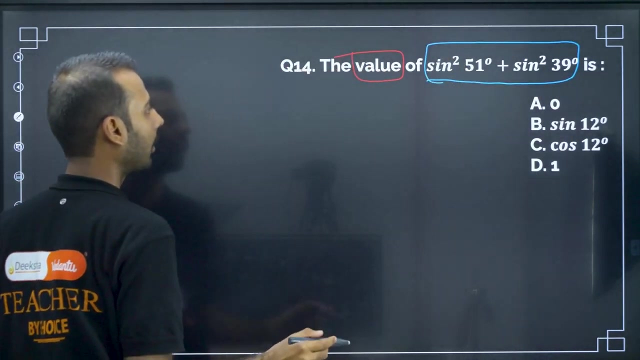 See here this: sin 60.. I am using this formula synopsis point. So here I have written: sin 40, sin 40 cancelled and finally we are left with 4.. So what are we left with? the answer is 4. moving on to next question: the value of what are they asking? the value of one expression they have given. what is that expression? sin square 51 plus sin square 39 is the value of sin square. 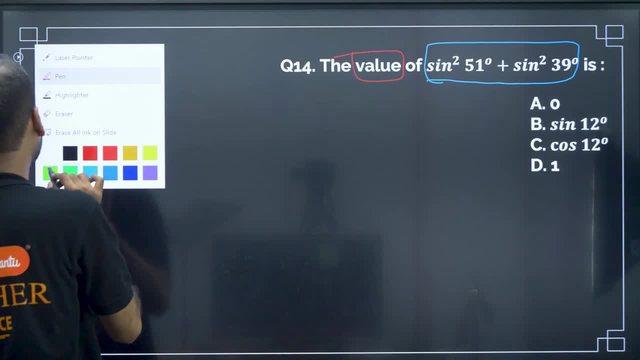 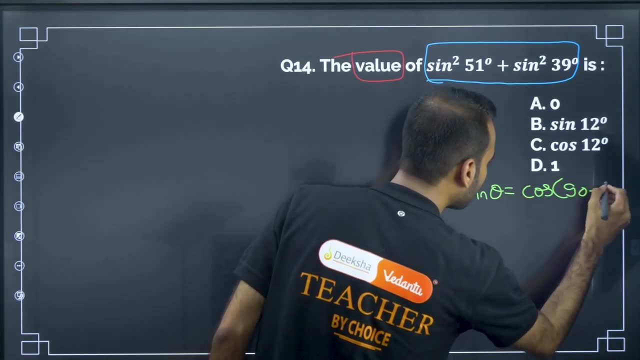 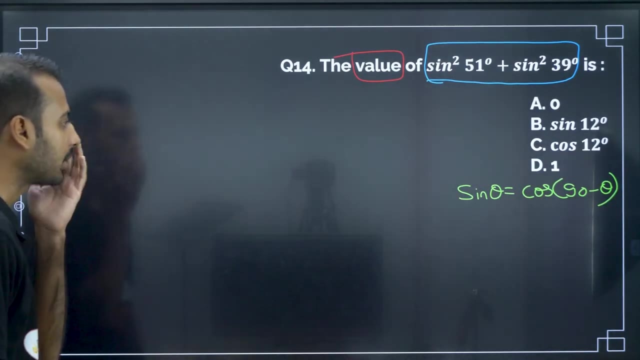 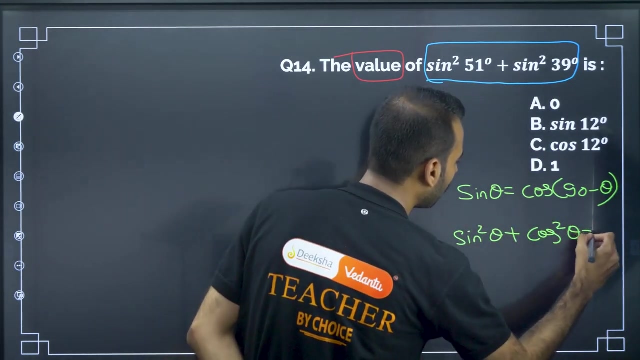 Now for to solve this problem, you should know some basic identity. So, for example, if you know the identities of trigonometry, what is that? sin theta can be written as cos of 90 minus theta. sin theta can be written as cos of 90 minus theta. sin theta can be written as cos of 90 minus theta. sin theta is equal to cos 90 minus theta. and one more identity. you should be knowing what is that sin square theta plus cos square theta is equal to 1.. 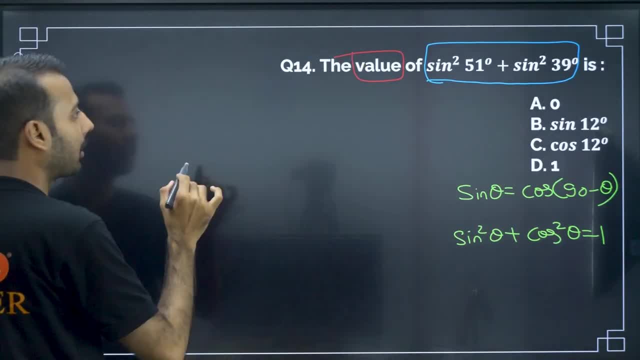 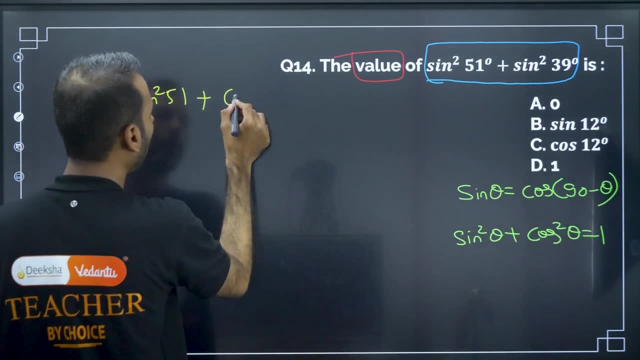 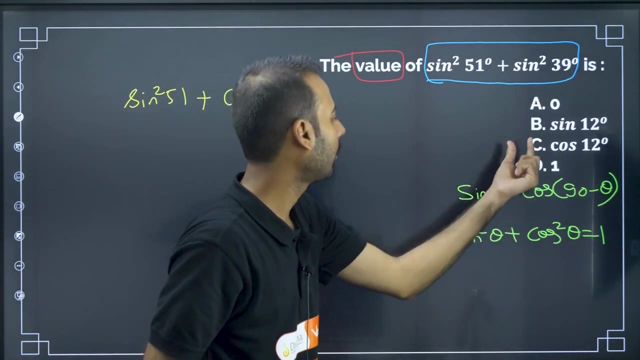 If you know this identities, you can Solve this problem within second. So first let me write sin square 51 as it is plus sin 39 can be written as cos of 90 minus 31.. So sin sin theta can be written as cos of 90 minus theta. 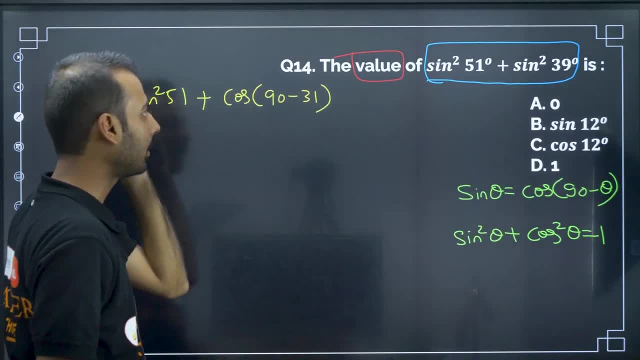 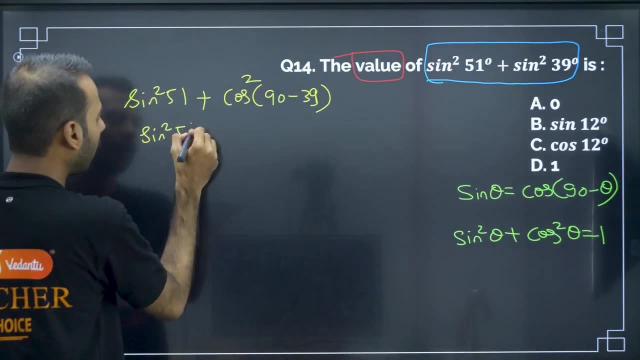 So for that I am writing: cos of 90 minus 90 minus theta is 39.. I am writing it like this square is there, So I am placing square. This becomes a sin square 51 plus cos square. So sin square 51 plus cos square 51, its value is equal to 1.. 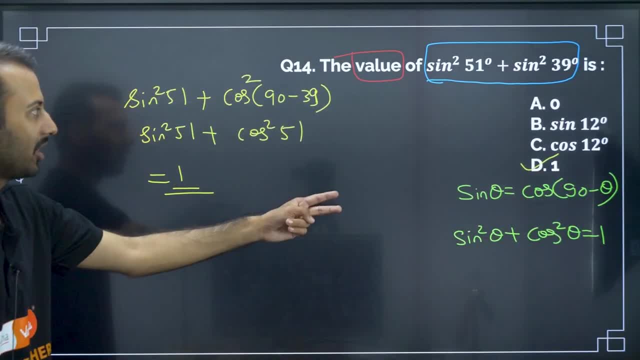 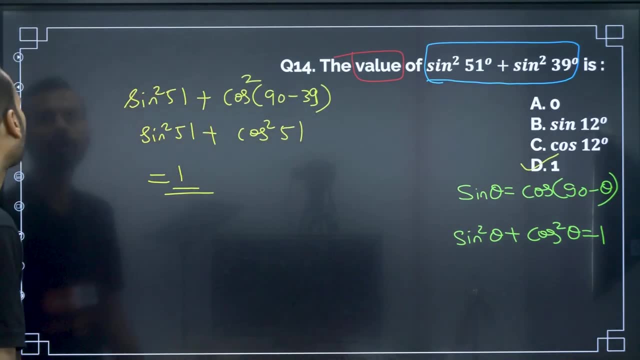 So is there any such option? Yes, d is the answer. So here, basic two points you should be knowing and you have to solve this So hardly it will take 20 seconds to solve this. So moving on to next question. 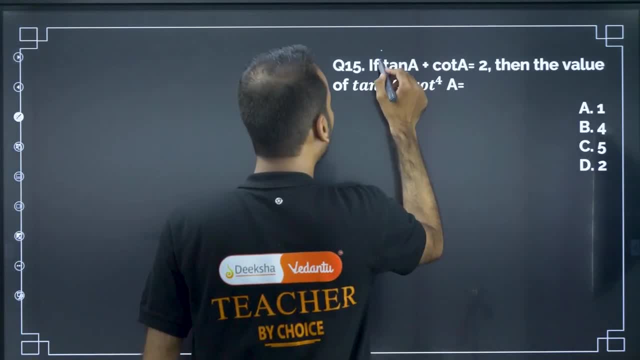 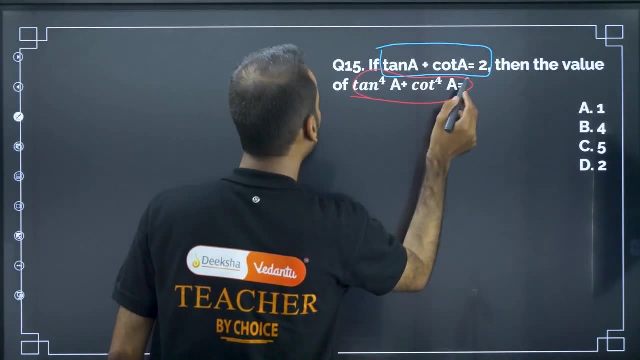 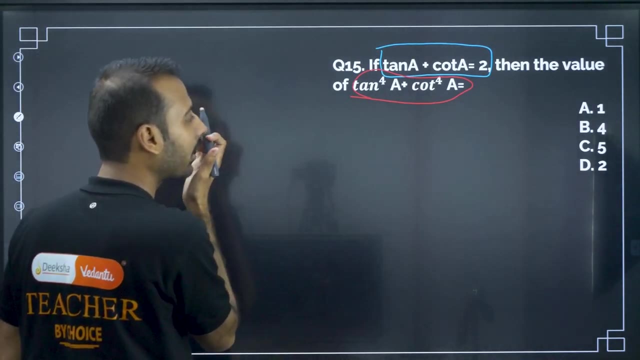 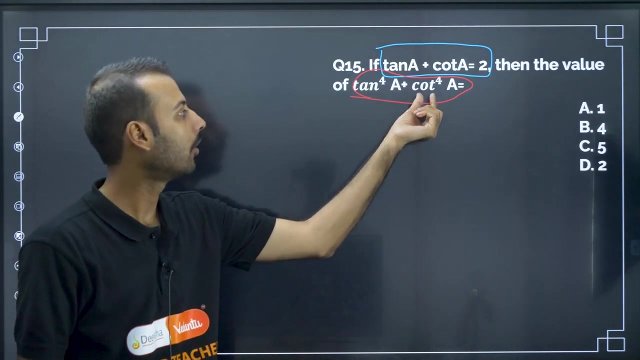 If tan a plus some value they have given, if tan a plus cot a is equal to 2, then then what are they asking? They are asking to find this. They are asking to find this: If tan a plus cot a is equal to something they have given, tan a plus cot a is equal to 2, then the value of what are they asking? they are asking to find a value of this. 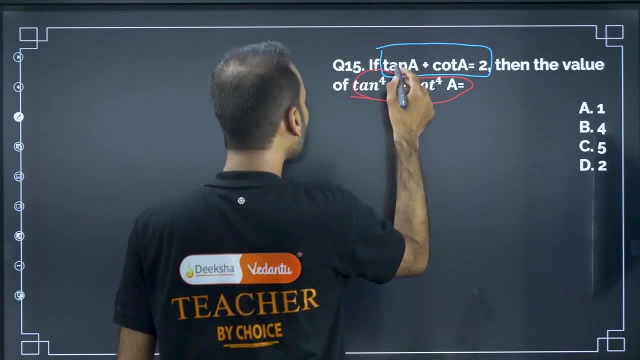 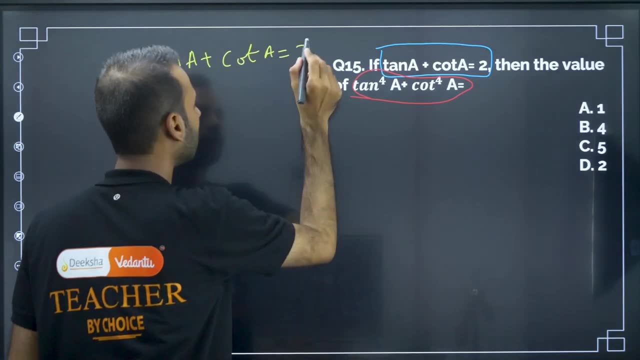 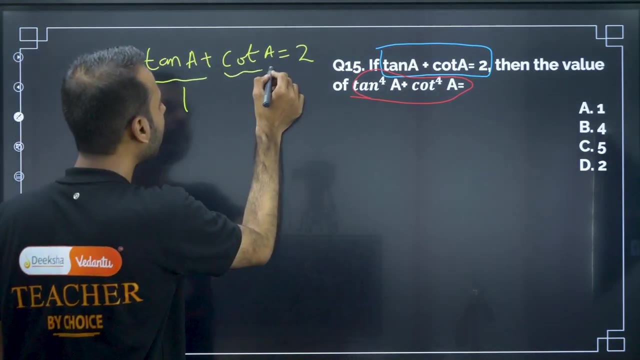 So tan a plus cot a is 2. tan a plus cot a is equal to 2, is equal to 2. they are asking tan 4 a plus cot 4 a. Now let me say this as This as 1 and this as 1, tan a as 1 and cot a as 1.. 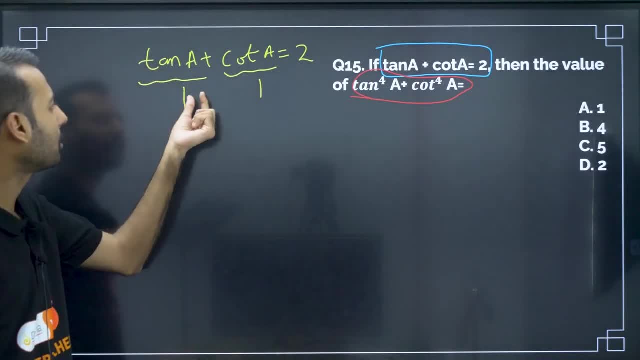 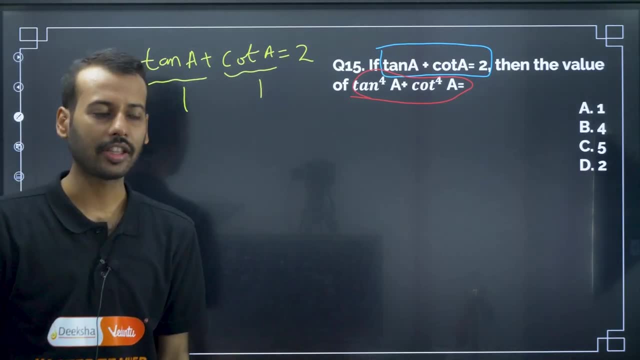 Now some student. they will put objection, Sir, why you are saying tan a is 1, it can be 0.5, and this can be 1.5, it can be 0, it can be 2, yes, it can be anything. but here, dear, if I write tan a as 1, cot a as 1, I am not doing anything wrong. 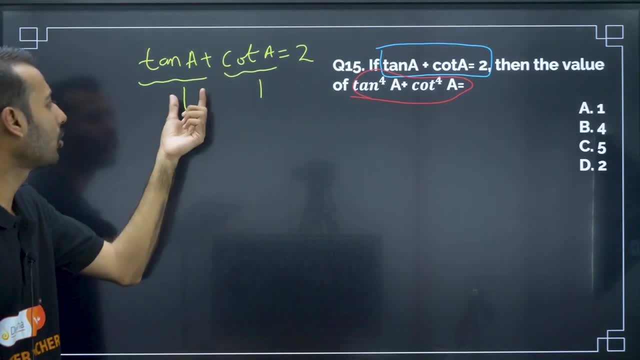 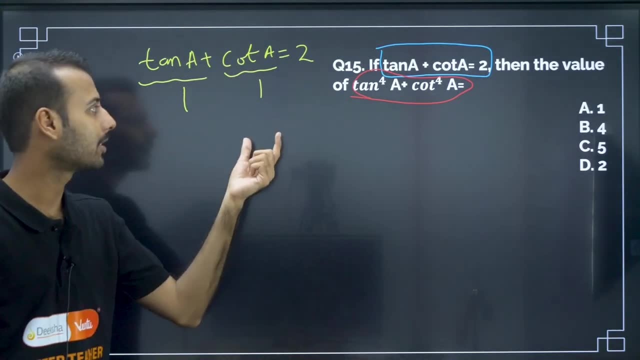 I am seeing this quantity might be 1, this quantity might be 1, it can be 0.5 and it can be anything, but I will assume. I will assume that tan a is 1, cot a is 1. And there is nothing wrong in my assumption. so it is ok if you do like this, or else, if you want to go for normal method, also, you can go for normal method. it will take lot of time. 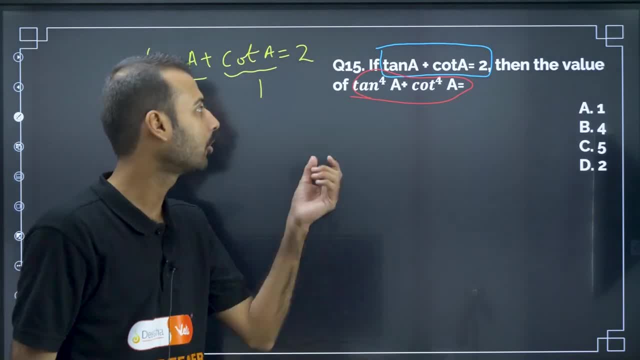 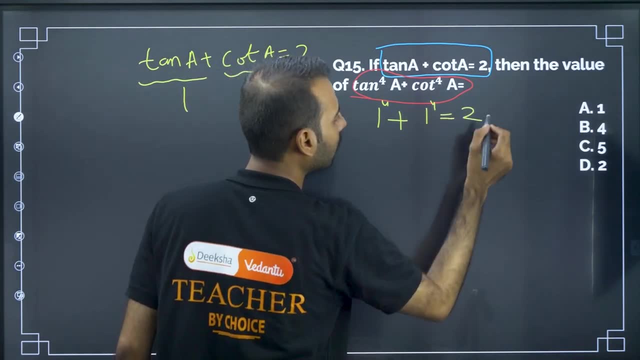 So in competitive, normal method it will work, but it will time consuming. to save time, we have to go for some shortcut. So let me write this as 1: 1 power 4. 1 power 4. this is equal to 2. is there any such option like 2? d is the answer. 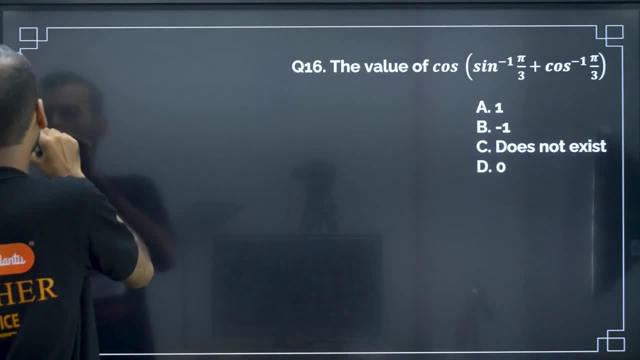 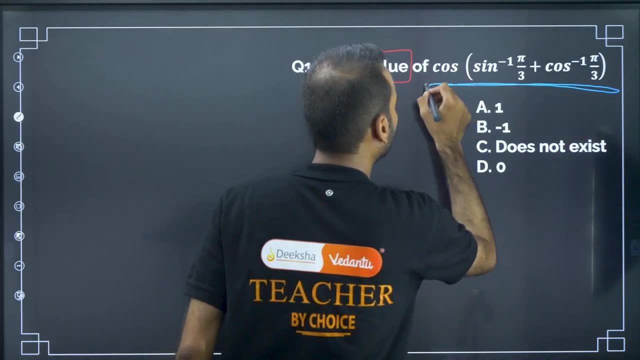 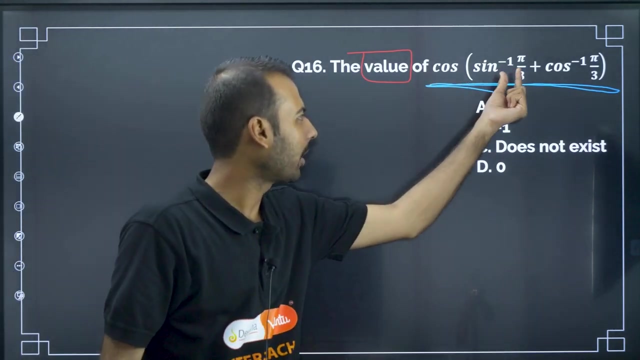 Moving on to next question, the value of next question, the value of one expression they have given. What is? What is that expression? if you go through cos of this, cos of this is now go see this cos of sin inverse, pi by 3 plus sin cos inverse. the moment you see this, you should say: answer does not exist. 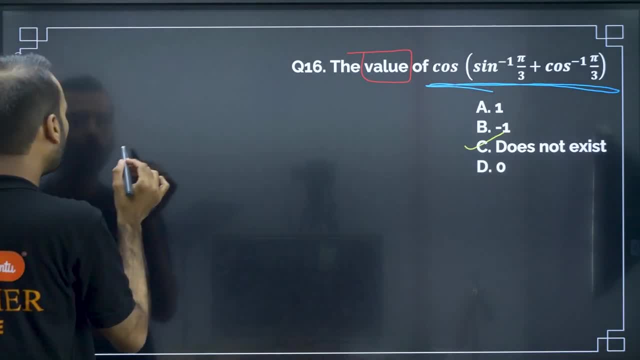 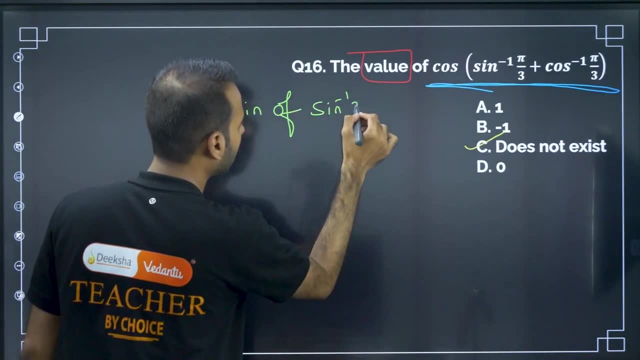 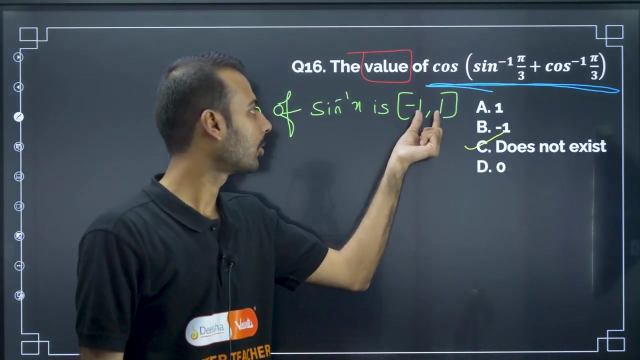 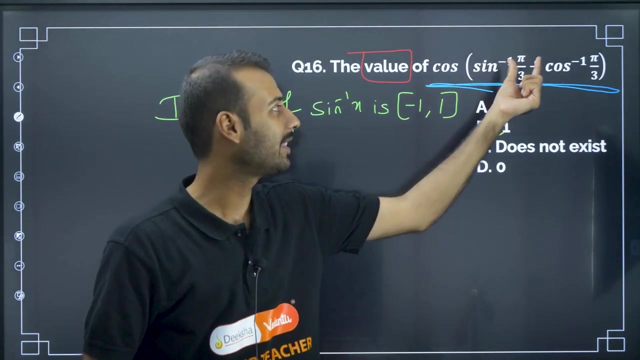 Why? answer does not exist. because domain of domain of sin inverse. sin inverse x is minus 1 to 1.. But for here, sin inverse, they are giving pi by 3 as domain to sin inverse. pi is 3.1. 4 by 3 means it will be more than 1. for sin inverse they are giving more than 1. that will not accept. 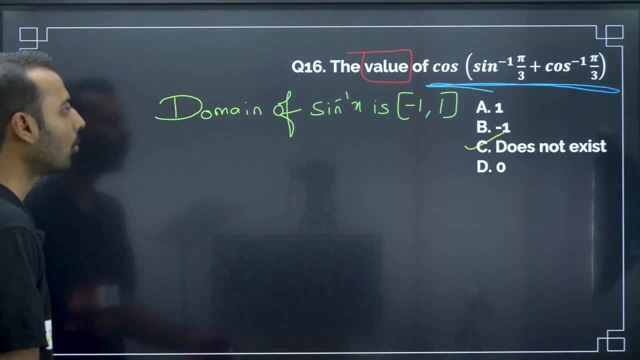 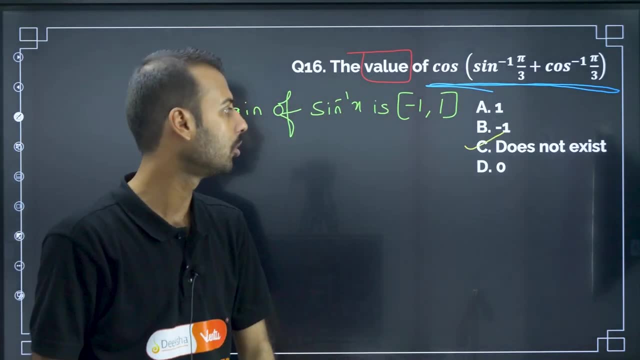 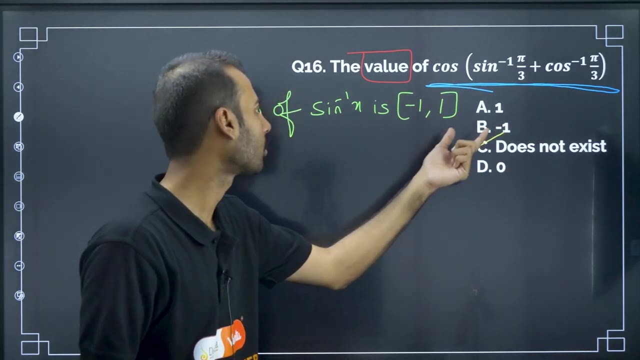 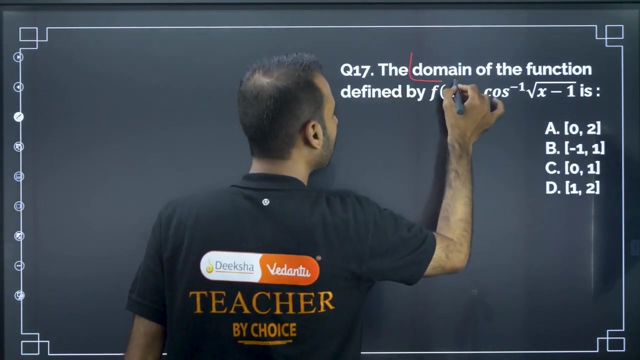 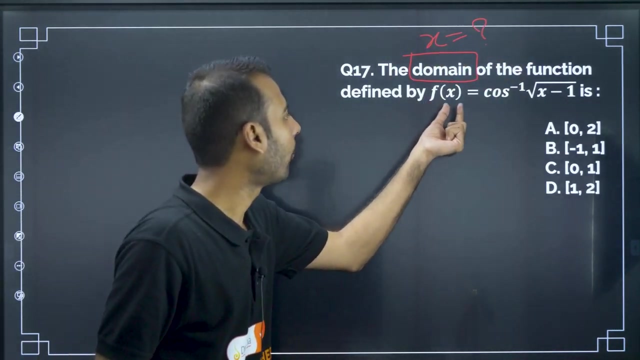 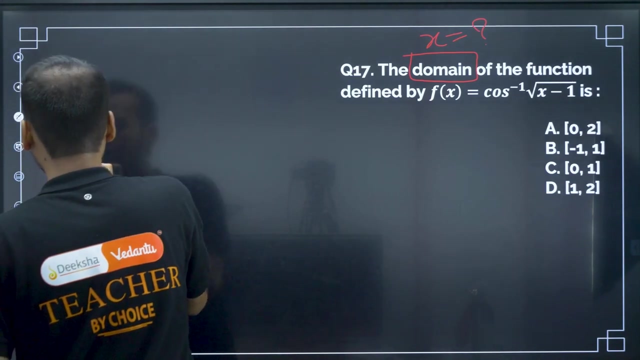 So does not exist, is the answer only see here, if you know this point. so that is why I said domain and range of all 6 trigonometric functions you should know for solving problems related to. So if you know, only Hardly it will take time to tick 1 second or 2 seconds. so do not leave inverse trigonometry. moving on to next question: the domain of what is the question? domain domain means what x values they are interested in. x of the function defined by f of x is equal to 1 function. they have given 1 function. what is that function? cos, inverse of root, all those things they have given. now let me highlight that. 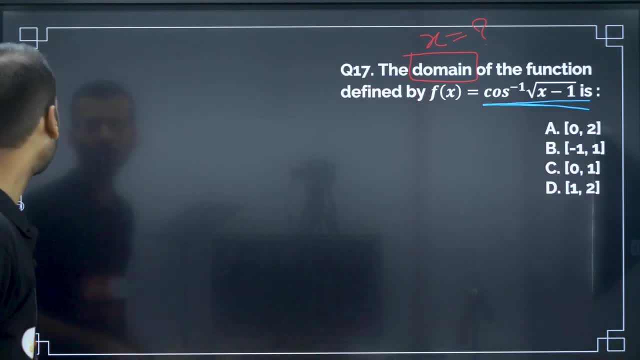 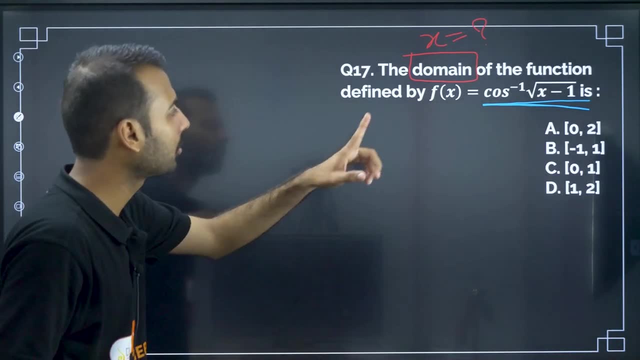 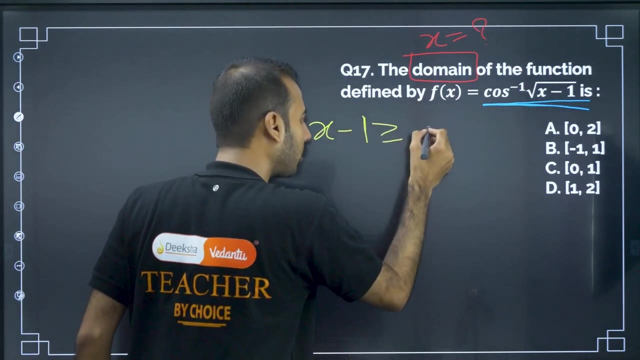 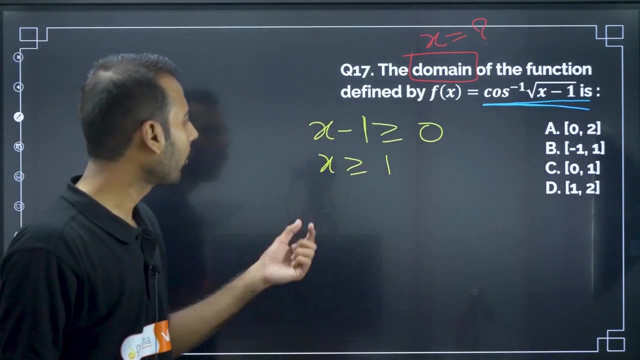 This is the function. Now they are asking domain. every time I say in my previous videos also: the moment you see square root, what? the moment you see square root, that whatever is that inside that square root? inside that square root that has to be greater than or equal to 0, that has to be greater than, which implies x is greater than or equal to 1. x is greater than or equal to 1. now, if you go through the options, x is greater than or equal to 1. there is only one option. d is the only one option. so answer for this is d. 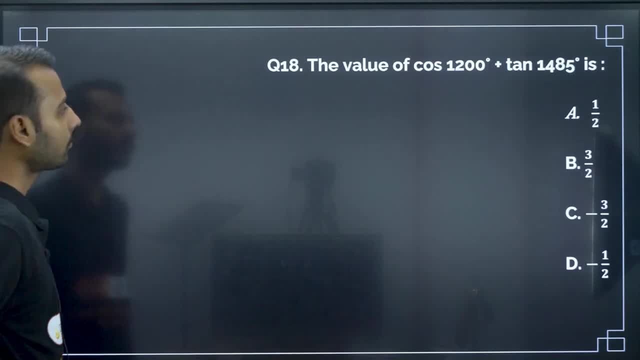 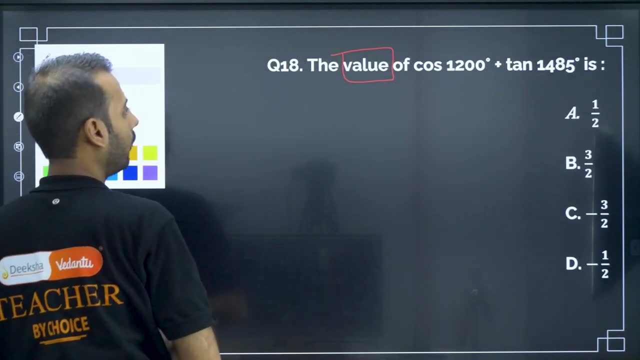 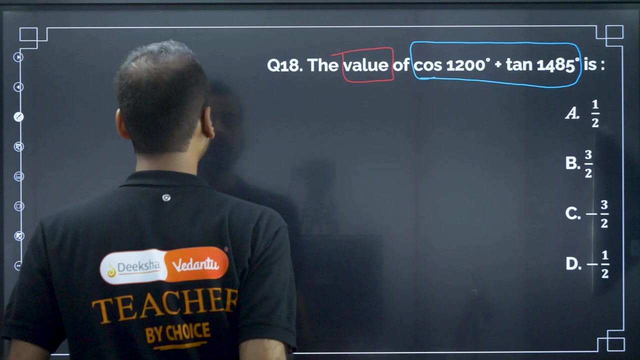 Moving on to next question, The value of. again, they are interested in the value of the value. of course, the value of course This one is what they're asking: to find its value. so let me copy and paste that expression here: course to well and read. course to well and read, plus 10 off 1485, 1485, 1485.. 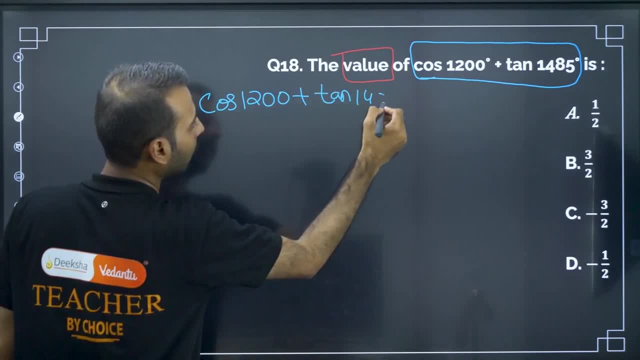 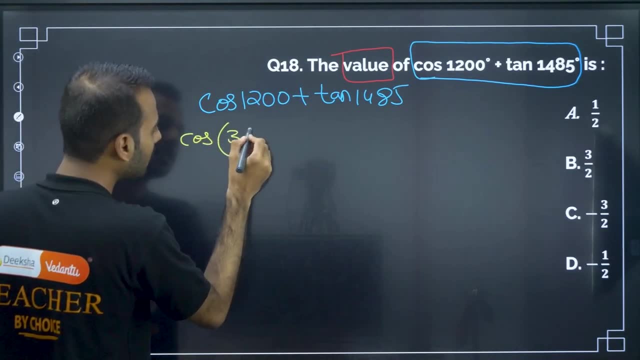 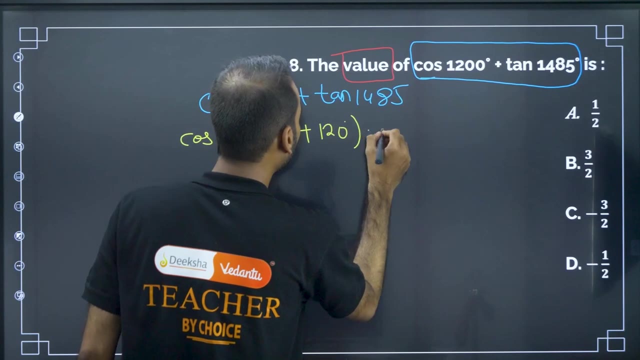 So let me copy and paste that expression here: cost 200.. cost 200 plus 10 off 1485, 1485, 1485.. Now for this let me write: cos of 360 into 360, into 3 plus 120,. for this let me write: 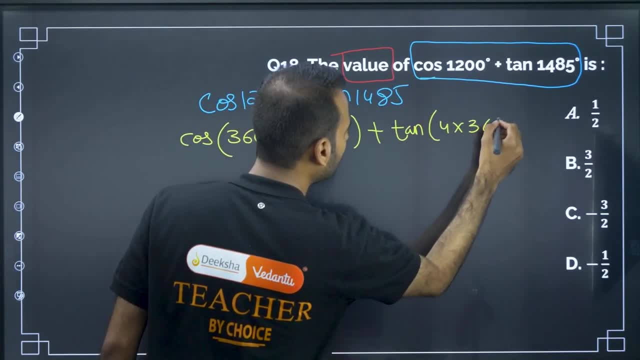 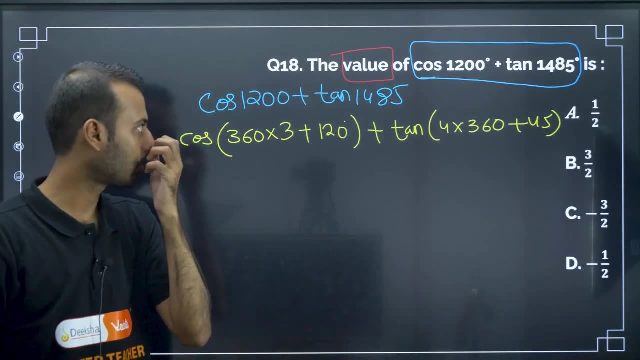 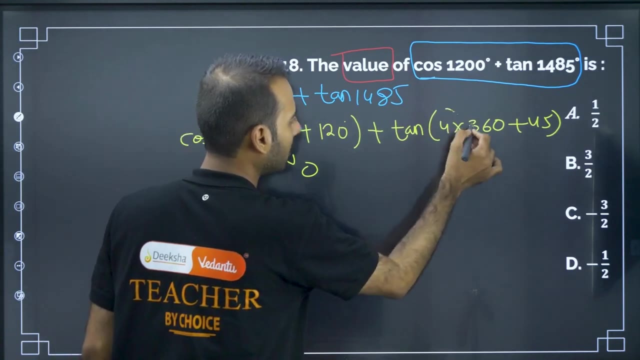 tan of 4 into 360 plus 40. pi 36, 3 is a 1, 0, 8, 0 plus 2, 1, 20 and 1, 4, 4, 0 plus 45. So, anyways, this is 0,. anyways, this is 0,. so here we are left with cos of 120 and here 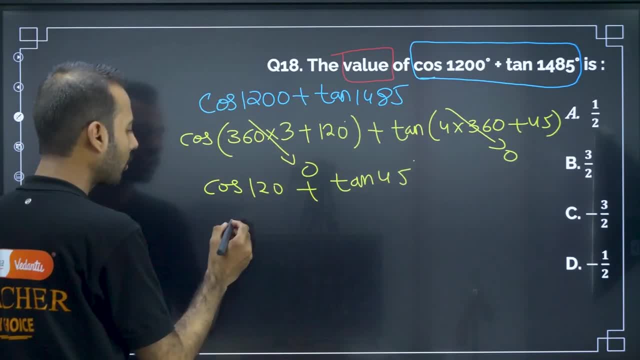 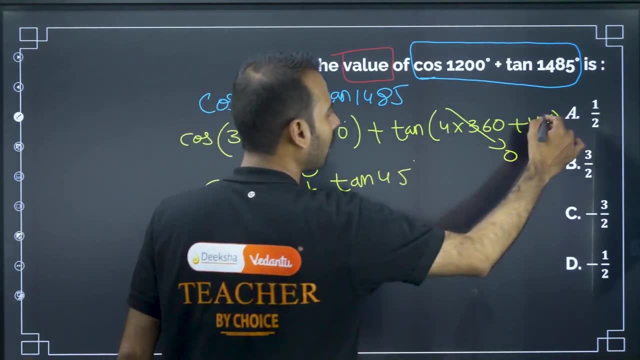 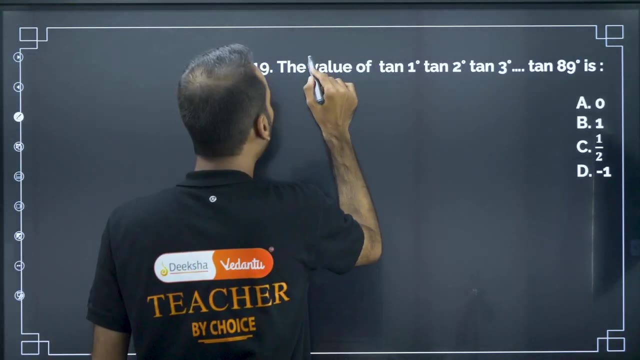 we are left with tan of 45, cos 120 is minus 1 by 2 and tan 45 is 1, so 1 minus 1 by 2 is 1 by 2 is the answer. Moving on to next question, the value of what are they asking. they are asking to find value. 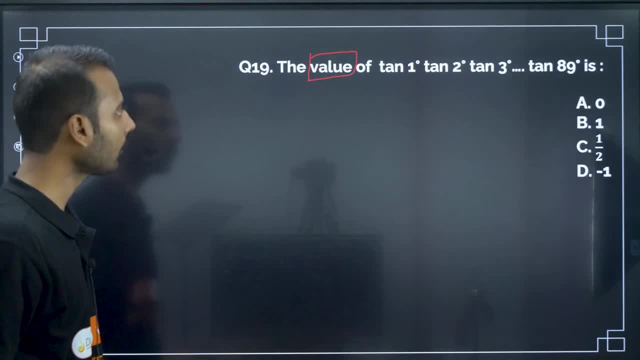 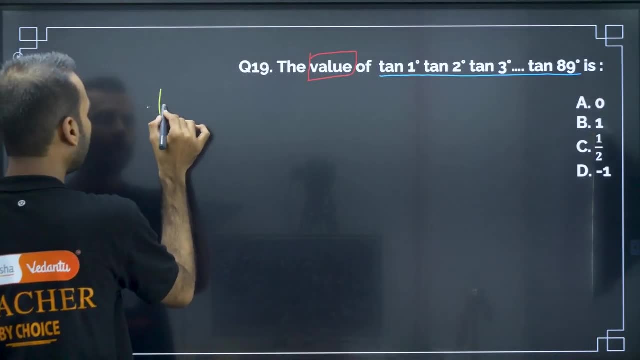 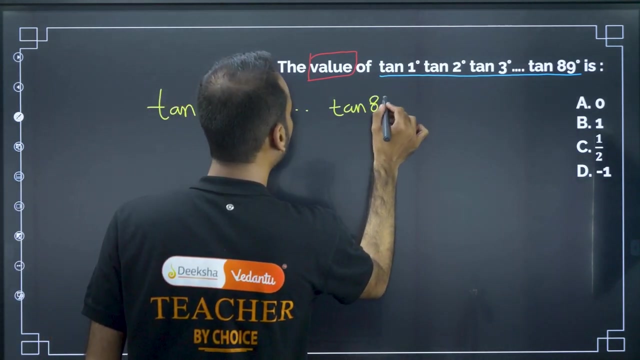 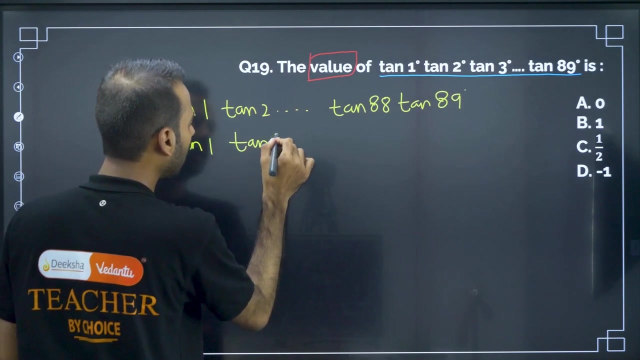 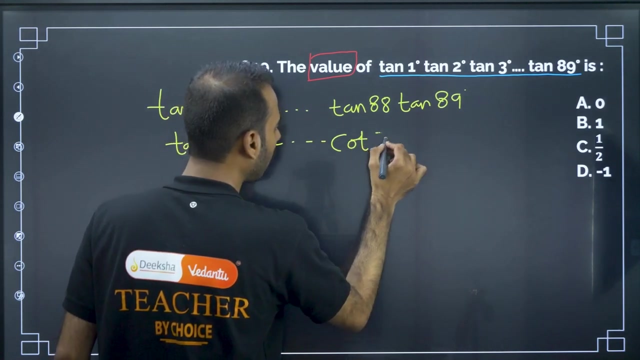 of some expression. they have given The value of tan 1. this now, see here let me write that tan 1, tan 2, so on: tan 88, tan 89.. So for this let me write same tan 1, tan 2, tan 2. and for this let me write cot, cot, 2, cot. 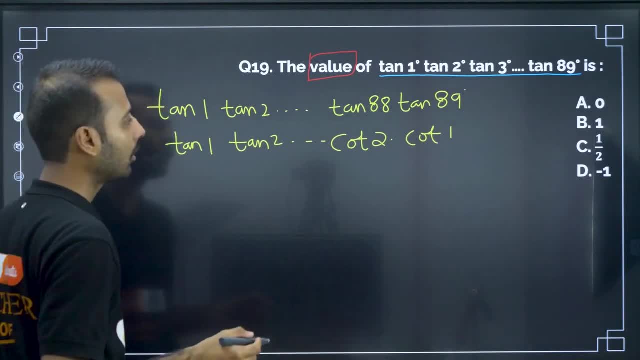 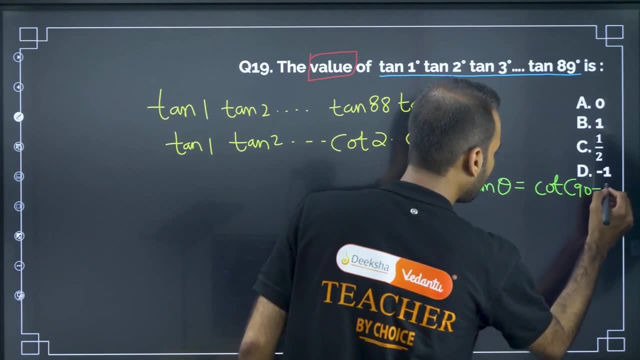 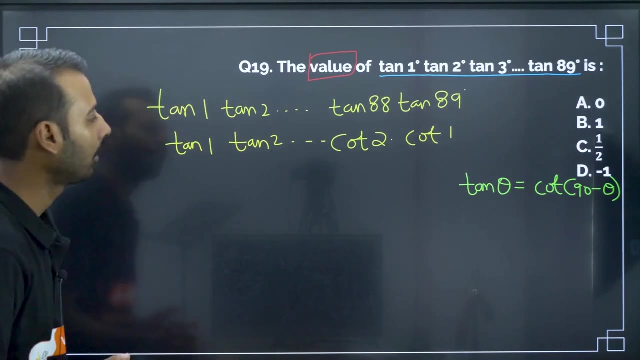 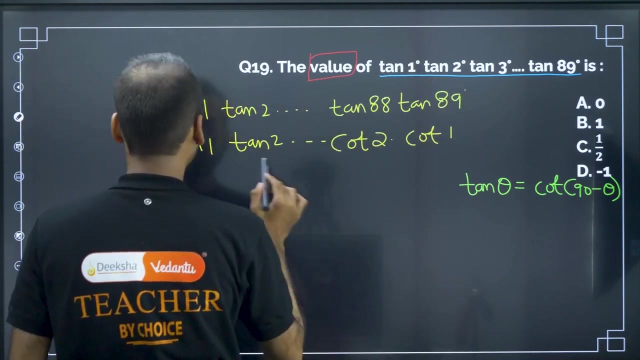 2. Now the reason why I am writing like this: one synopsis point you should be knowing: tan theta can be written as cot of 90 minus theta. tan theta can be written as cot of 90 minus theta. So for this tan theta can be written as now: if here it is tan 88, now tan 88, tan. 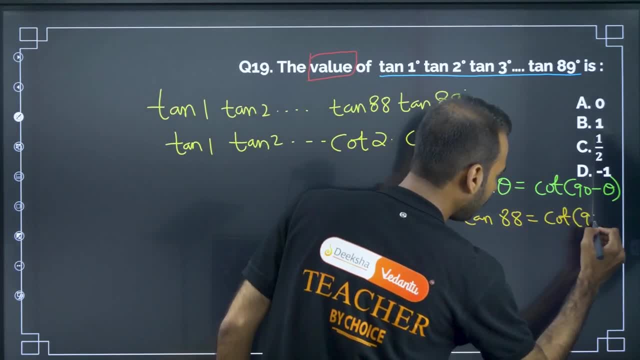 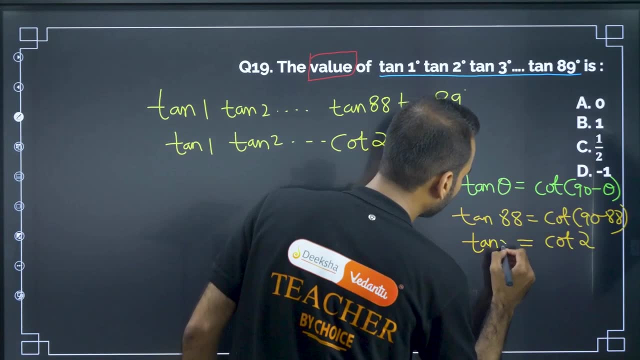 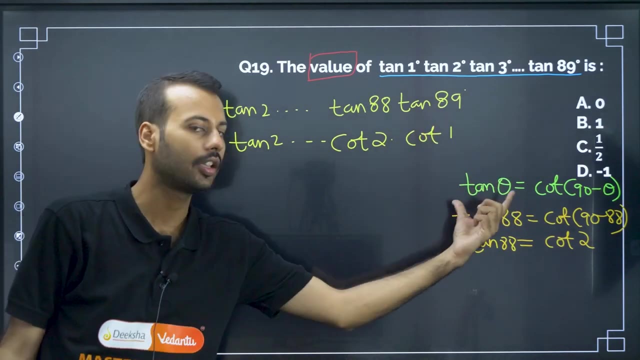 88 can be written as written as cot of 90 minus 88. So this is cot 2. tan 88 is equal to tan 88 is equal to cot 2. tan 88 is cot 2, tan 89 is cot 1 in the same way. here I have shown the mechanism. 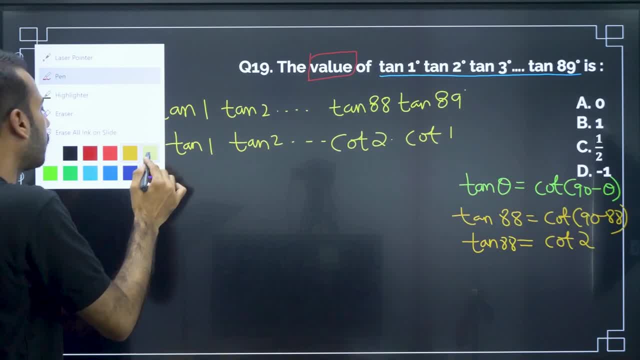 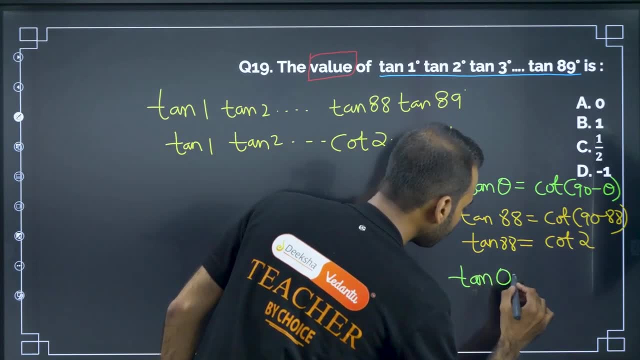 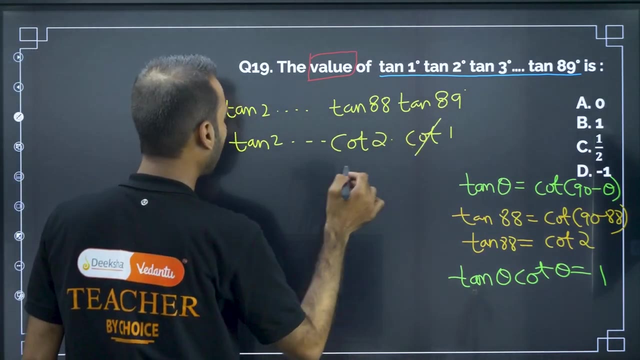 of why I am writing this Now. if you observe this, this goes like this: tan 1 cot 1. again one more synopsis point I want to give tan theta- cot theta. product of tan theta cot theta is 1.. So this becomes tan theta- cot theta 1. tan theta- cot theta 1, 1 multiplied by 1. multiplied by 1. 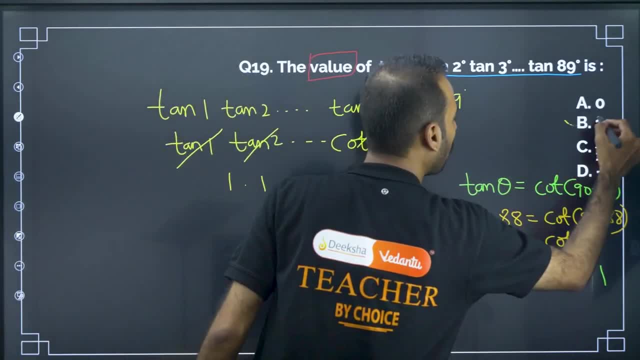 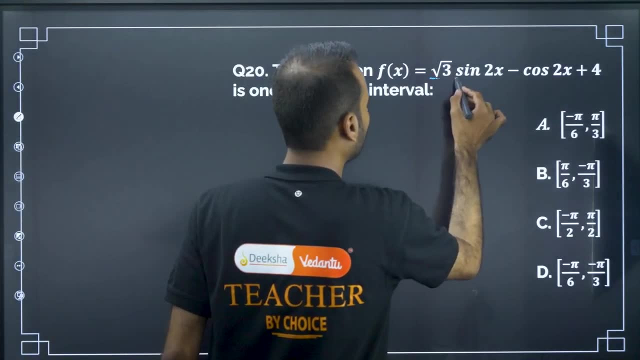 multiplied by 1, so on. So, ultimately, you are going to get 1 as the answer. Moving on to next question, the function. they have given some function. if this function is 1, 1, they are saying that it is 1, 1.. 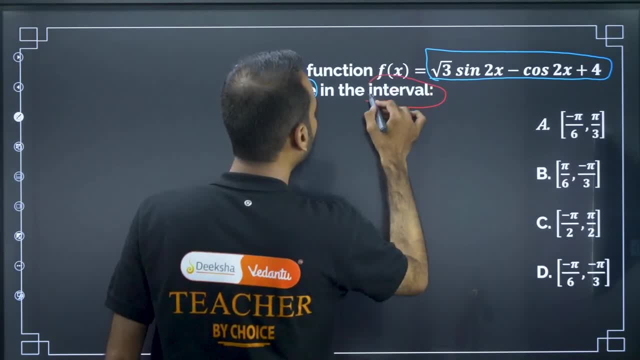 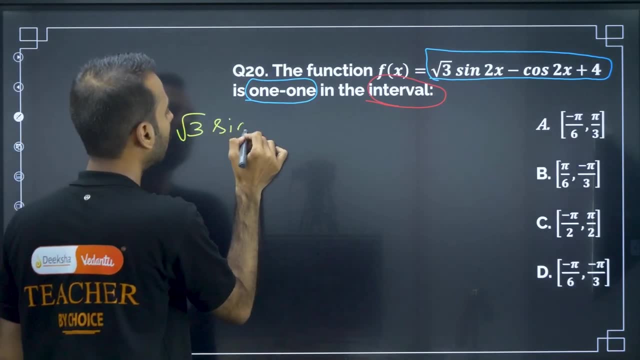 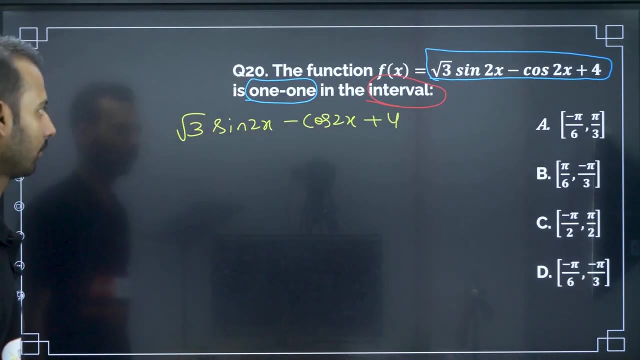 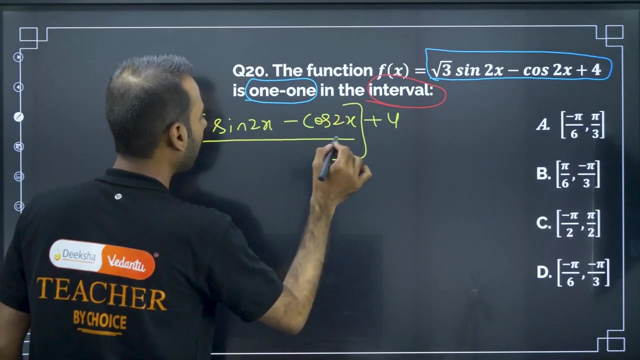 In the interval. what are they asking? in what interval this function is 1, 1? they are asking like this. So let me write that question: root 3: sin 2 x minus cos 2 x, cos 2 x plus 4: root 3.. So for this, let me multiply. let me multiply by 2 and divide by 2.. 2 root 3. 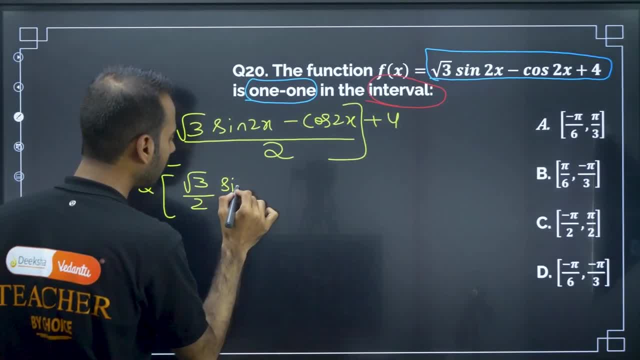 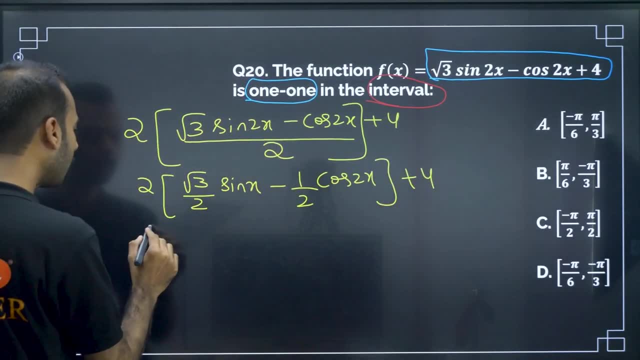 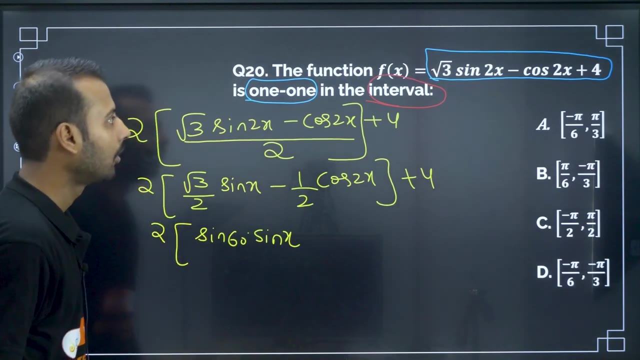 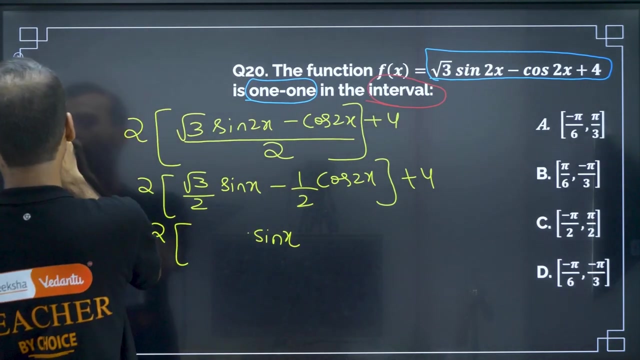 by 2. root 3 by 2.. Sin 2 x minus 1 by 2. cos 2 x plus 4: 2: here let me write sin 60, sin x, rather than writing this as. let me write this as cos 30. root 3 by 2 can be written as cos pi by 6. this can: 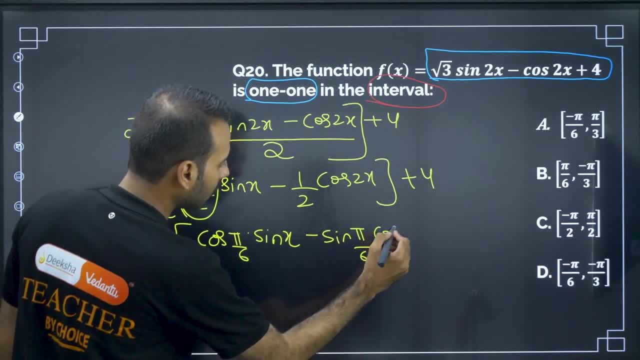 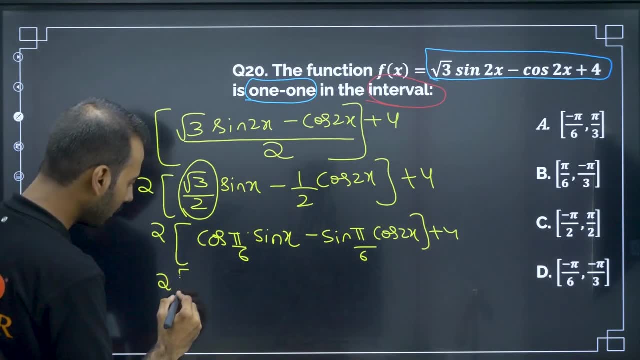 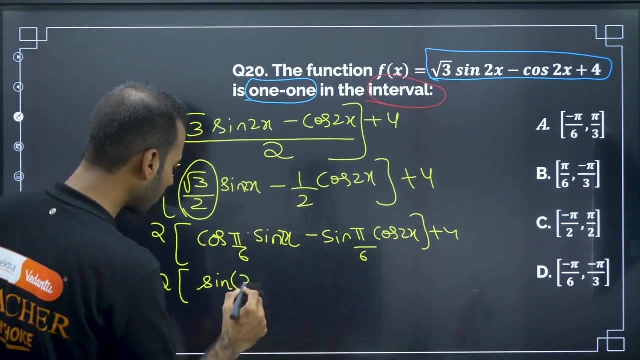 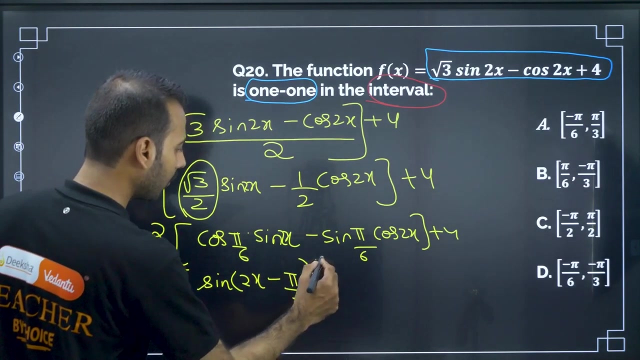 be written as: So: sin pi by 6 cos 2 x plus something. Now here let me write 2 cos pi by 6. this is sin. I think this should be 2 x. this should be 2 x. this becomes 2 x 2 x minus pi by 6 plus. 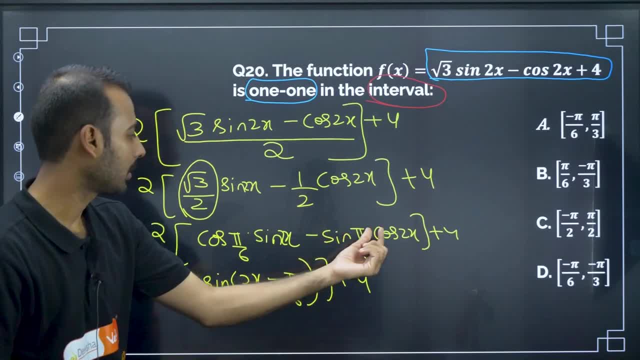 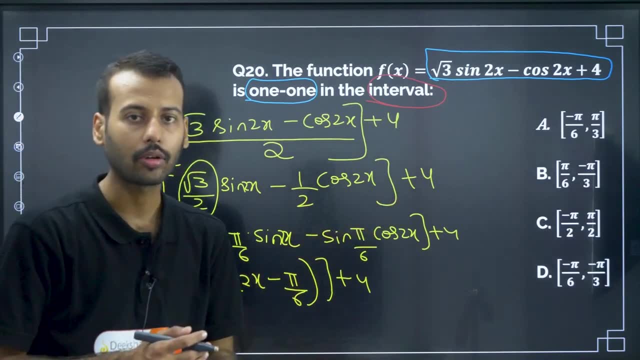 4, as it is sin a cos b minus cos a sin b. So this: So sin a minus b. just I am saying, I am not writing. try to recall the synopsis point. sin a minus b is equal to sin a cos b minus cos a sin b. So whenever it is sin a cos b minus, 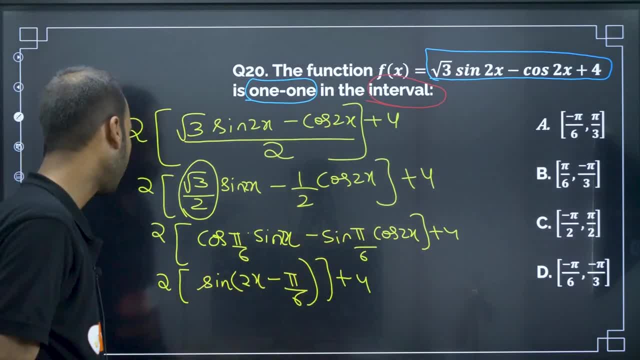 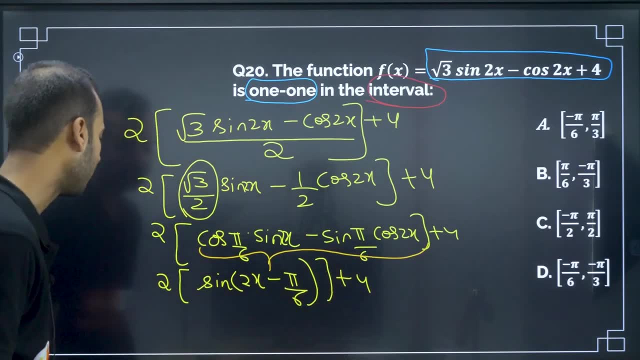 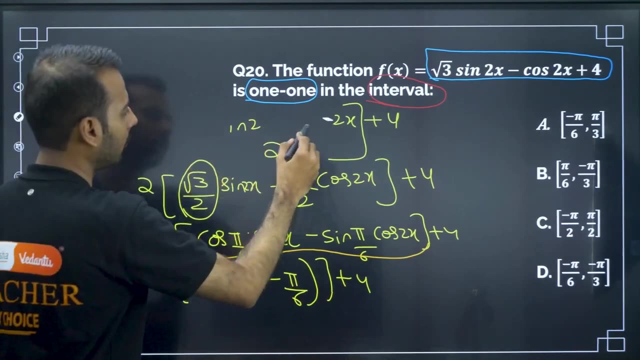 cos b. that can be written as sin a minus b. So this entire equation, I have transformed this entire. I am transforming it like this: that plus 4 as it is Now. one thing you must observe here: since here space is not there, I am writing it here. 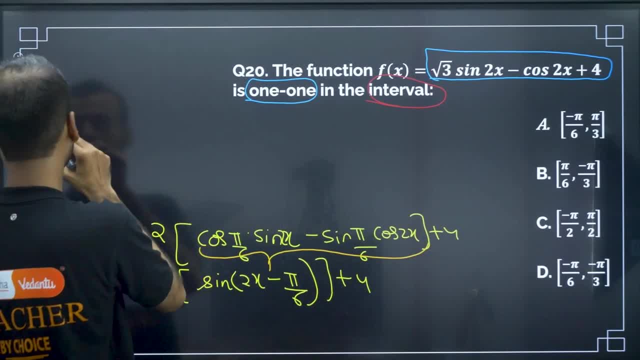 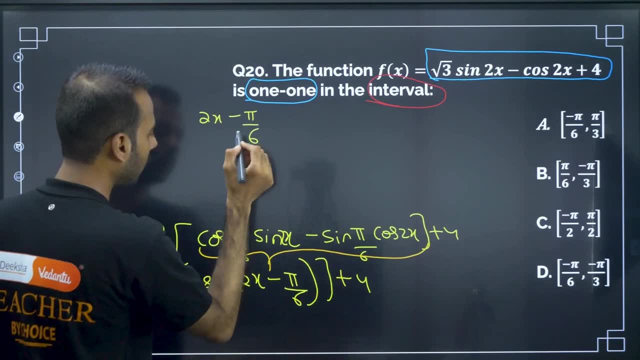 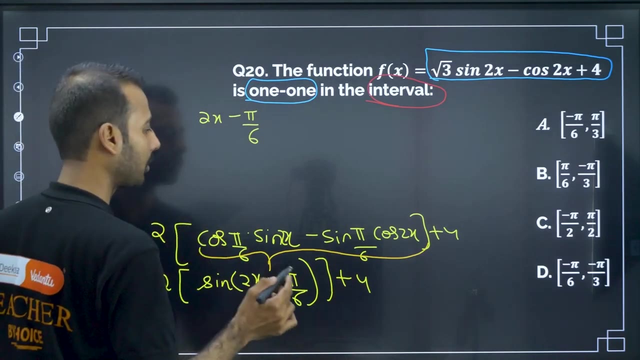 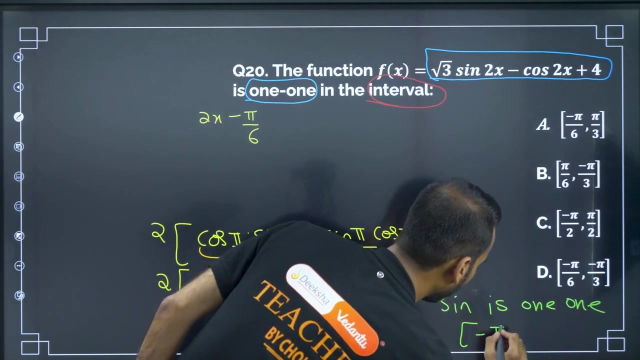 So how does this work? is when Sin a is 1. 1幹 can be written as 2x, 2x minus pi by 6, 2x. phenomena 1, 1 współ포 1-2x2간 2x- 1 by 6, 2x. See, I will try to recall when Sin is 1: 1.. Sin is 1: 1 in the range. 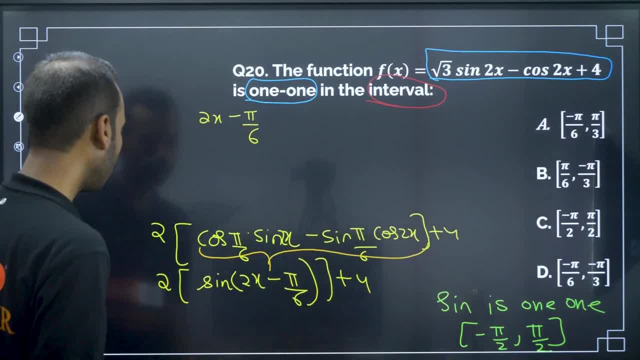 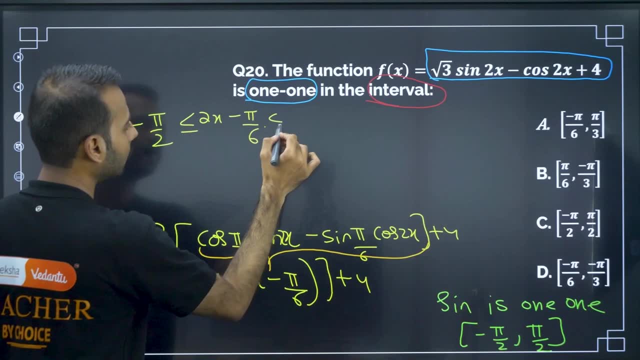 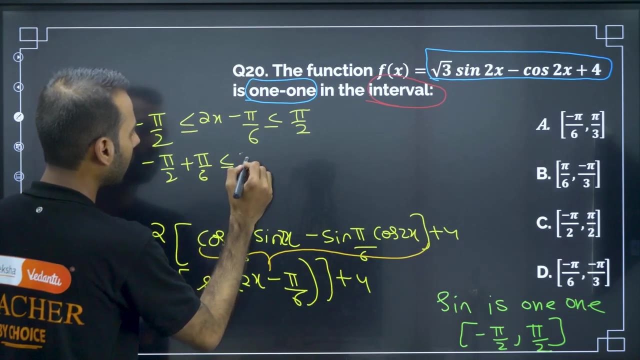 from minus pi by 2 to pi by 2.. So this 2x minus pi by 6 has to be has to be from minus pi by 2 to pi by 2.. If I add pi by 6 on both sides, minus pi by 2, plus pi by 6, less than or equal to 2x less. 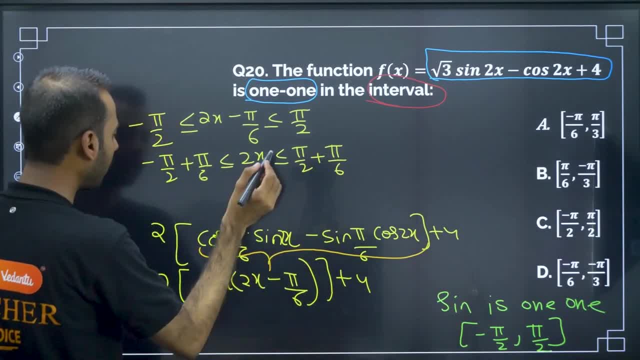 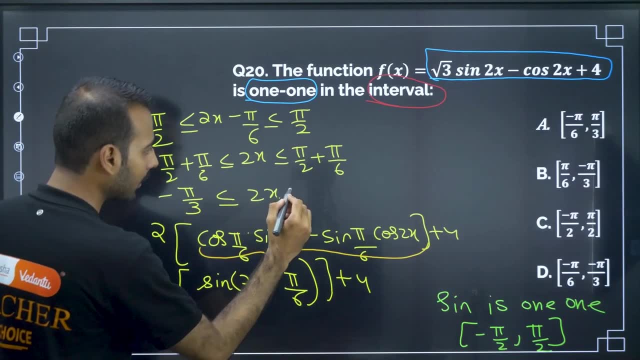 than or equal to pi by 2. I am adding pi by 6. I am trying to simplify this. So this is: minus minus pi by 3, minus pi by 3, less than or equal to 2x less than, or equal to 2 pi by 3, 2 pi by 3.. 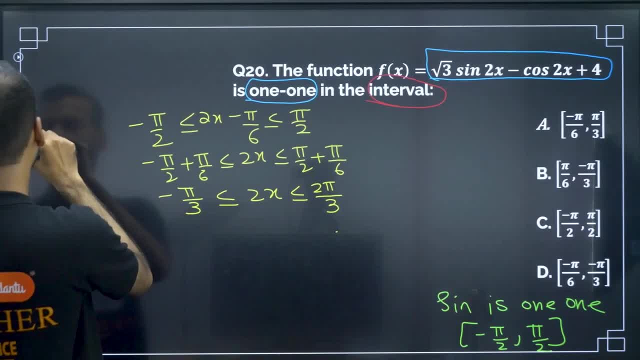 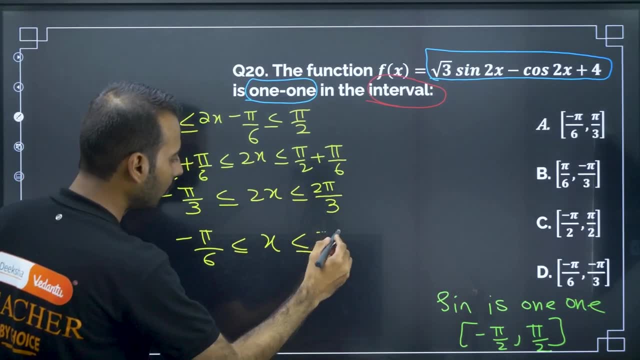 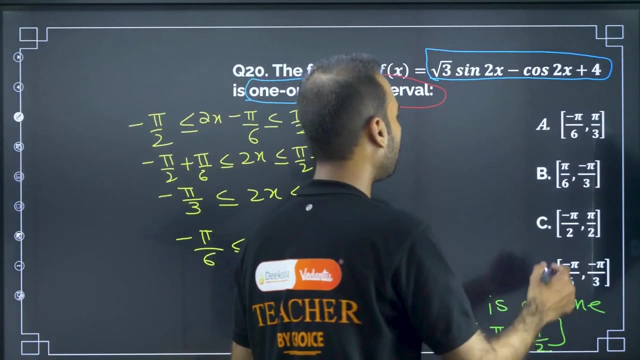 Let me erase this. let me erase this, all this. next, If I divide 2 on both sides, this becomes minus pi by 6, less than or equal to x, less than or equal to pi by 3.. So x belongs from minus pi by 6 to pi by 3, minus pi by 6 to pi by 3.. 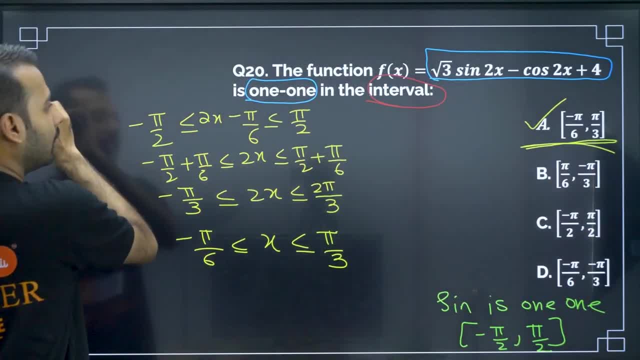 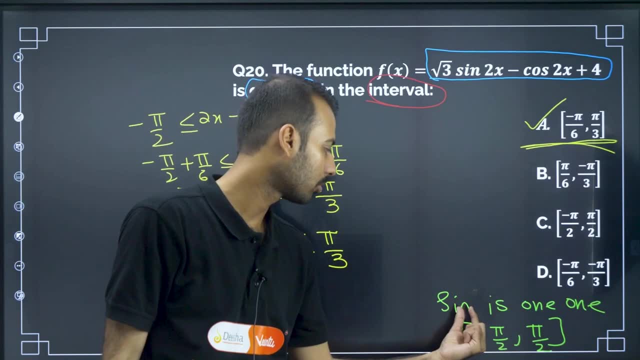 A is the answer for this: minus pi by 6 to minus pi by 3.. So the function is 1: 1 in the interval minus pi by 6 to pi by 3.. So one synopsis point we are supposed to know: sine is 1: 1 in minus pi. 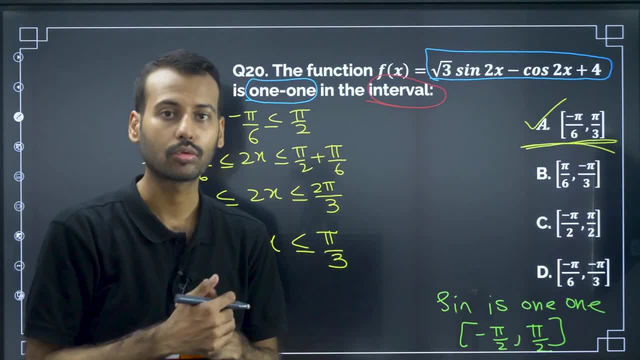 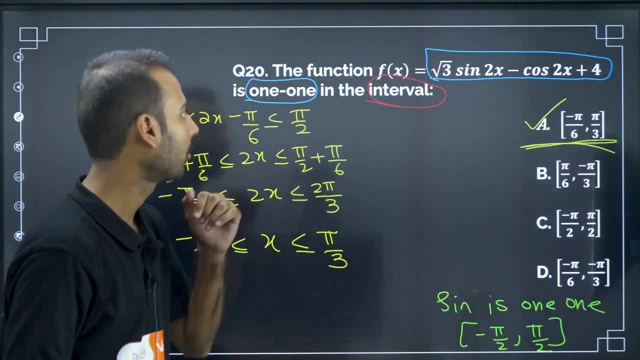 by 2 to pi by 2. and one more synopsis point that we are supposed to know for solving this problem is: sine a minus b is equal to sine a cos b minus cos a sine b. So with that, two synopsis points, you are able to solve this problem. Easy question, little time consuming not much time within one. 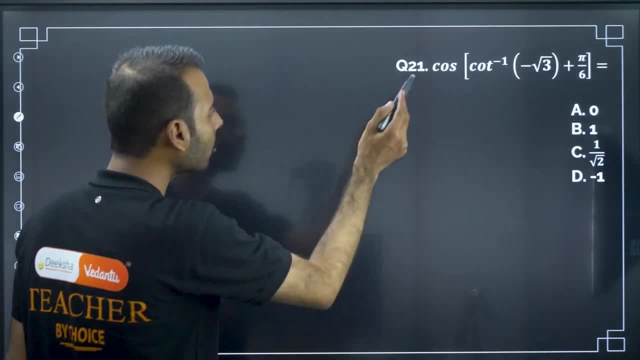 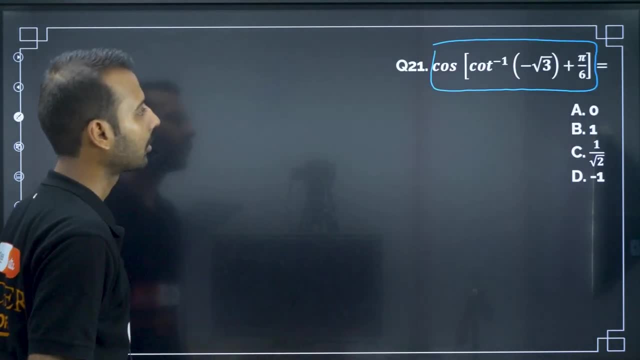 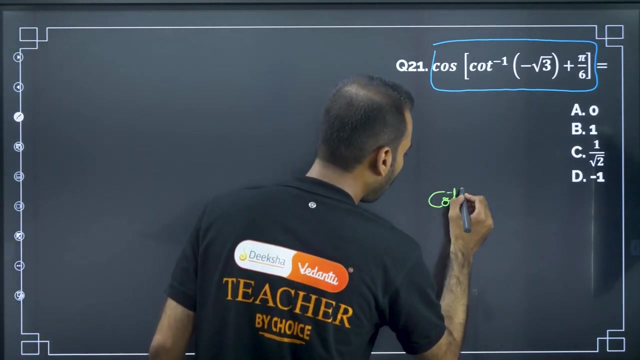 minute. we can solve this. Next, moving on to next question: Cos of, cos of. they are asking to find a value of cos of cot inverse. this Now: how to approach this problem. before approaching this problem, One synopsis point you should be knowing: cot inverse of. 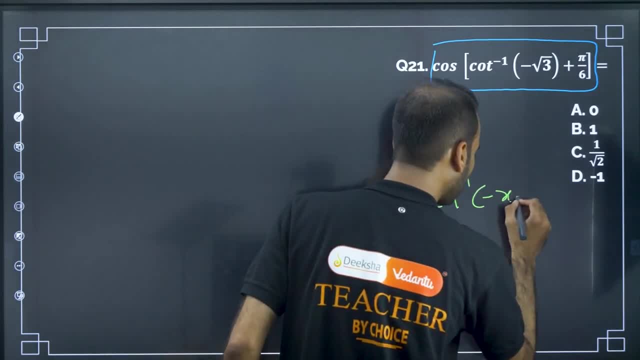 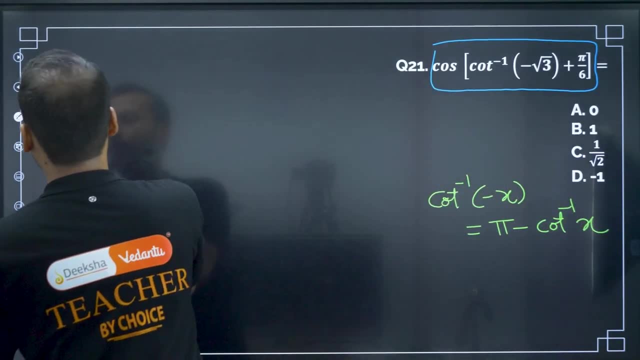 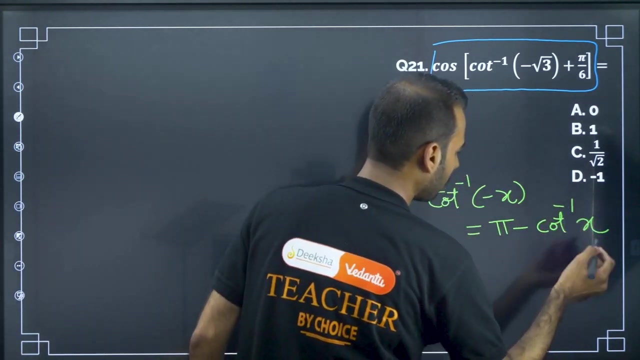 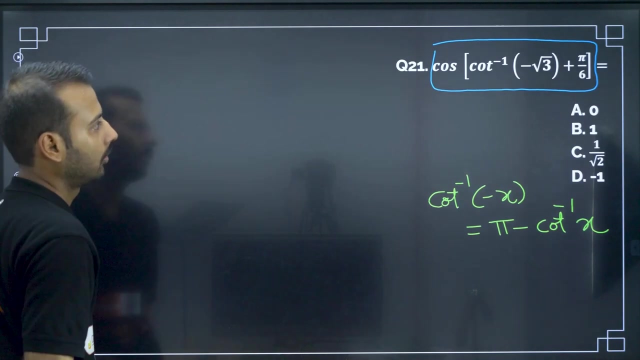 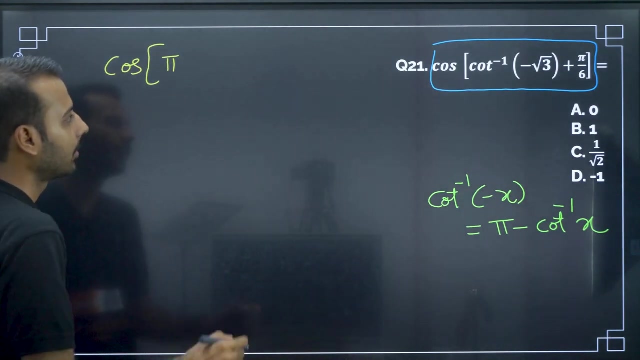 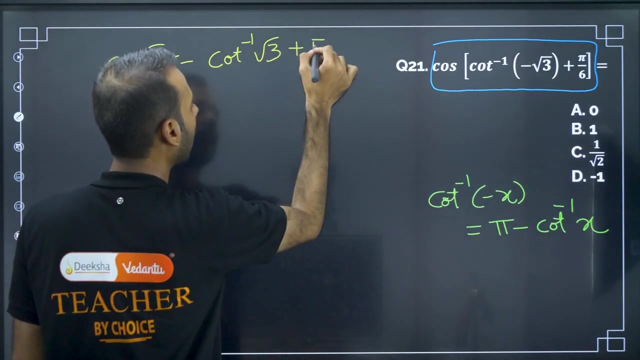 cot inverse of minus x is pi minus cot inverse x. pi minus cot inverse x. pi minus cot inverse of minus x is pi minus cot inverse of minus x. so cos of�리, cos of restraints of pi minus cot inverse can be written as pi minus cot inverse of minus. x is pi minus cot, inverse root 3 plus pi by 6 that I am giving, as it is Caught- inverse ofố root 3.. So that we are going to directly substitute this, So which is Effect второй, For the 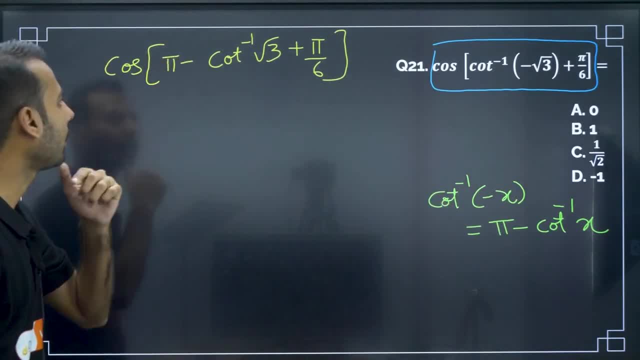 inverse. we are going to destroy integraph as it was already written as a respect. interpret вdim deeper: cot inverse of minus x is pi minus cot inverse of minus x. So prot inverse is pi minus cot minus cot inverse x. so i'm writing it like this: synopsis point you should be knowing. next, cos of. 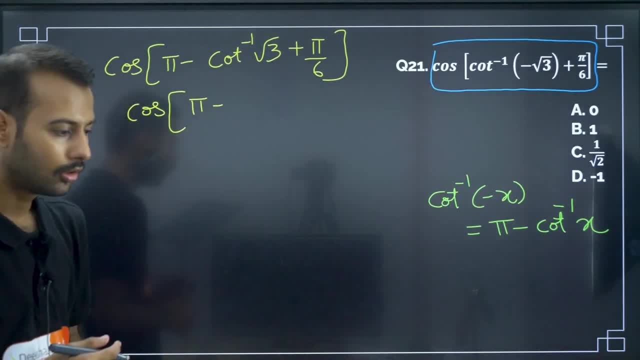 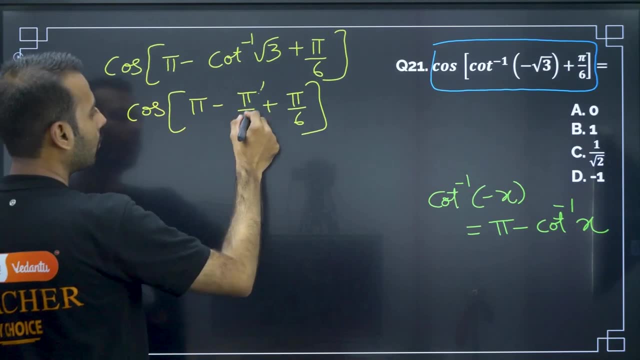 pi minus cot inverse root 3. cot inverse root 3 can be written as: minus pi by 6 plus pi by 6, minus pi by 6 plus pi, so this and this will get cancelled. cot inverse root 3 is pi by 6, so cos pi. 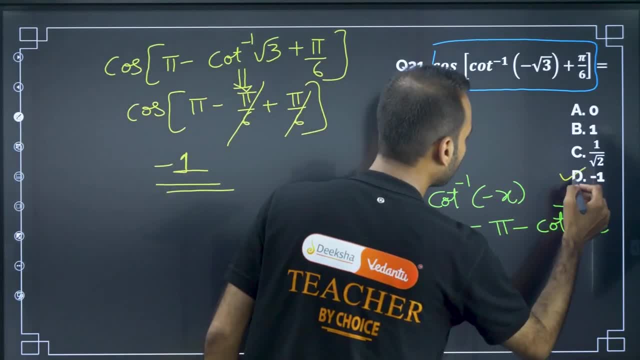 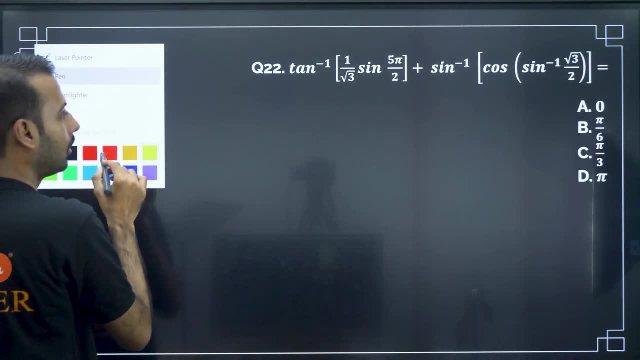 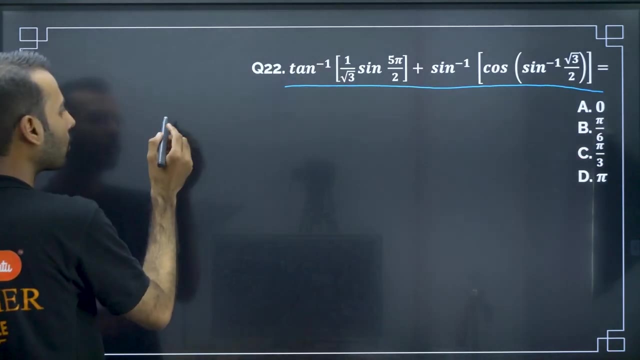 is minus 1. is there any such option like minus 1? yes, d is the answer. moving on to next question: tan of they have given one expression. they have given one expression. tan of this plus this is equal to. again, we just have to simplify this. so, simplification: tan inverse, tan inverse 1 by root. 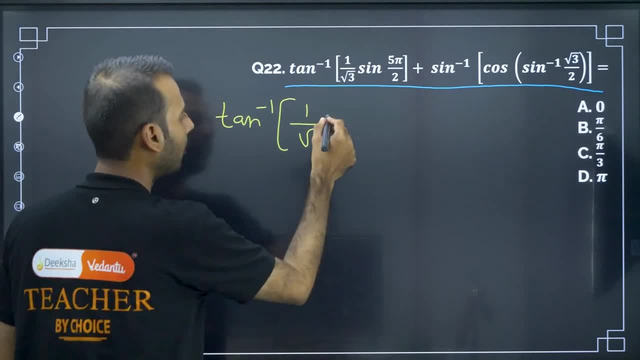 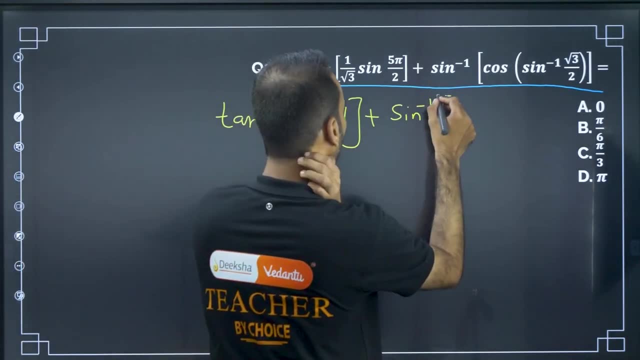 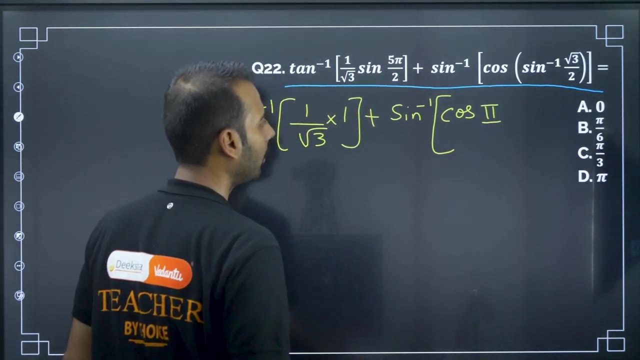 3, 1 by root 3 sin 5, pi by 2 can be written as 1, so i am writing this as 1 plus sin inverse sin inverse cos, cos, sin inverse root 3 by 2. this can be written as pi by pi by 3, so sin inverse root 3 by 2, i am assuming. 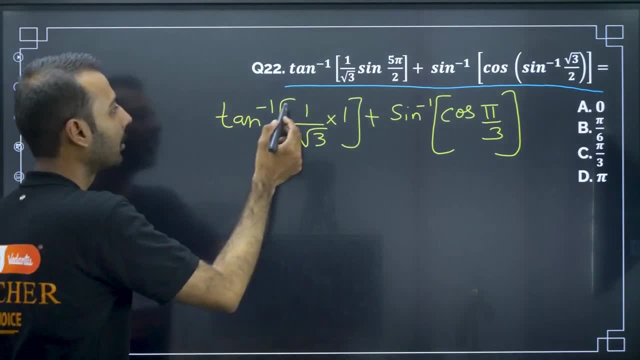 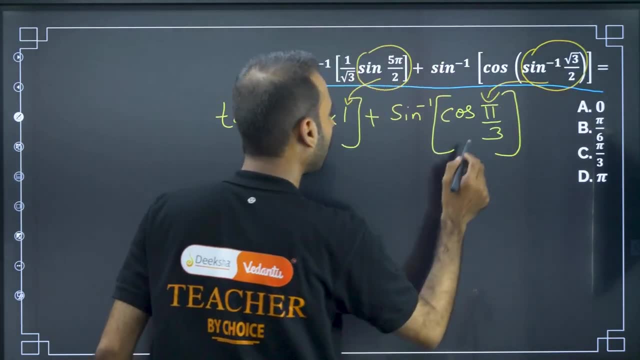 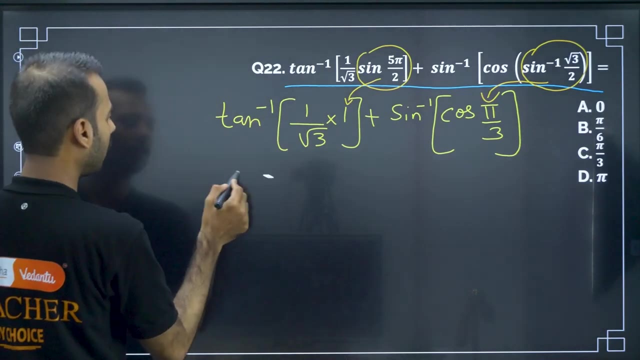 students, you are able to make out what i am replacing: sin 5, pi by 2. for that i am writing this as 1. for sin inverse this: i am writing this as pi by 3. next, moving on to next tan inverse: tan inverse 1 by root 3. tan inverse 1 by root 3 is tan inverse pi by 6. 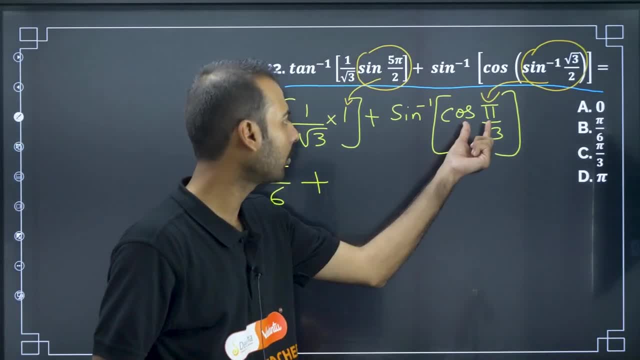 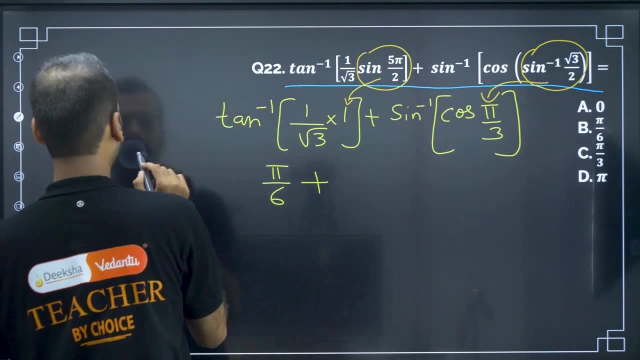 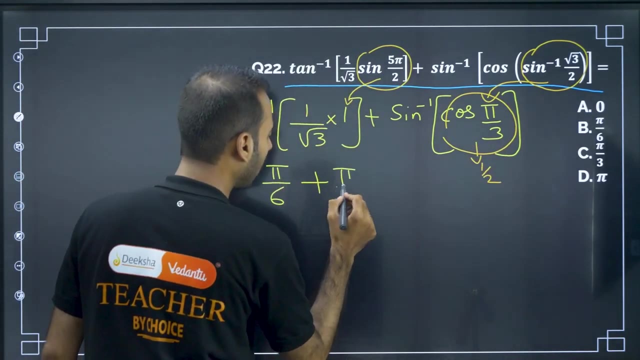 plus sin inverse cos pi by 3 is cos pi by 3 is 1 by 2. sin inverse 1 by 2 is cos pi by 3. value is 1 byOO. sin inverse 1 by 2 is pi by 6. so pi by 6 plus pi by 6 is 2 pi by 6which is equal to. 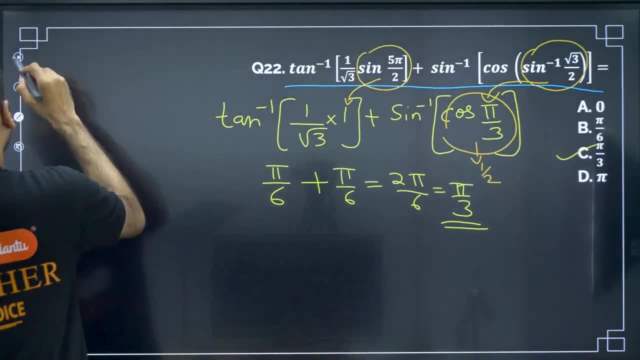 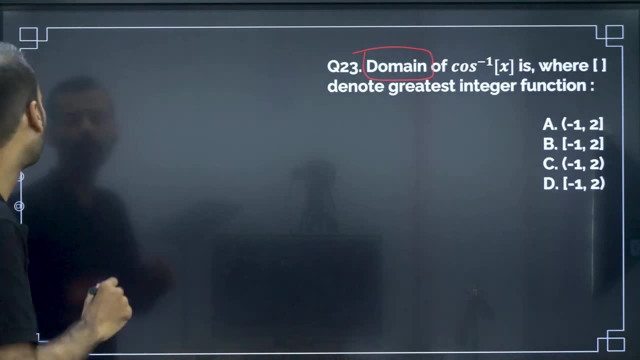 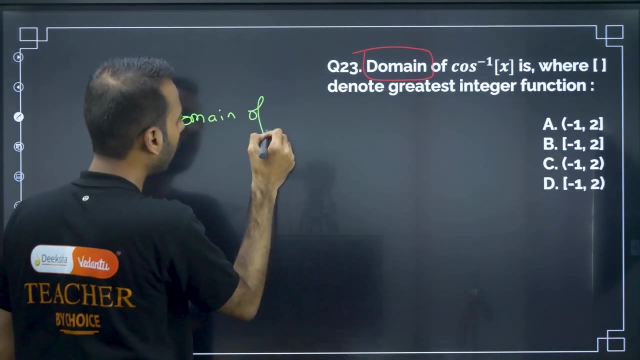 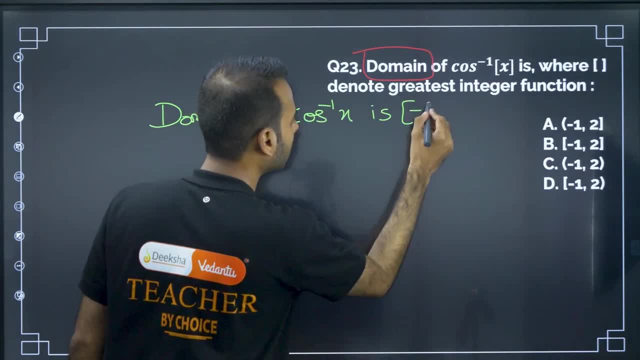 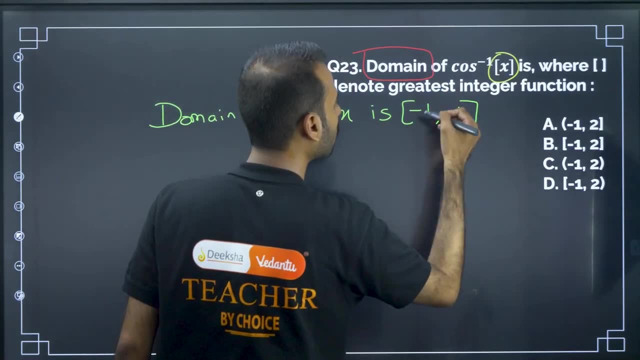 cos inverse x is minus 1 to 1, but here they have included gif also. they have included this gif also. So for gif minus 1, if I give, it is ok, I can give up to 2,, but I should. 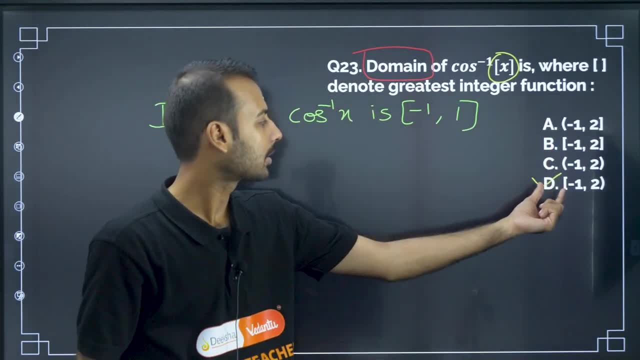 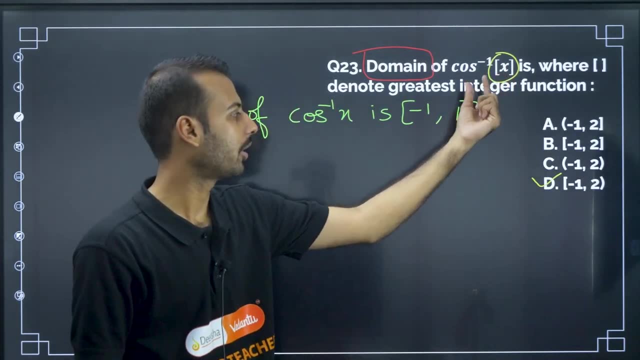 not give 2, so d is the answer. see, I try to analyze this. if I am giving minus 1 as input to this, it is ok. above minus 1 to, anyways I can give, I will get minus 1 as input only. 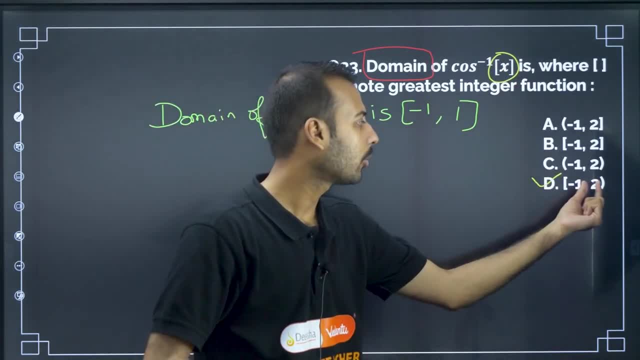 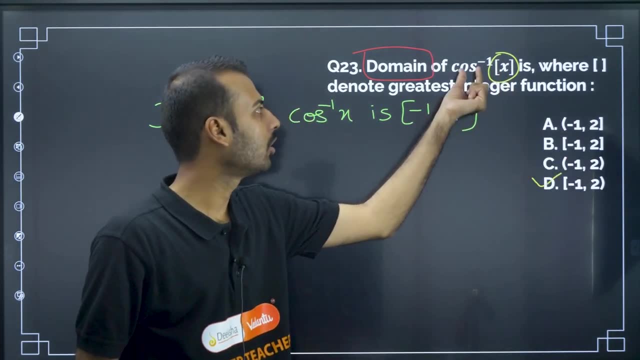 but if up to 1, ok, it is ok, that will take. if I am giving 1.9999 or 1.9 bar, this gif will make it as 1 and it will give that as input, also minus 1 to 2, it is all analysis. 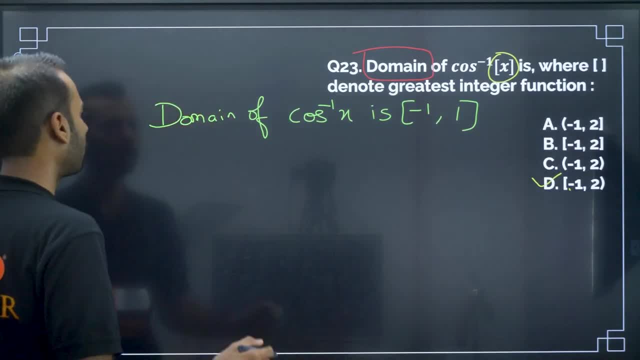 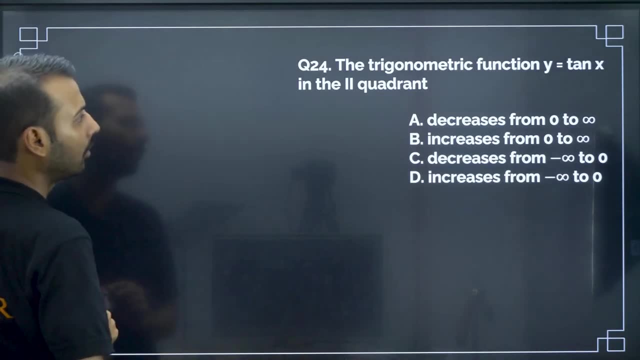 of this. again, very simple analysis only. Moving on to next question, The trigonometric function y is equal to one trigonometric function they have given in the quadrant. what are they asking? decreases, increases, decreases, increases, whether this. 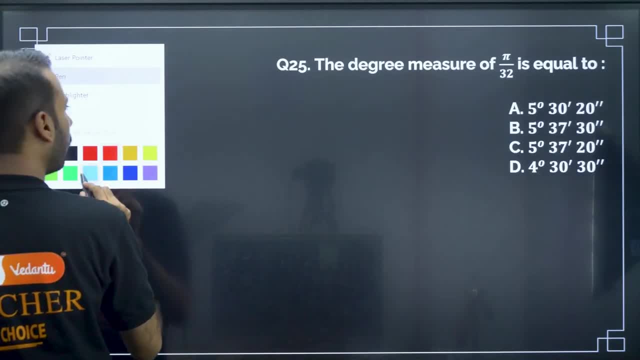 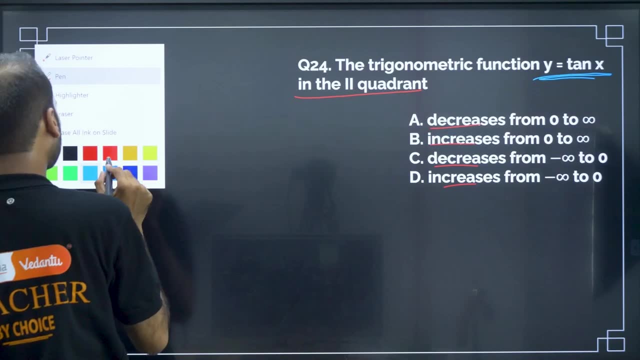 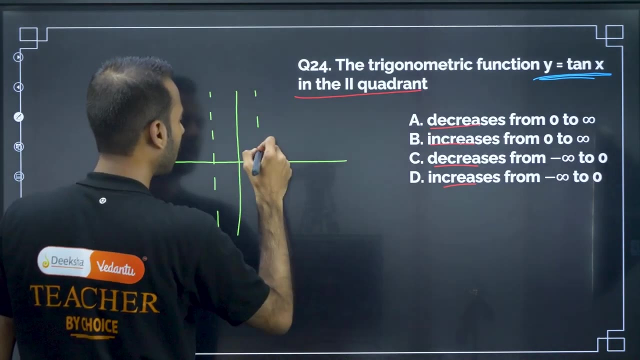 will increase or decrease. they are asking that, so what information they have given here. if you observe this question, y is equal to tan x. now, the moment you see, y is equal to tan x. tan x graph should come to your mind. 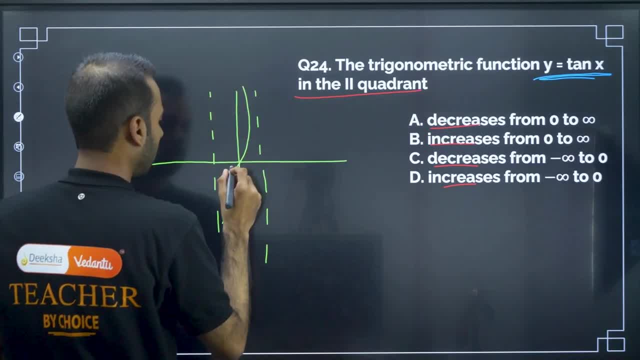 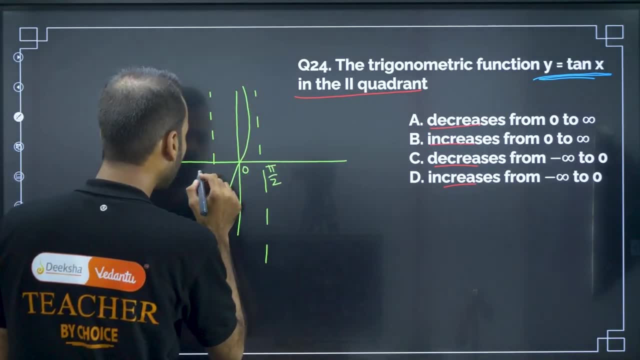 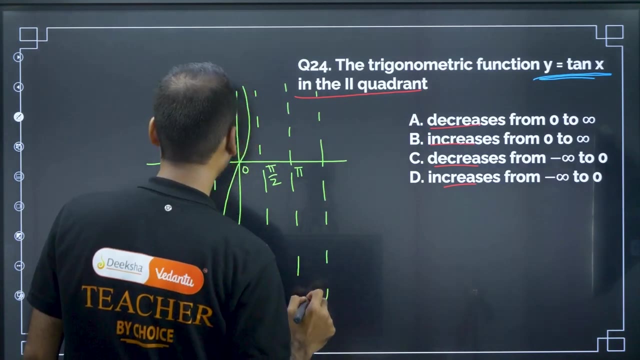 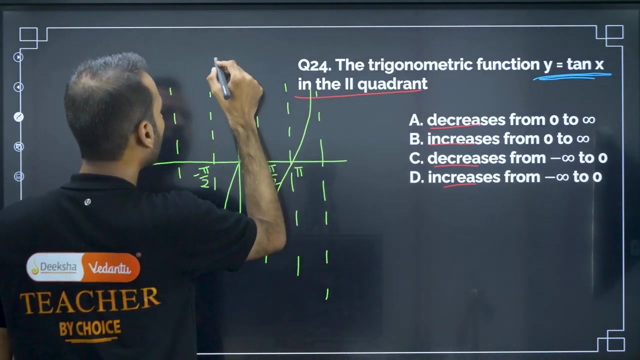 What is that graph? This is 0,. this is 0, this is pi by 2, this is minus pi by 2, this is minus pi by 2, this is pi, bla, bla, bla, bla bla. and this is bla bla bla bla. so tan x- y is equal to tan x- the. 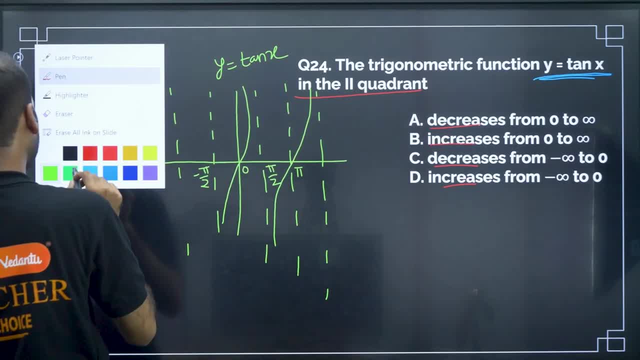 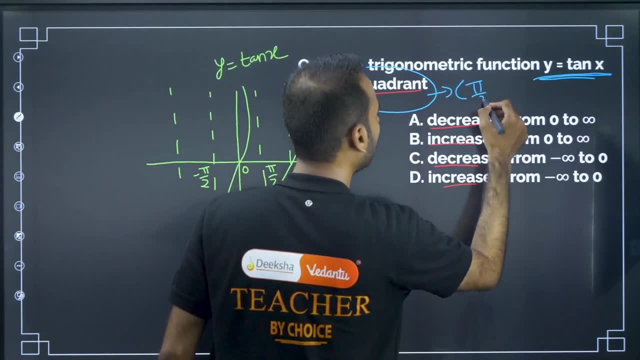 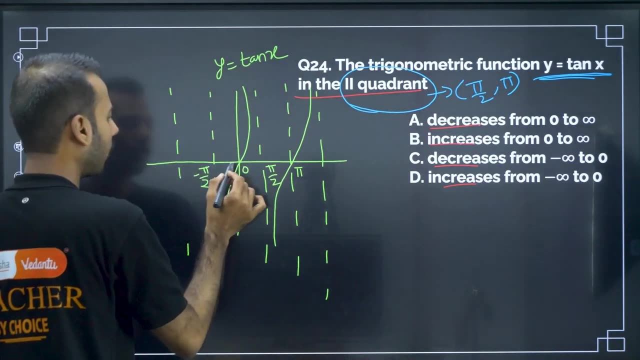 trigonometric. Ok, Second quadrant. second quadrant means what second quadrant means? second quadrant means from where to where, pi by 2 to pi. So if I observe this, y is equal to tan x graph from pi by 2 to pi by 2, if I observe from: 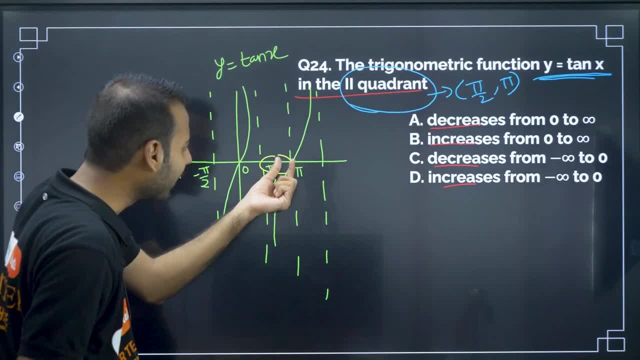 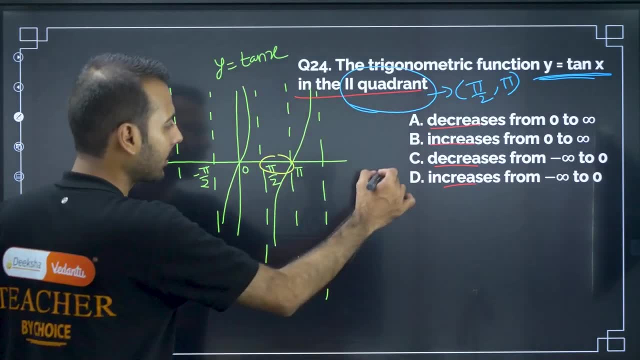 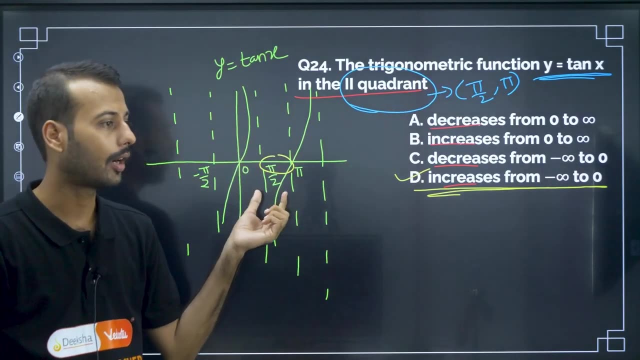 this region. what happens here? it is increasing, increasing from minus infinity to 0, increases from minus infinity to 0, is there any such option? increases, yes, this is the answer. so increases from minus infinity to 0.. So, if you are having this tan x graph in your mind, hardly it will take one second just. 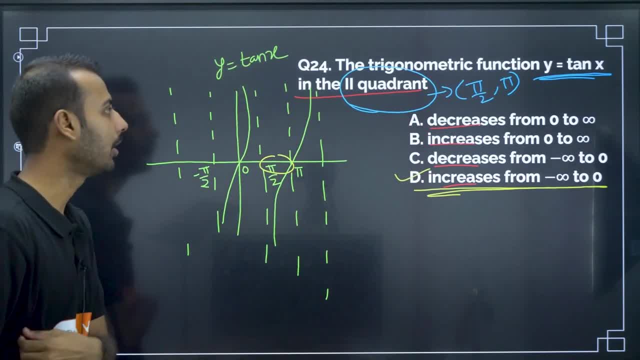 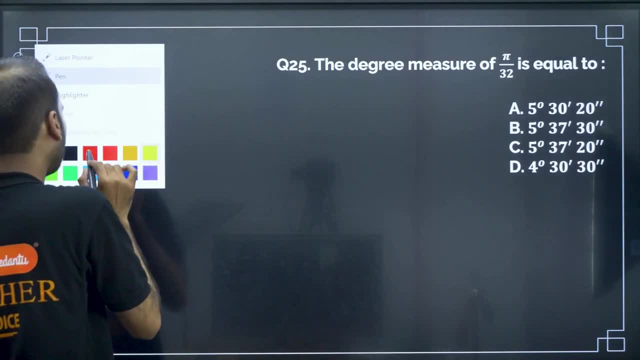 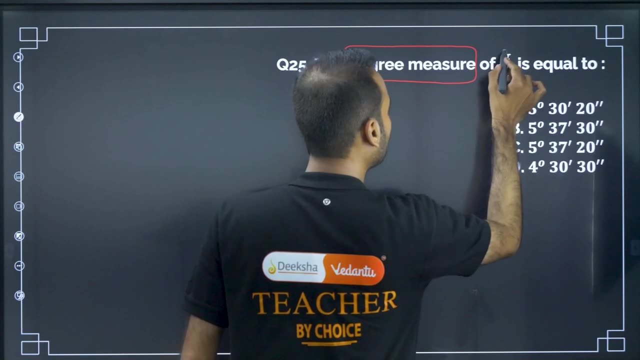 to mark this. so this graphs. you have to fix this in your mind. Next, moving on to next question: the degree measure of degree measure, of degree measure. so what are they asking? They are asking degree measure of what of pi by 32 is equal to. they are asking degree. 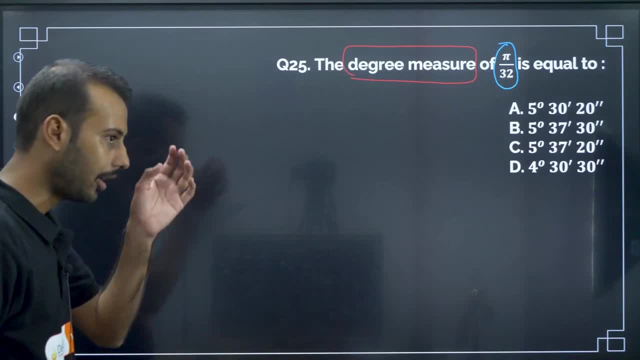 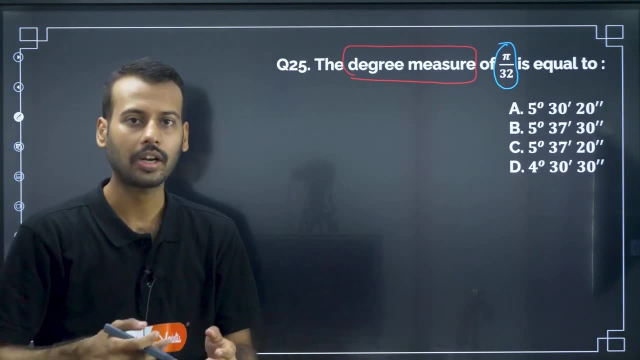 measure of. So this, all this degree measure, radian measure, all this they will start. they will teach you in starting of trigonometry. introduction to trigonometry starts with definition of angle and then they will say units of angle, all that there. 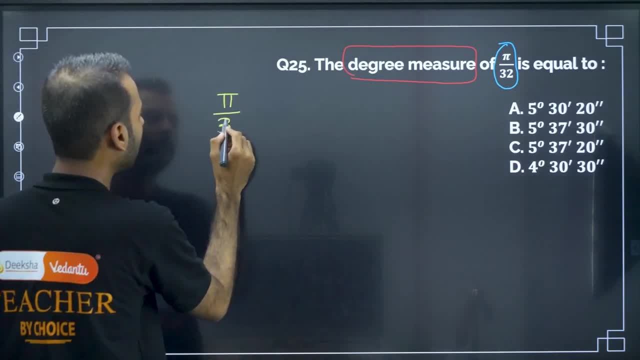 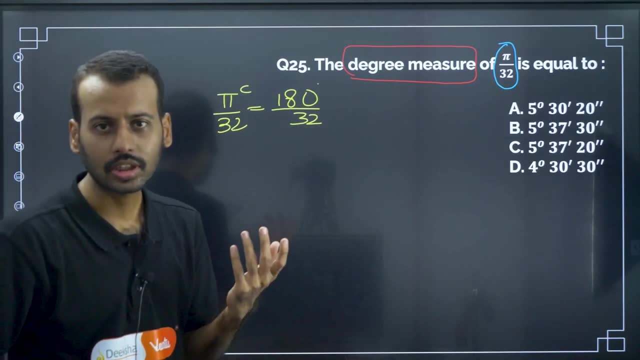 So pi by 32 is equal to. how to approach this? pi by 32, pi radian is equal to. this is 180 degree divided by 32.. Now you should know division, division. they will teach in fourth standard, so you just 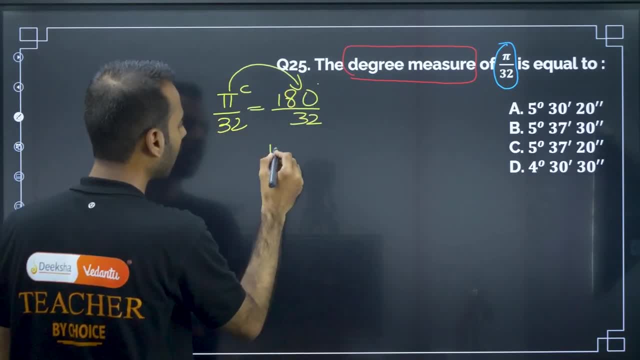 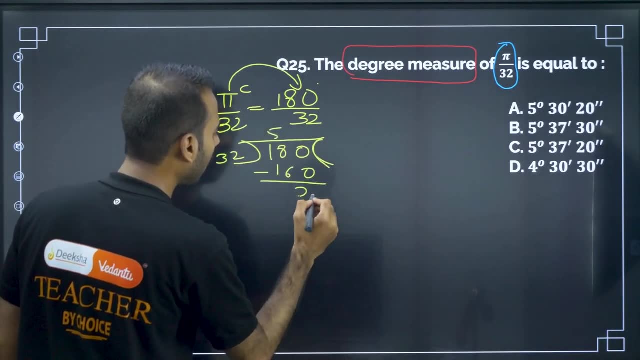 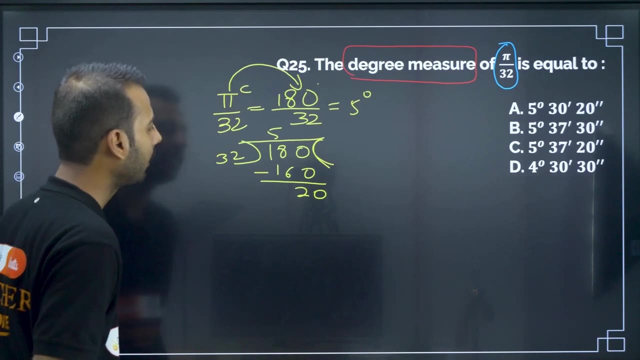 have to divide this pi radian is equal to 180 degree. 180 degree divided by 32.. Ok, So 180 degree divided by pi is a 160,. so here we are left with 20,, 20.. So 180, this is 5 degree, this is 5 degree. 20 by 32,, 32,, again, degrees only. but if I 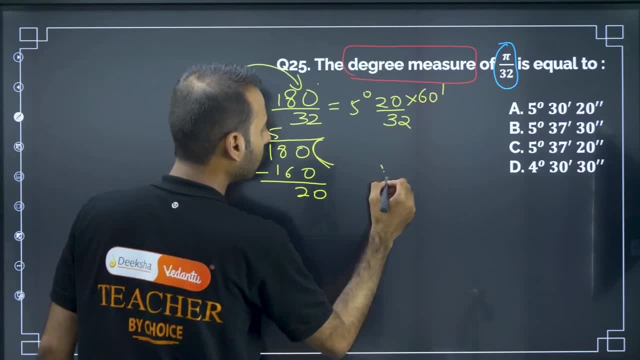 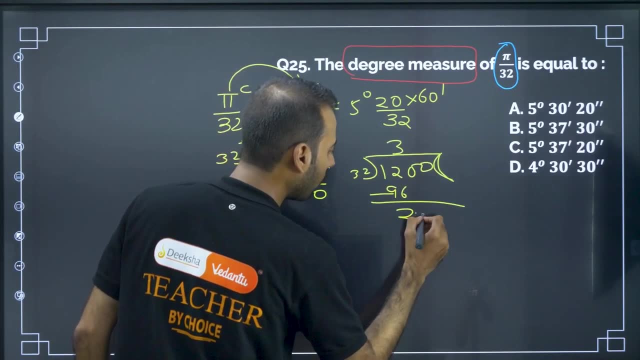 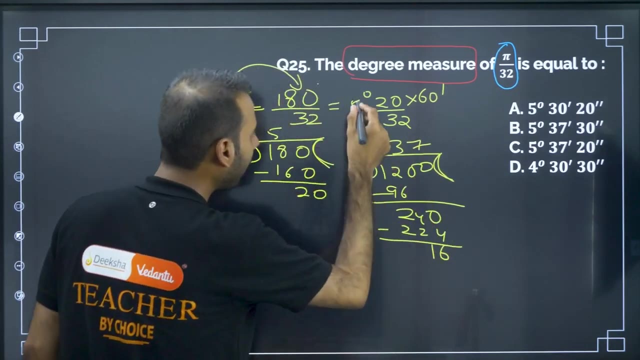 want, I will multiply this and I will write in: so 1200, 1200 divided by 32, 32, 3 is a 96. 24.. So 7s are 32, 7s are 224, here I am left with 16.. 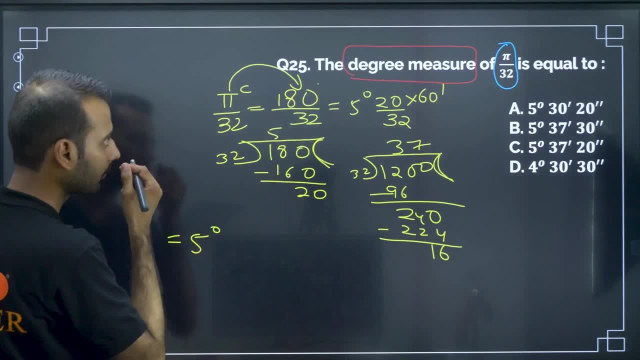 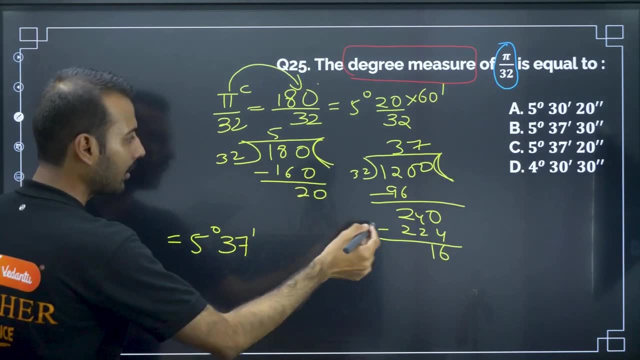 Now this 5 degree, this 5 degrees, 20 by 32 into 60, that is, this can be written as 37 minutes and then 16 by 32,, 16 by 32, this is also in minutes for this, if I convert. 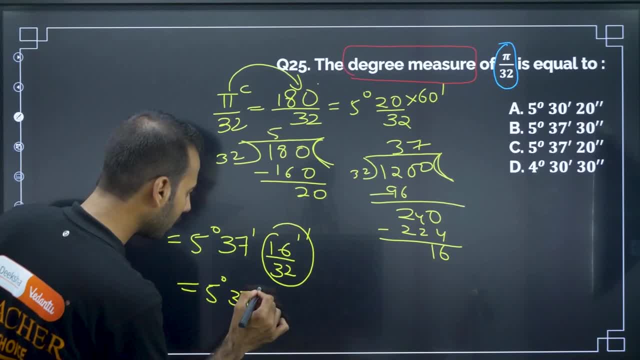 to seconds: 5 degrees, 37 minutes, 37 minutes. This is 0.5 minute. Ok, Ok, If I write in seconds, this becomes 30 seconds, so is there any option? 5 degrees, 37 minute. 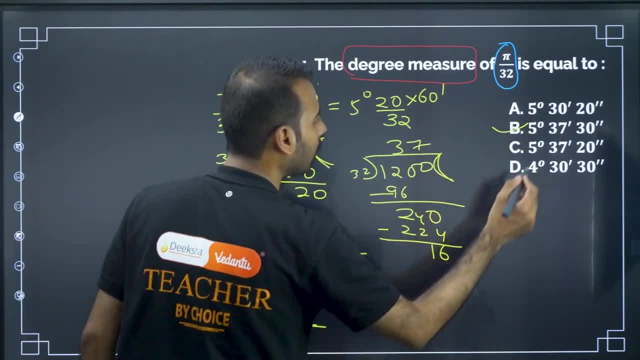 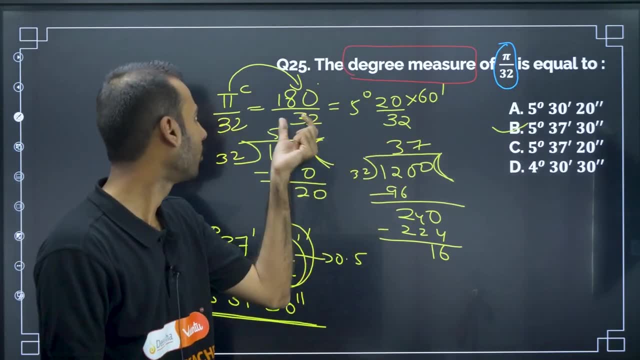 and 20, 30 seconds. yes, B is the answer. Moving on to next, see, this was very easy question, only just division. you should know that they will teach in fourth standard. and also pi: radian is equal to 180 degree trigonometry. 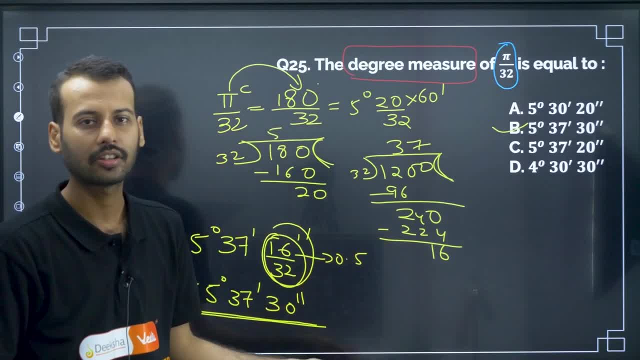 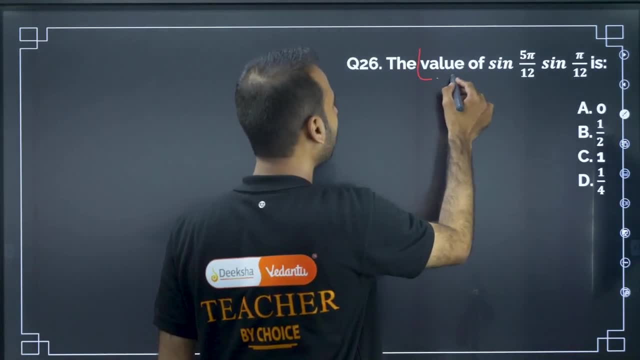 starts from here. only that also. you should only division hardly. it will take 30 or 40 seconds for division. Moving on to next question: the value of sign. What are they asking in this question? They are asking value of sign 5 pi by 2 L. sign 5 pi by 2 L is they are asking to find. 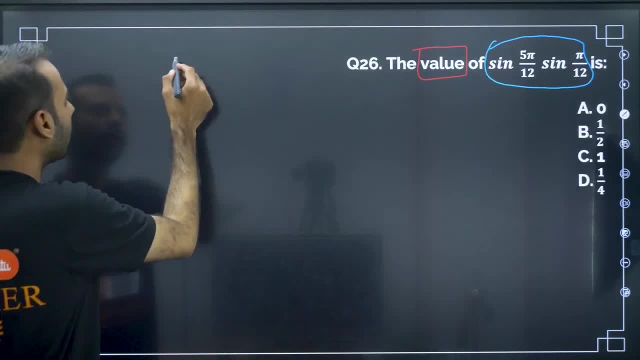 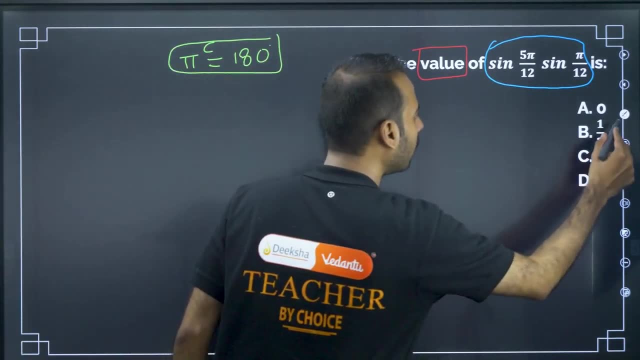 this. So one thing you should be knowing this. I will assume all the students who are watching this video might be aware of this: pi radian is equal to 180 degrees. Now, further, if you observe this question, what are they asking? sign and here sign. 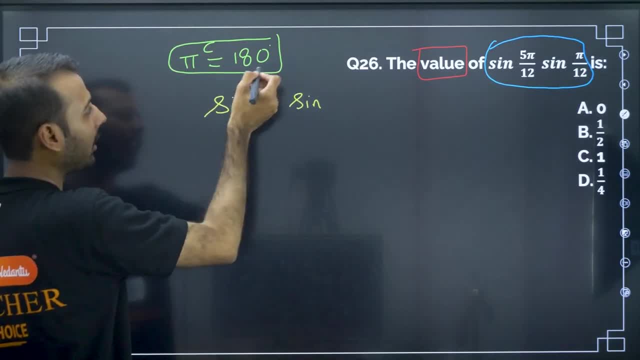 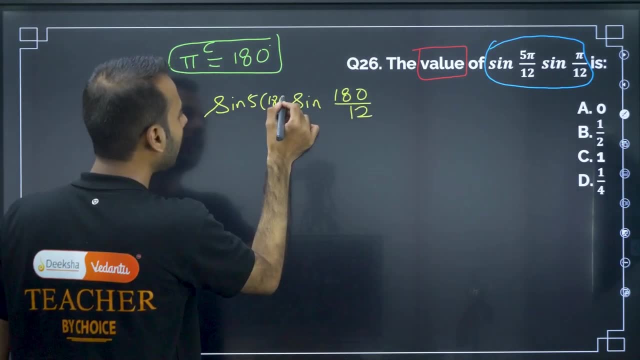 pi by 2 L in place of pi by 2 L. it is 180 by 2 L, 180 by 2 L. So what are they asking? They are asking pi 180 by 2 L and also here pi 180, 180 by 2 L. so sign of sign 75, sign. 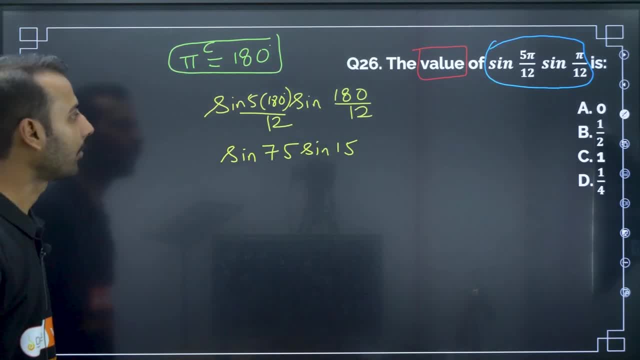 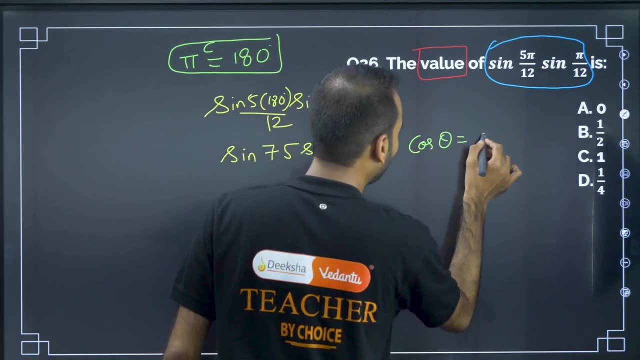 15, sign 75, sign 15.. One more synopsis point you should be knowing. what is that. sin cos theta is equal to sin of 90 minus theta, or sin 90, sin theta is equal to pi cos theta. What is that? 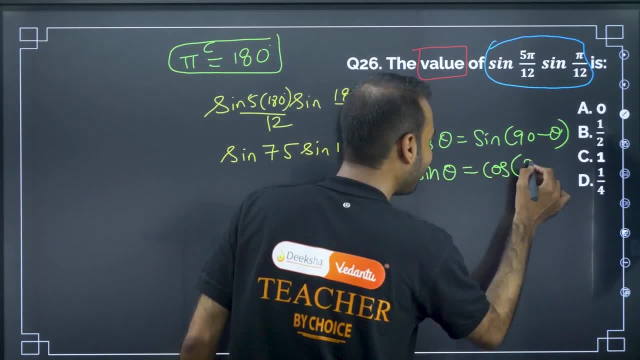 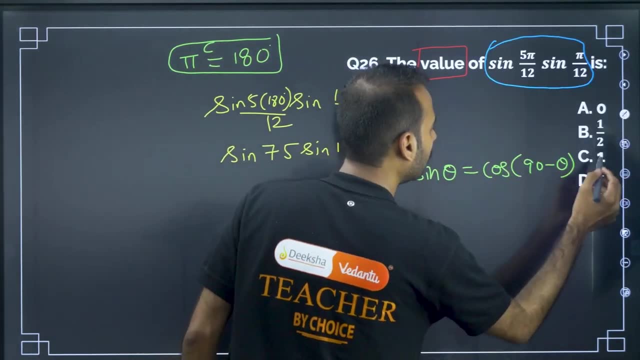 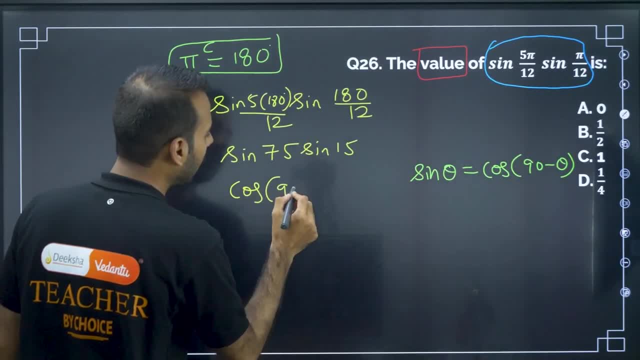 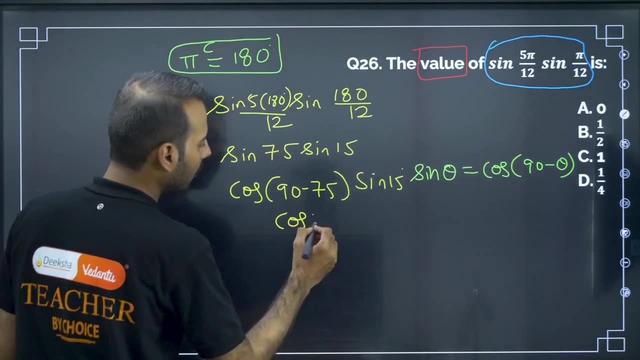 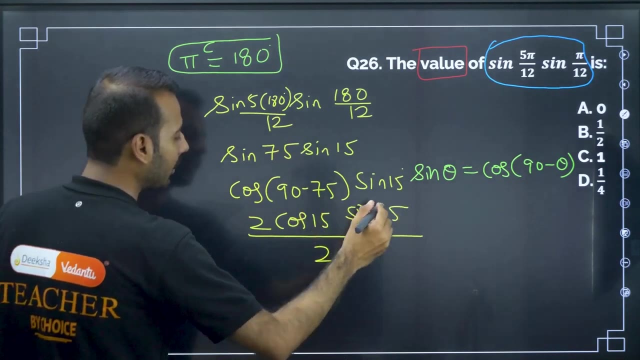 to cos of 90 minus 75 is equal to sin 15.. So this is cos 15, sin 15, if I write 2 here and if I divide by 2, so 2 cos 15, sin 15 is sin 30.. 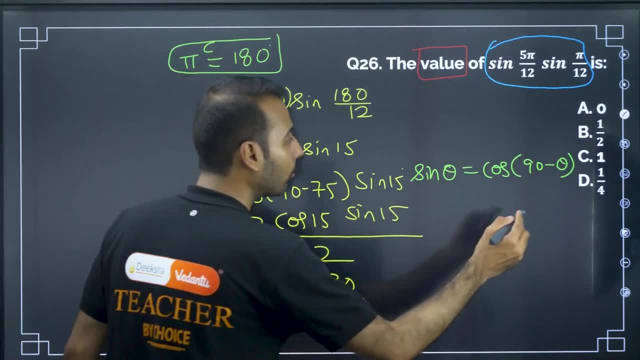 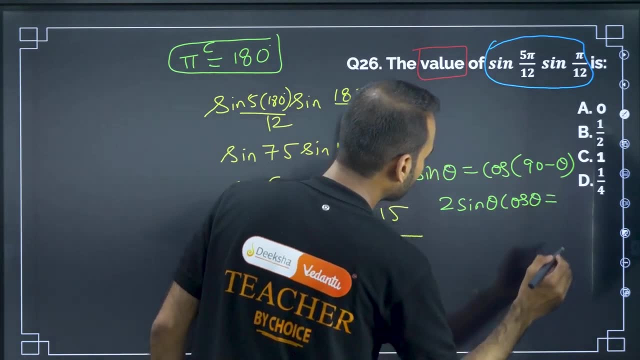 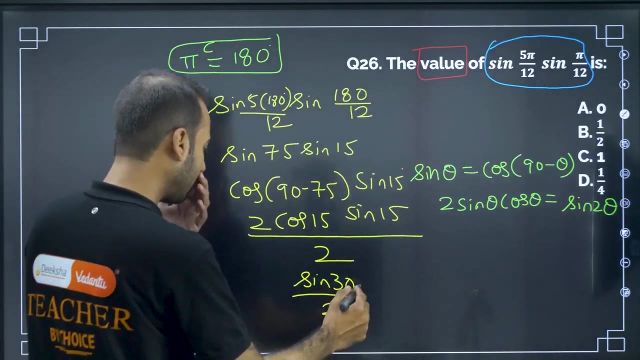 So this is sin 15.. 30 divided by again one more formula. you should be able to recall at this point what is that: 2 sin theta cos theta. 2 sin theta cos theta is equal to sin 2 theta. Next, moving on to this sin 30, value is 1 by 2, and already one more 2 is present here. 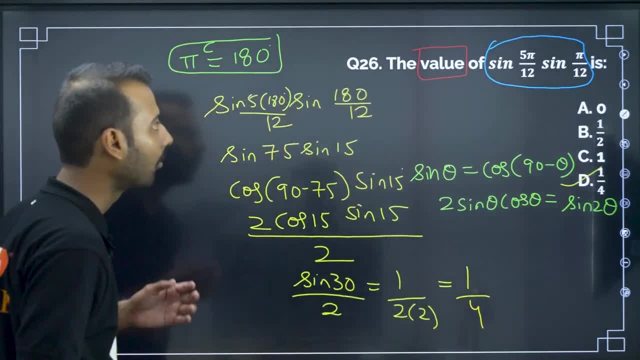 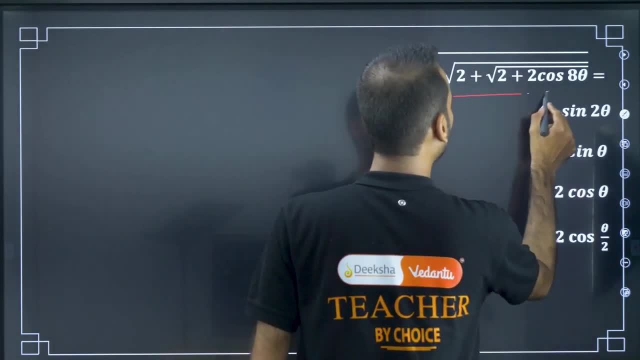 So this is overall 1 by 4, so the answer is 1 by 4.. Moving on to next question, root of this: they are asking to find the value of this For this one synopsis point. you should be knowing what is that synopsis point. I will. 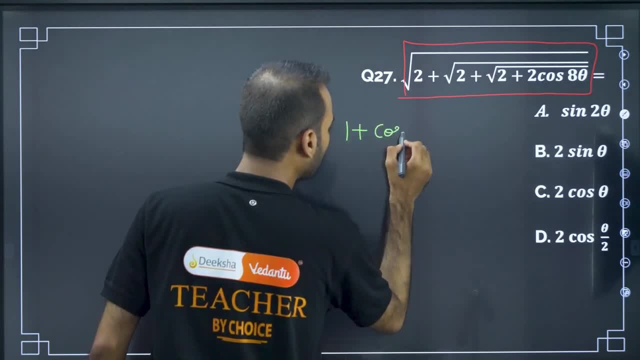 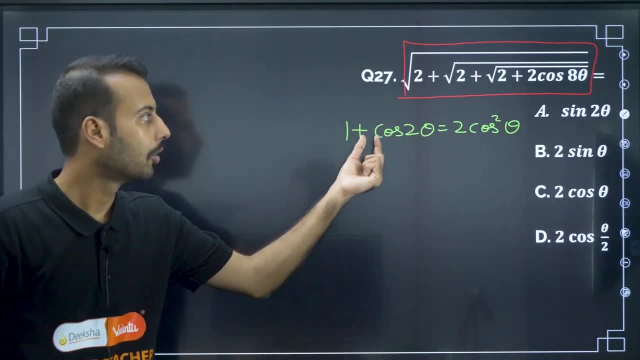 write here: 1 plus cos 2 theta is equal to 2 cos square theta, 2 cos square theta. This synopsis point proof everything. it is there in trigonometry chapter. So 1 plus cos 2 theta is equal to 2 cos square theta. 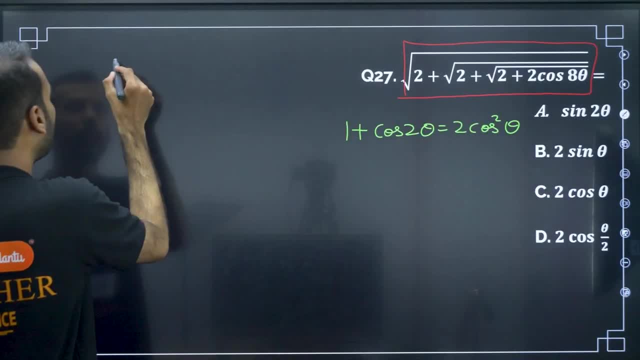 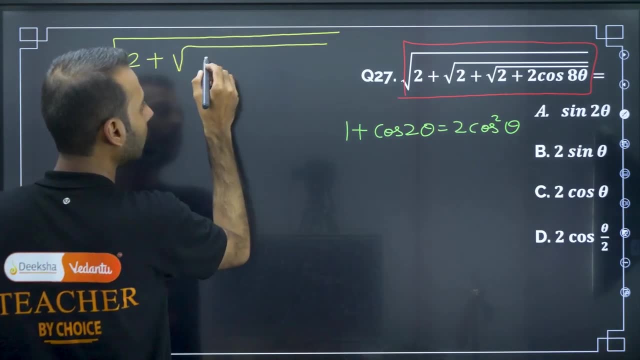 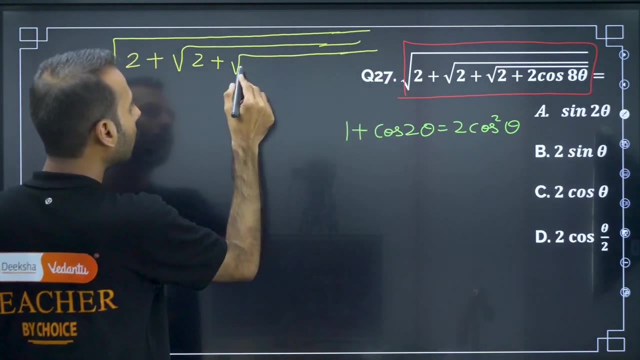 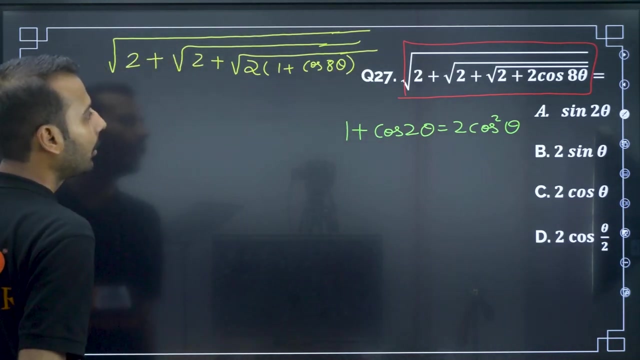 So first let me copy and paste That question here. let me copy and paste that question here: root of 2 plus 2 plus under root of 2 plus under root of under root of 2.. If I take 2 common from that, I am left with 1 plus cos 8 theta. 1 plus cos 8 theta under. 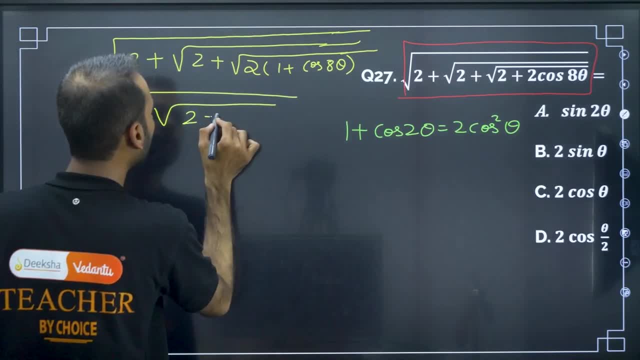 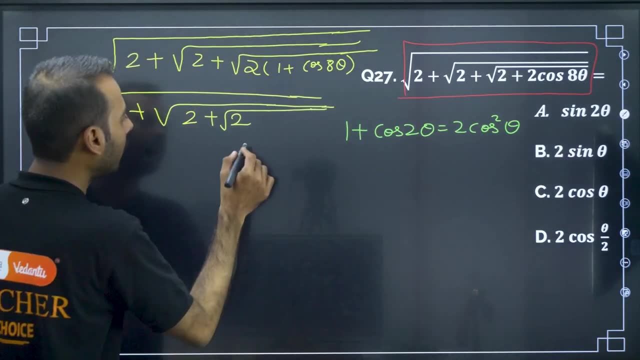 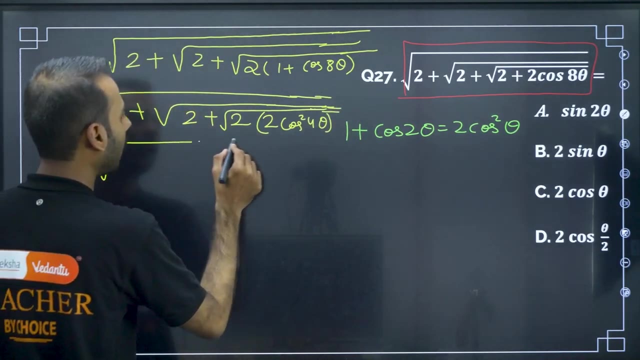 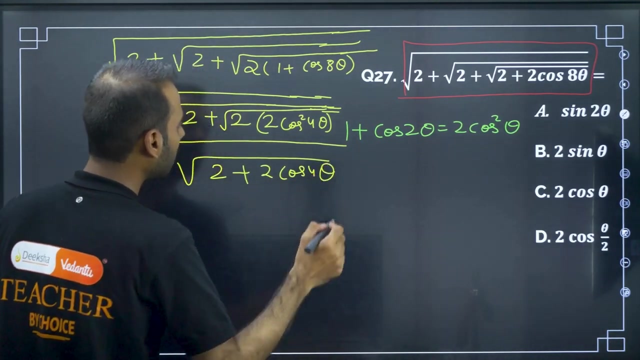 root of 2 plus 2 plus 2.. Here if I write under root 2 in place of 1 plus cos 8 theta, this can be written as 2 cos square 4 theta. 2 cos square 4 theta. Next, under root of 2 plus. under root of 2 plus 2 cos 4 theta. 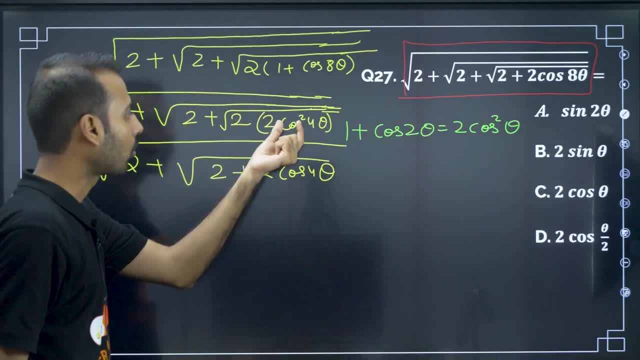 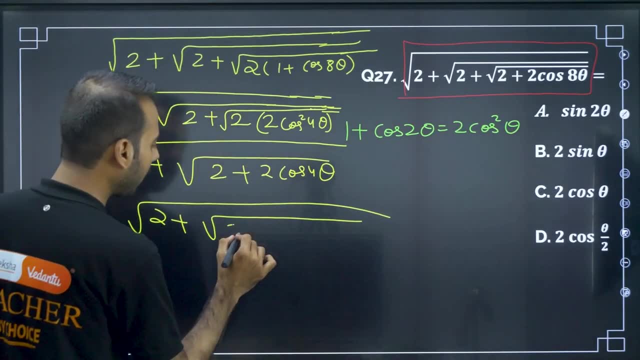 See here this 2, 2 is a 4. if I bring it out of root it becomes 2 cos square 4 theta root. they will get composed all this Next 2 plus under root of 2.. 2 if I take common 1 plus cos 4, theta 1 plus 2.. 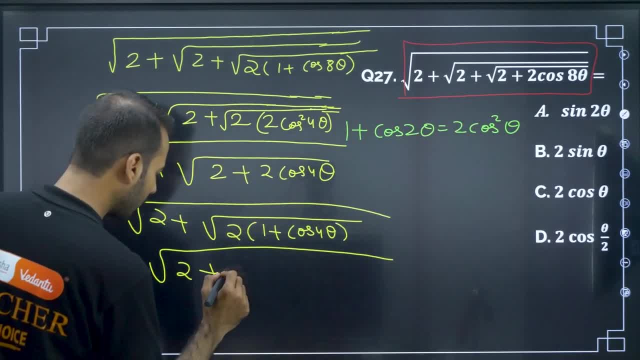 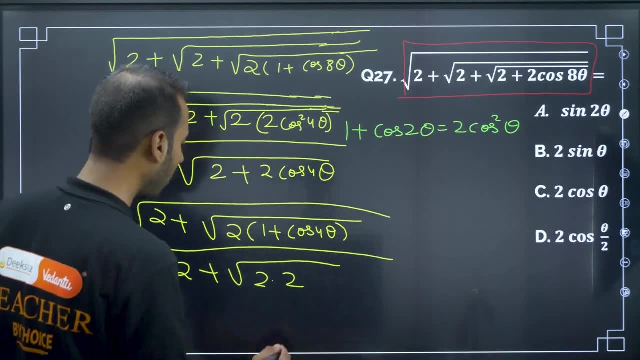 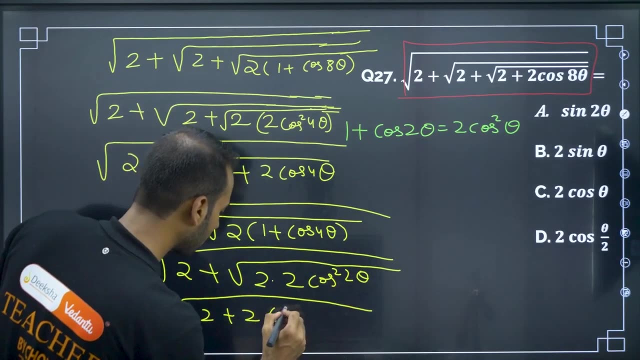 Again I will use this formula under root of 2 plus under root of 2: 2 cos 4 theta, cos 4 theta. if I write that as 2 cos square 2 cos square 2 theta, So under root of 2 plus 2 cos 2 theta. if I drag this next under root of 2, if I take 1, 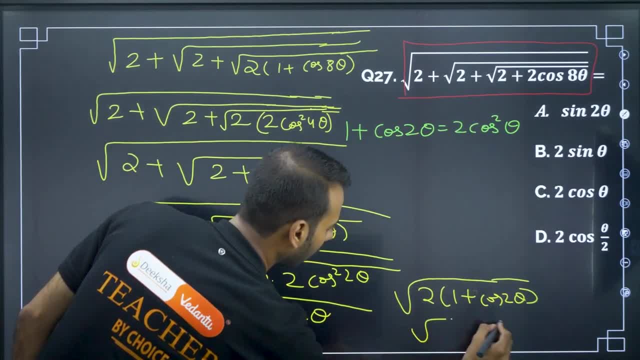 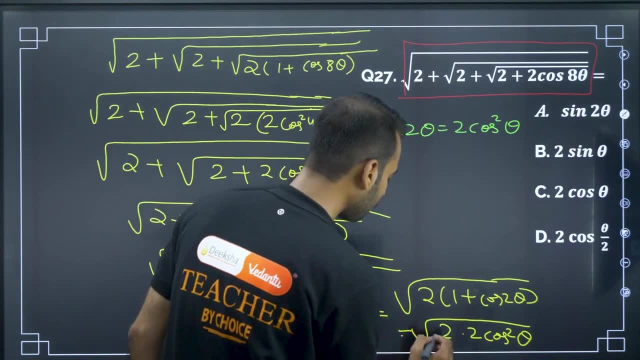 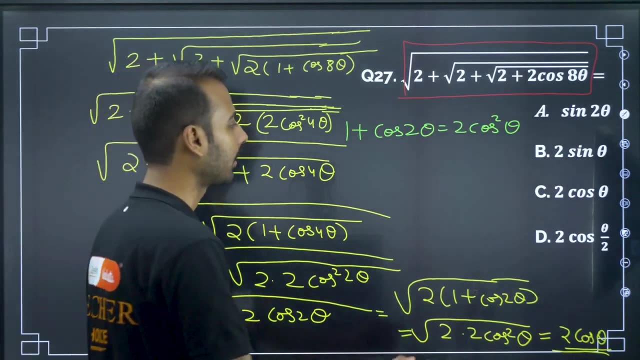 plus cos 2 theta, cos 2 theta under root of 2: 2 cos square theta, 2 cos square theta. So further, further, this can be written as 2 cos theta. So is there any option like 2 cos theta? yes, C is the answer. moving on to next question, 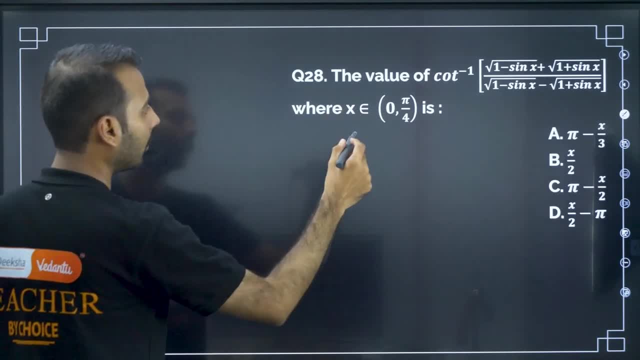 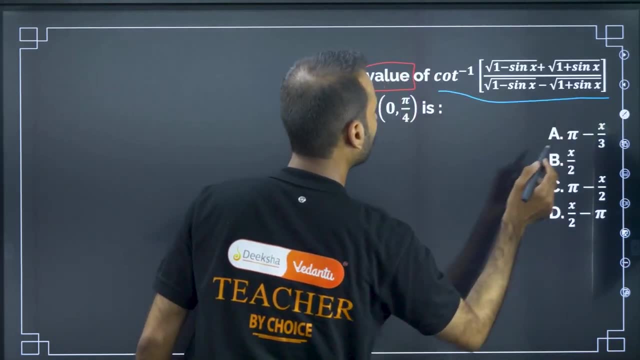 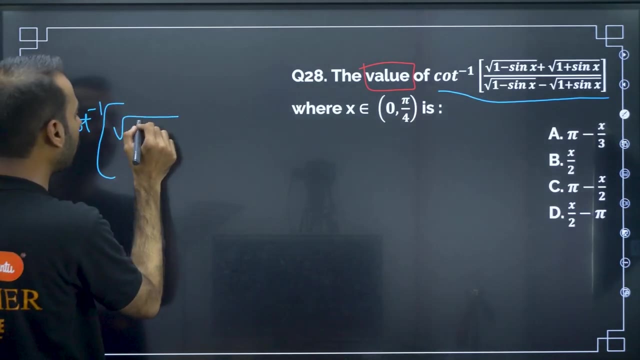 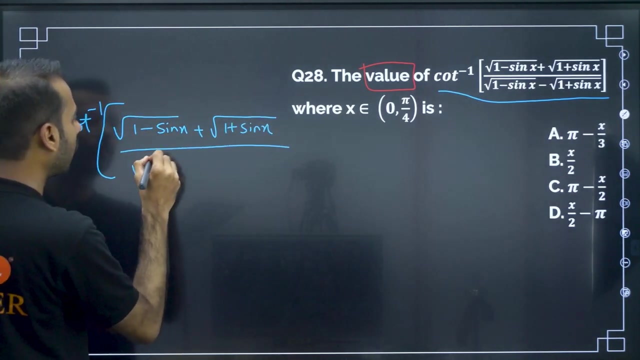 the value of this. they are asking to find a value of this. So what are they asking? the value of this. So how to approach this problem? cot inverse. cot inverse. let me write, let me copy and paste: 1 minus sin x plus 1 plus sin x divided by root of 1 minus sin x minus root of 1 minus. 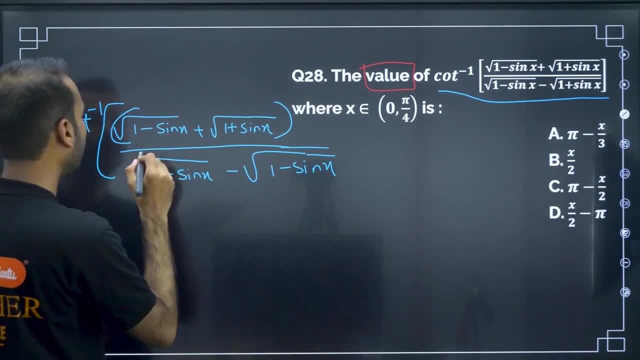 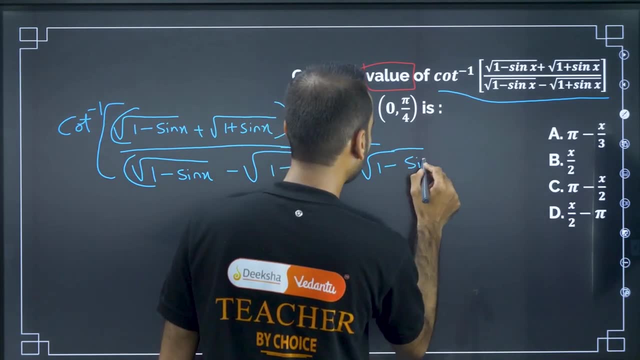 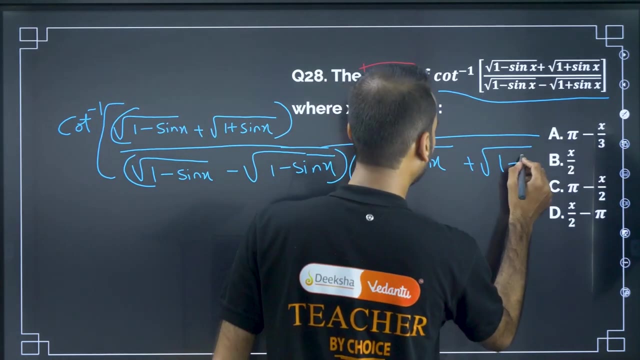 sin x, 1 minus sin x. If I multiply this, if I multiply this with what? 1 minus sin x, sin x, 1 minus sin x, here it is plus root of 1 minus sin x, 1 minus sin x. So here root. 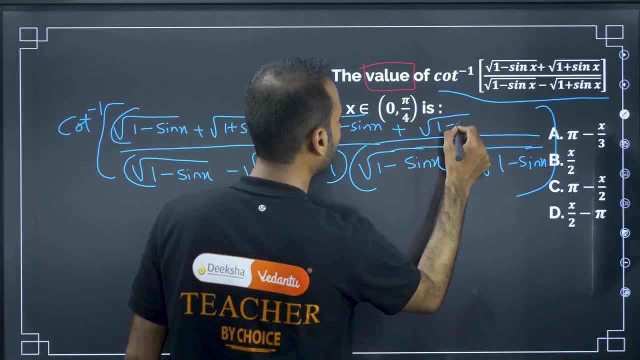 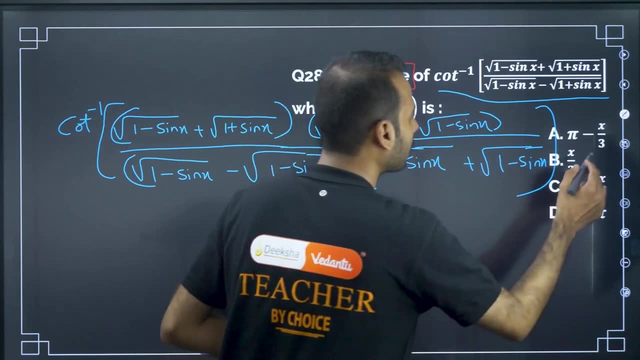 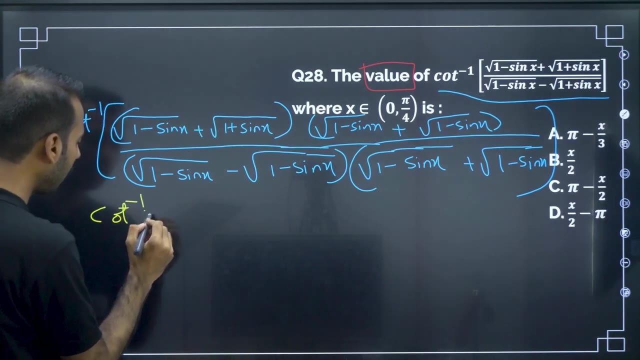 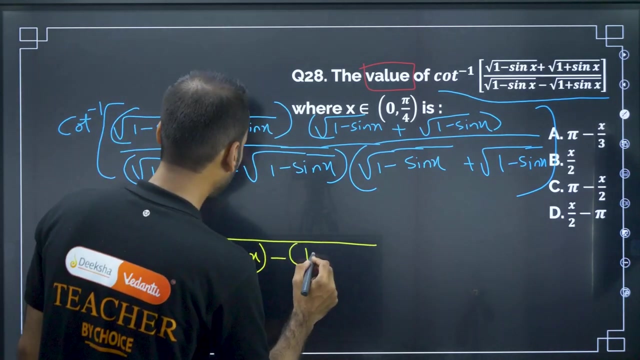 of 1 minus sin x, plus root of 1 minus sin x. So here I am multiplying this numerator and denominator with its conjugate. So the moment I multiply this, this gets simplified to a minus b, a plus b. So a square minus b square means 1 minus sin x minus 1 minus. 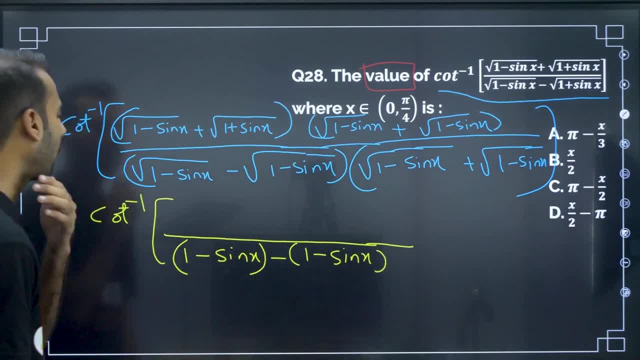 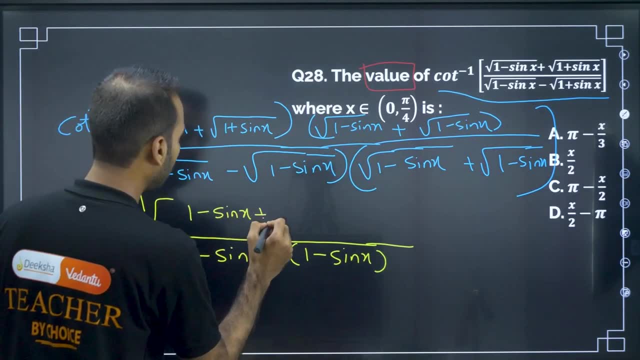 sin x, 2. sin x Next in the numerator. numerator a my a plus b a plus b a square plus b square a square plus b square plus 2 a b, 2 a plus b a square plus b square plus 2 a b, 2 a plus. 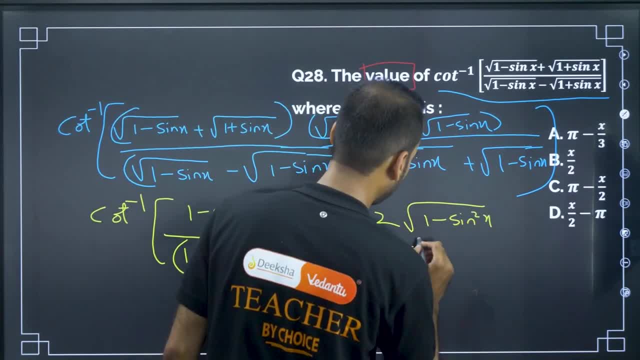 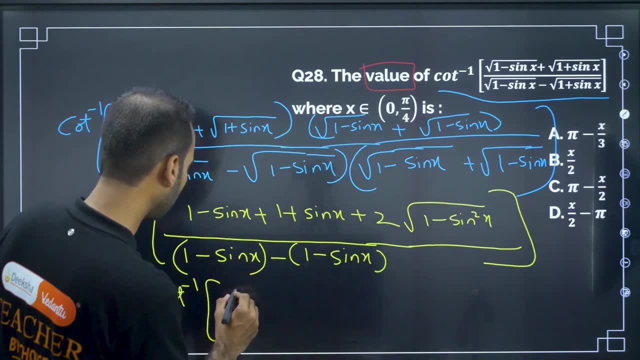 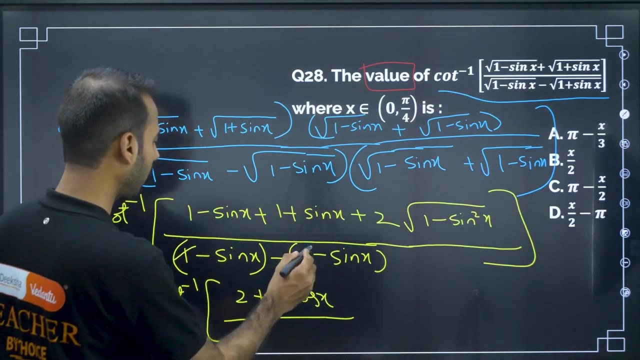 2 a. b is root of 1 minus sin square x, 1 minus sin square x. So this becomes cot inverse, cot inverse. 1 plus 1 is 2 plus 2. this is cos x divided by 1, and 1 will get cancelled minus. 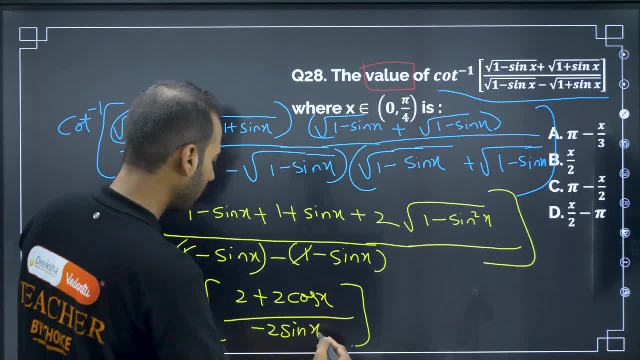 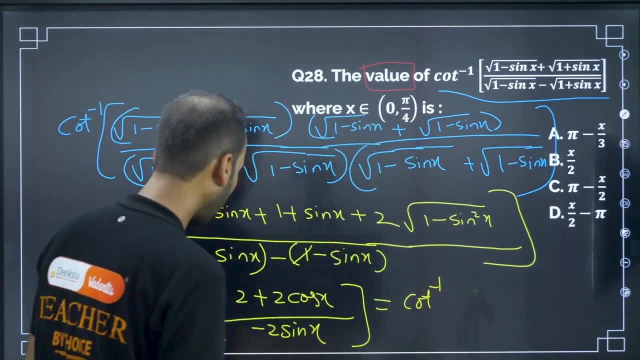 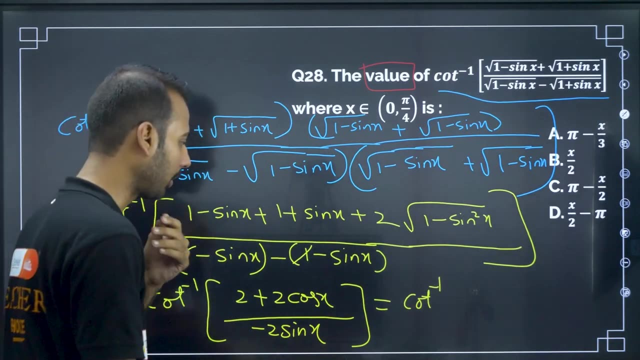 2 sin x minus 2 sin x. So if I take 2 common, if I take 2 common, here we are left with cot inverse of So 2. if I take common, 1 plus cos x, 1 plus cos x is 2 cos square x by 2.. So 2 if I take. 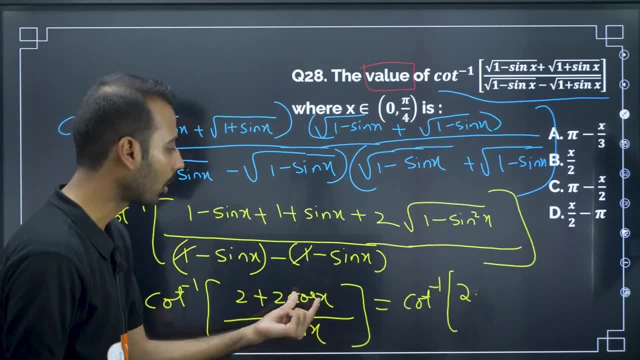 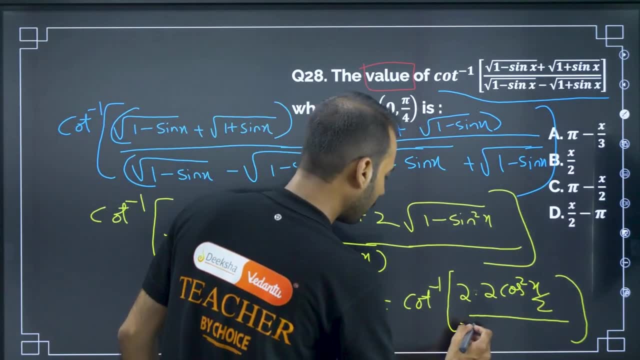 common. if I take 2 common, I am left with 1 plus cos x. 1 plus cos x can be written as 2 cos square x by 2 in the denominator, in the denominator minus 2: 2 sin x by 2 cos x by. 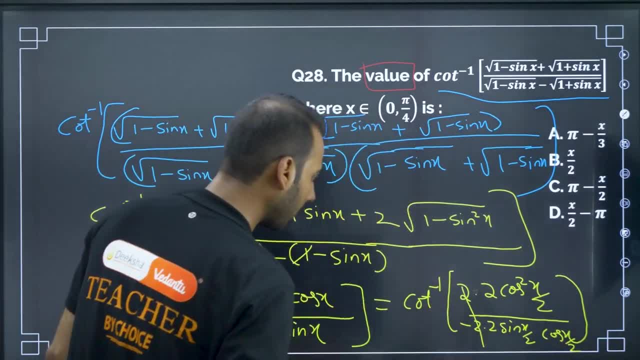 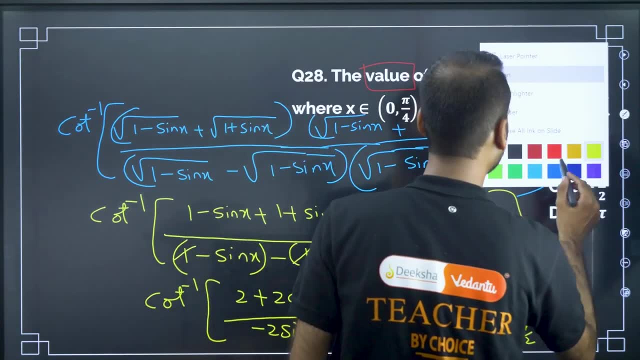 2, 2 and 2 will get cancelled. So oops, sorry, 2 will get cancelled, So 2 will get cancelled. Here i take 2, so this 2 will get cancelled. cos x by 2 and cos x by 2, so coach inverse. 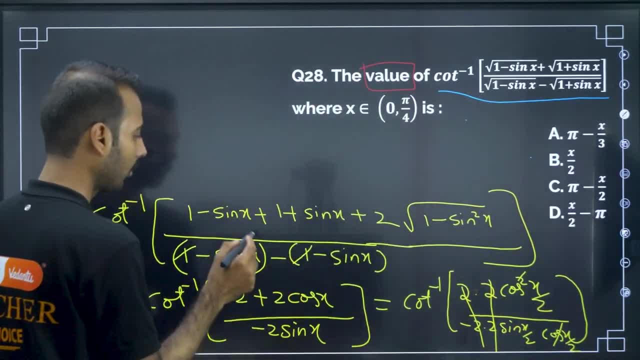 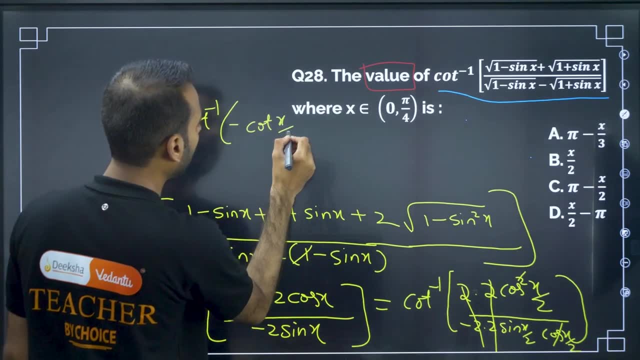 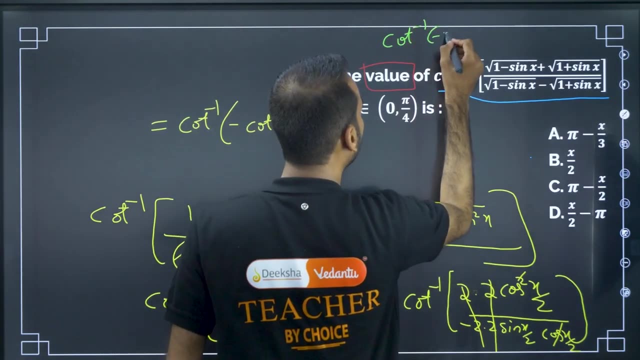 eraser if I remove all this. So here we are left with cot inverse of cot inverse of negative cot x by 2 negative cot. So one synopsis point you should be knowing at this point of time: cot inverse of minus x is pi minus cot inverse x. 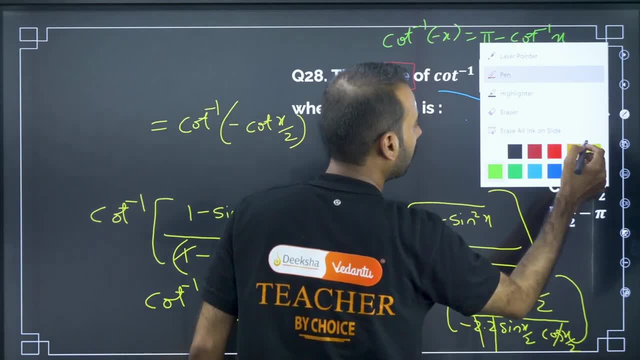 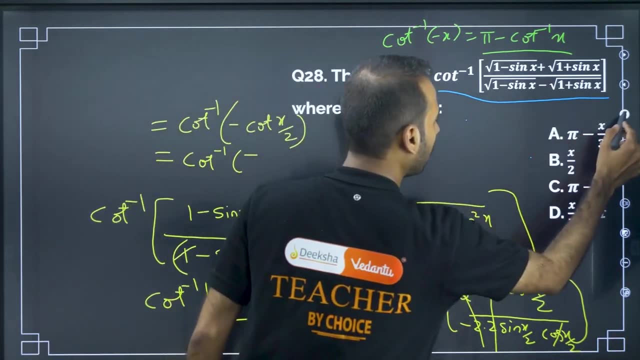 So for this, the first and last function is smallickt. Jess B empez unskeptろうaż. we don't have much force, so we just need to remove this one. So checked, investing also for this. cot inverse of cot inverse of minus x can be written as: 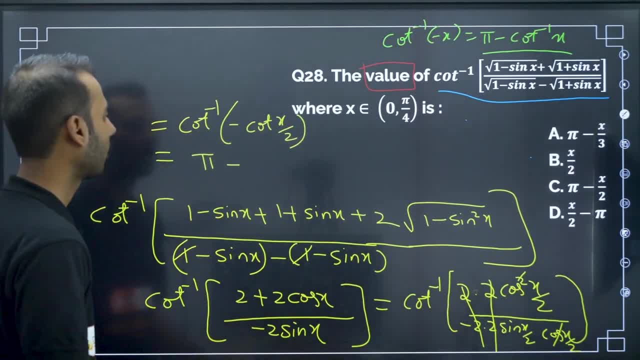 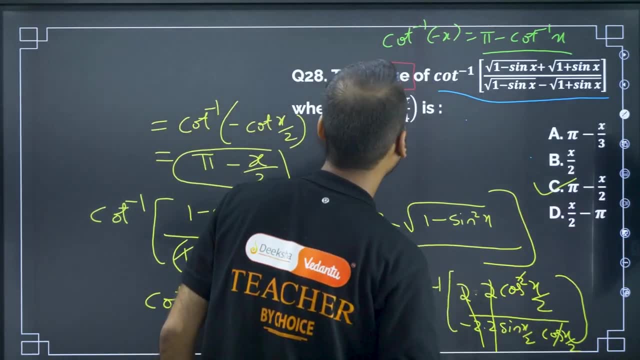 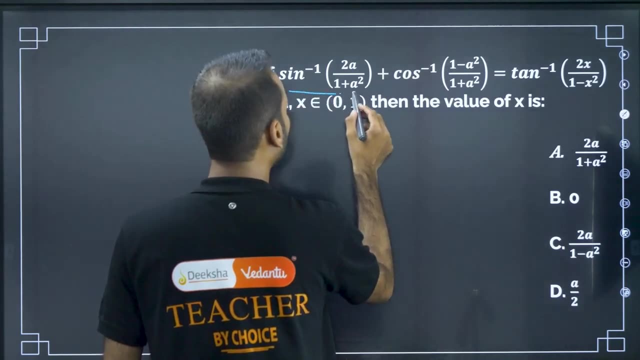 pi minus cot, inverse of cot, inverse of pi minus x by 2.. So is there any option like pi minus x by 2? Yes, C is the answer. Moving on to next question: sin inverse. some question. they have given some expression. they have given this expression. they have given. 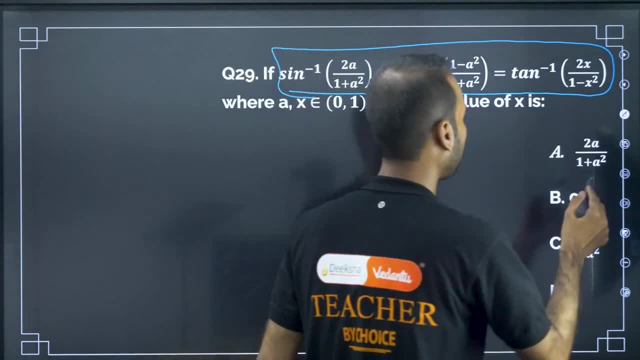 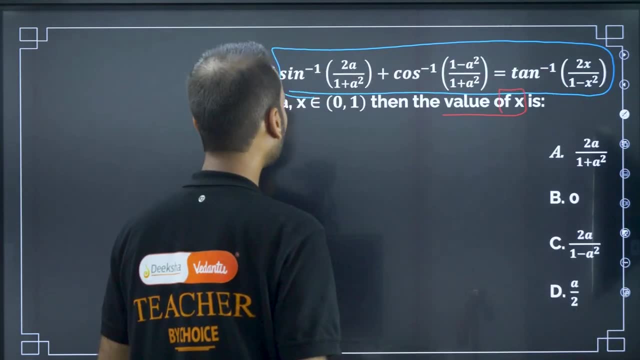 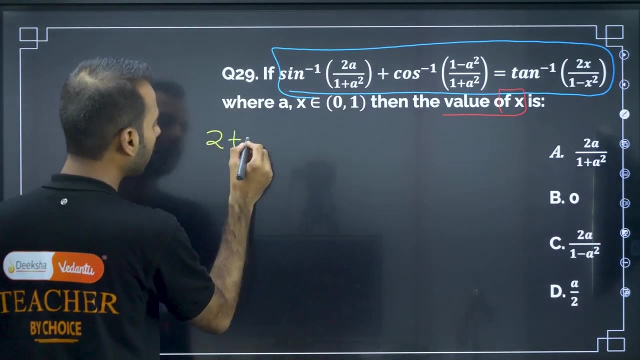 sin inverse of, then value of x is what are they asking? They are asking to find value of x. is So how to approach this problem? Some synopsis point. you should be knowing what are those synopsis point. So sin inverse 2a can be written as 2 tan inverse a, 2 tan inverse a. 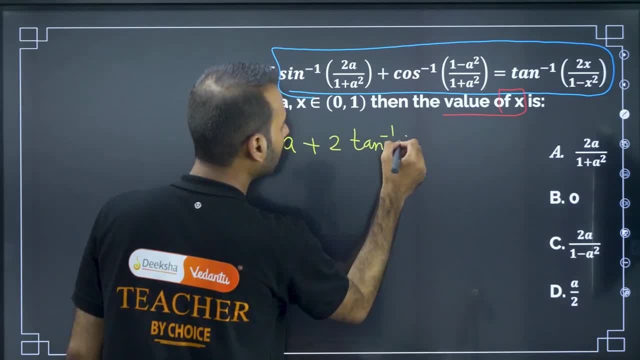 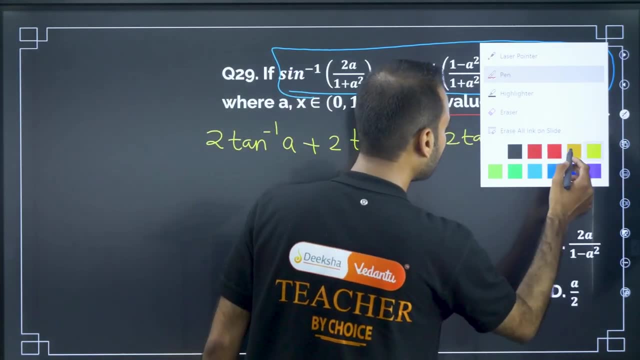 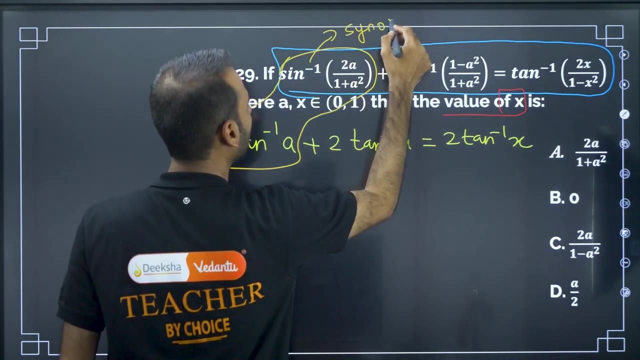 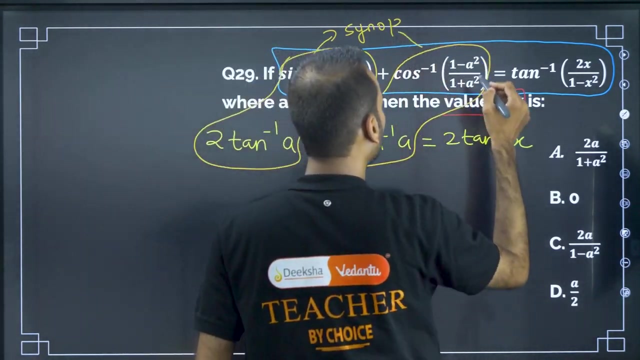 plus 2 tan inverse a. 2 tan is equal to 2 tan inverse a, sin inverse of sin, inverse of sin. inverse of sin 2 tan inverse x. See here: this sin inverse of this is this: you take this as synopsis point. you take Cos inverse of y minus a. again, this is also synopsis point, again synopsis. 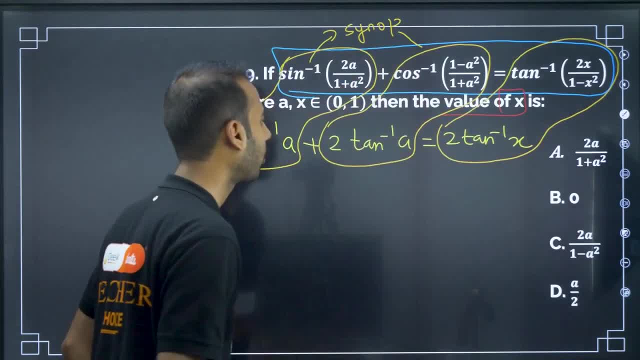 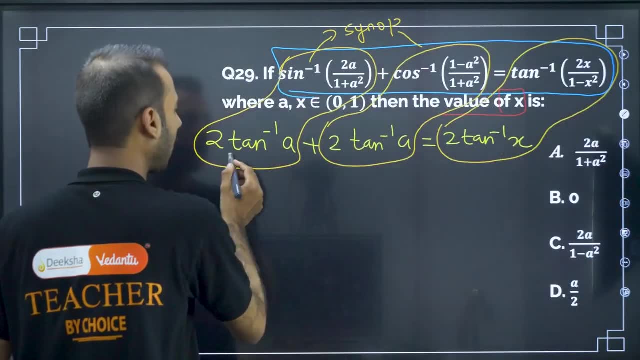 point: 2 tan inverse x. again, this also synopsis point. So if you know the synopsis of inverse trigonometry, see here. the things are very simple. What we have to do now- 2 tan inverse a, 2 tan inverse a is 4 tan inverse a, 4 tan inverse. 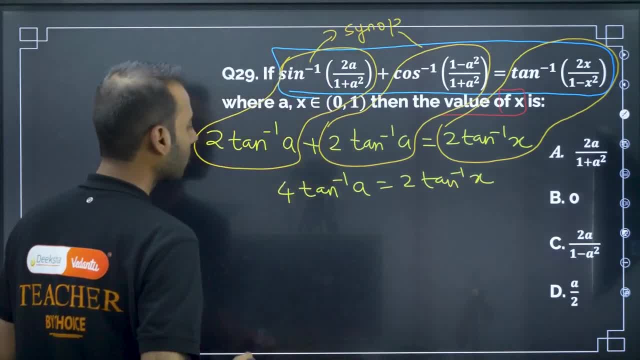 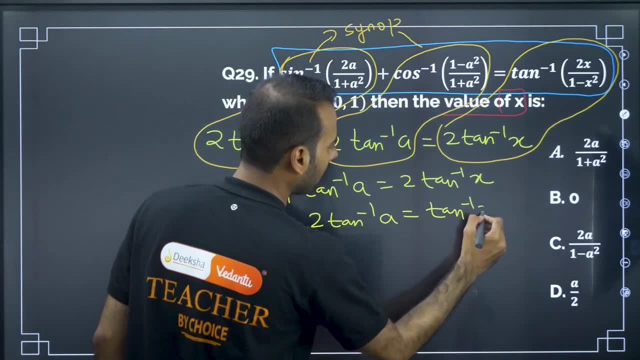 a is equal to 2 tan inverse 2 tan inverse x. So 4 tan inverse a is 2 tan inverse a. 2 tan inverse a is equal to tan inverse x. Next, 2 tan inverse a can be written as tan. 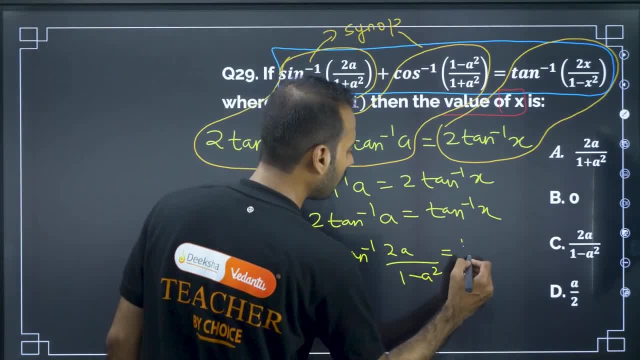 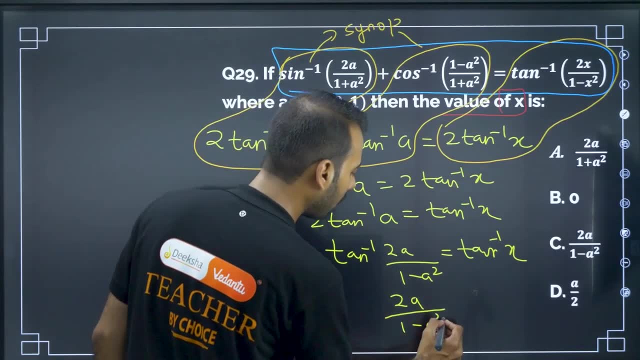 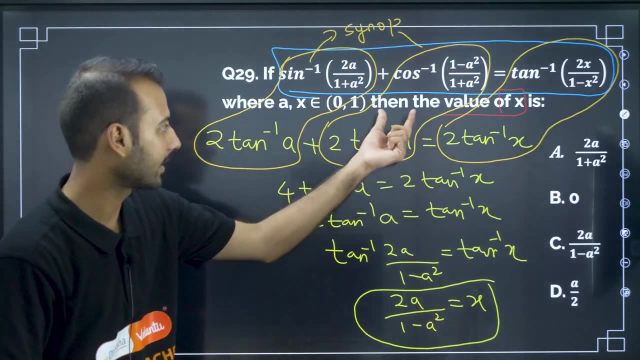 inverse 2 a by 1 minus a square is equal to tan inverse x. Next, 2 a divided by 1 minus a square is equal to x. So x is equal to 2 a by 1 minus a square. What are they asking? They are asking. 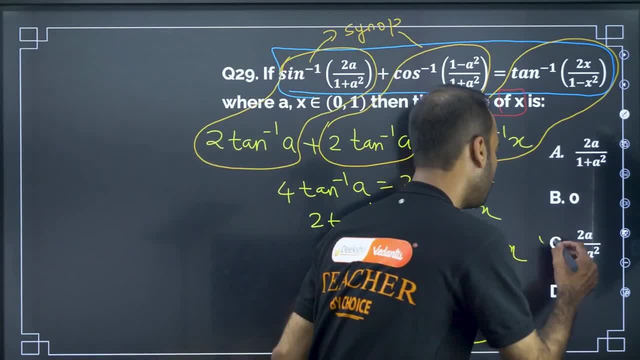 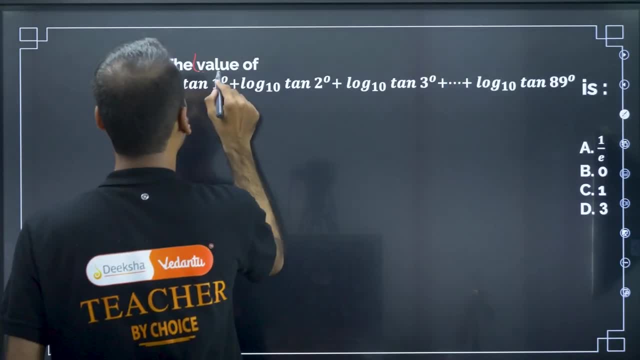 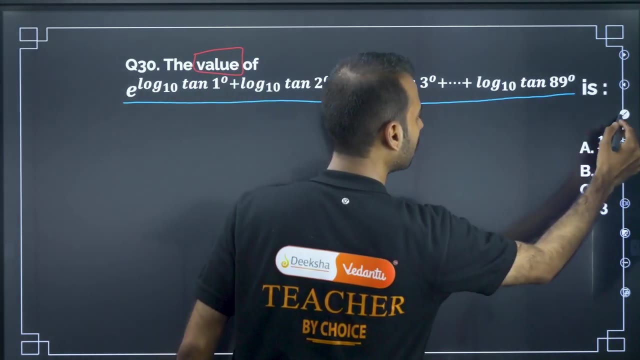 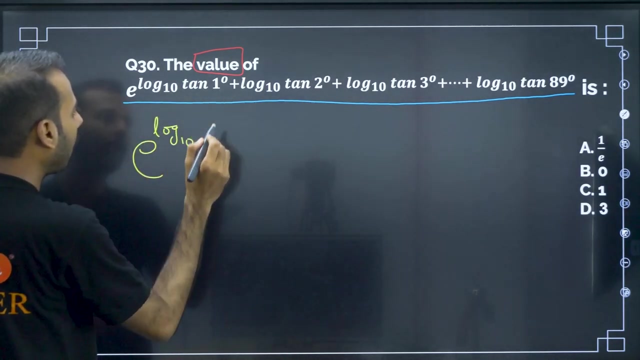 to find value of x. x value is 2 a by 1 minus a square. So c is the answer. Moving on to next question, The value of one expression. they have given they are asking value of one expression. What is that expression? e log, all this is So let me write e as it is, log to the base: 10 tan. 1. 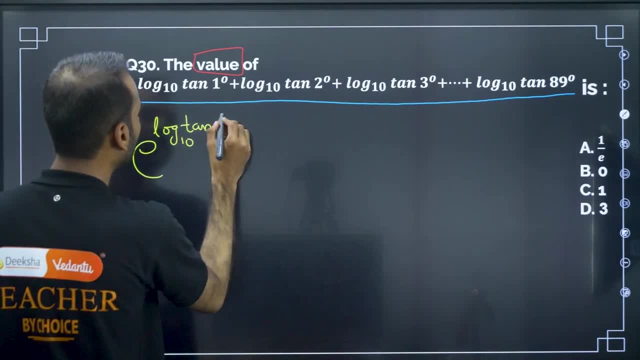 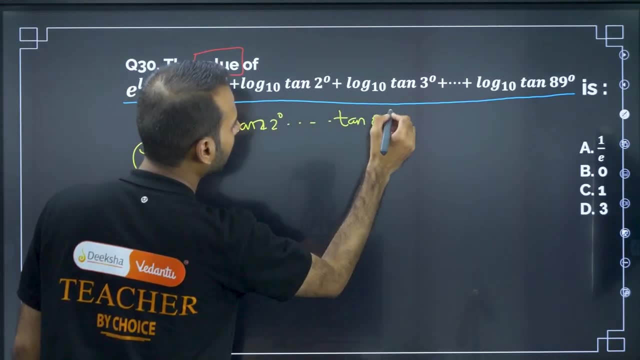 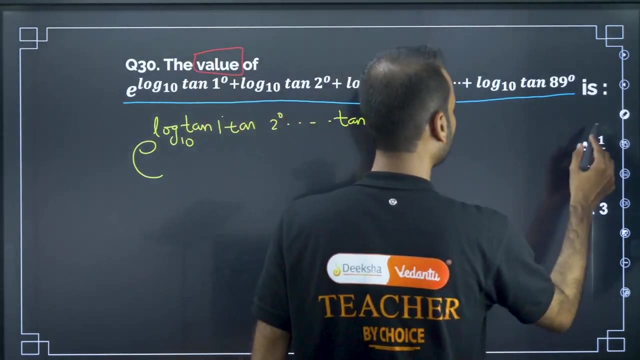 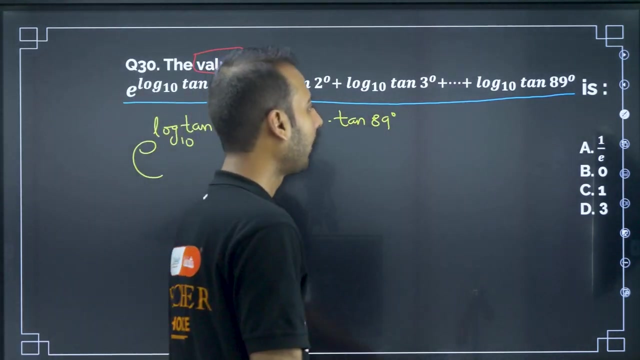 tan 2.. So tan 1, tan 2, tan 2, blah, blah, blah up to tan 89.. Tan 1, tan 2, tan 89.. Let me use tan 1, tan 2, tan 89.. Now e log tan 1.. See, here I am using properties of logarithm.